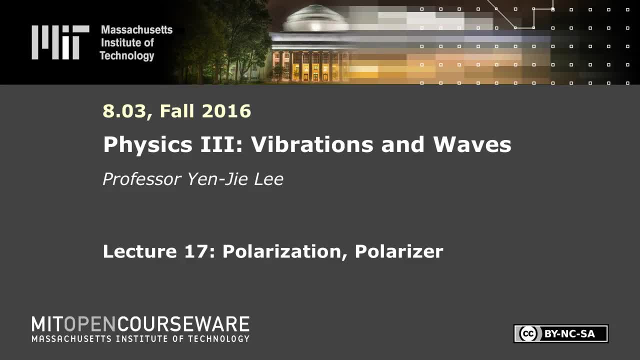 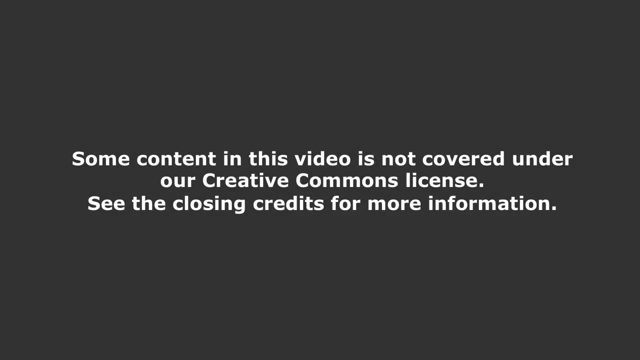 The following content is provided under a Creative Commons license. Your support will help MIT OpenCourseWare continue to offer high quality educational resources for free. To make a donation or to view additional materials from hundreds of MIT courses, visit MIT OpenCourseWare at ocwmitedu. 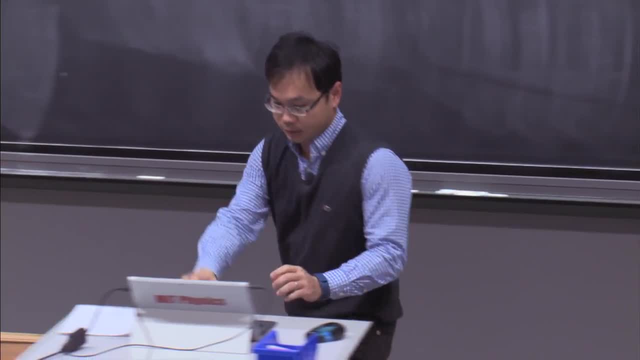 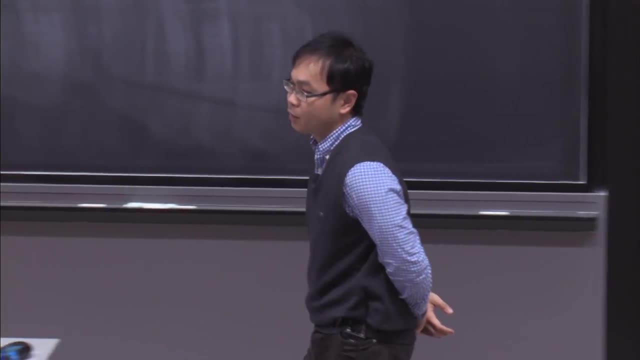 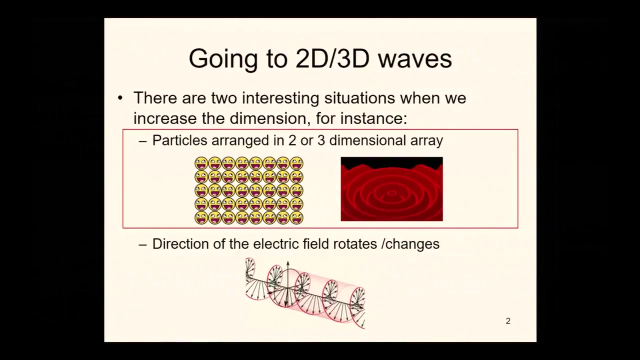 All right, so let's get started. So today- very happy to have you here- We are going to continue our discussion on the two-dimensional and three-dimensional waves. So, as I mentioned before, there are two interesting situations in which we can actually increase the dimension. 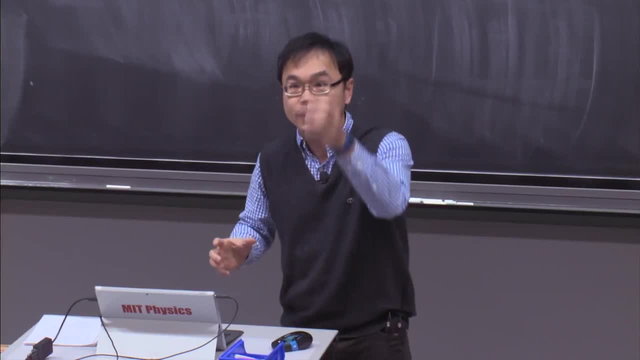 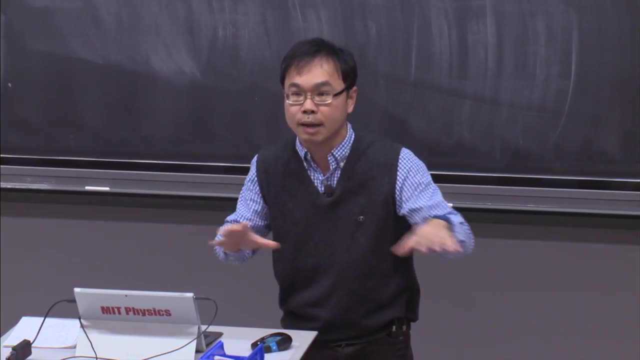 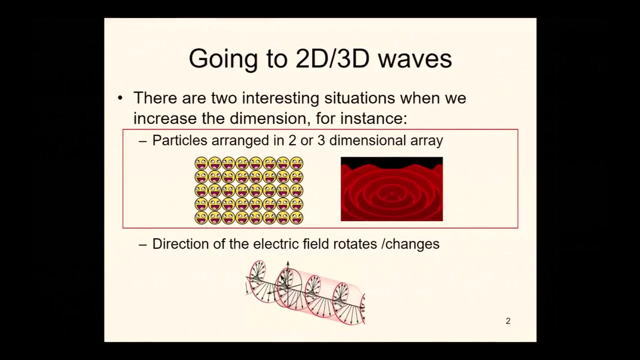 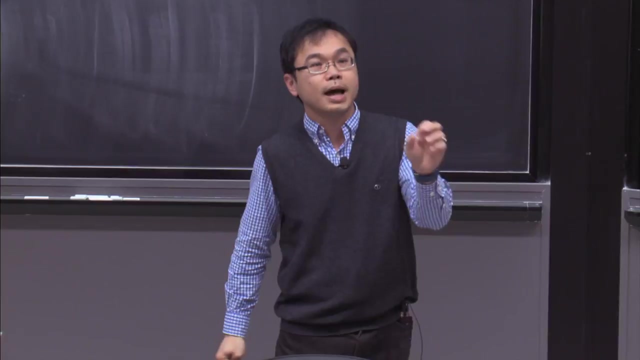 So, for example, I can have all the objects oscillating in just one dimension or one direction, but I change the way I place the objects in the space. For example, I can have particles which are arranged in two or three dimensional arrays, And we were talking about how to understand this kind of system. 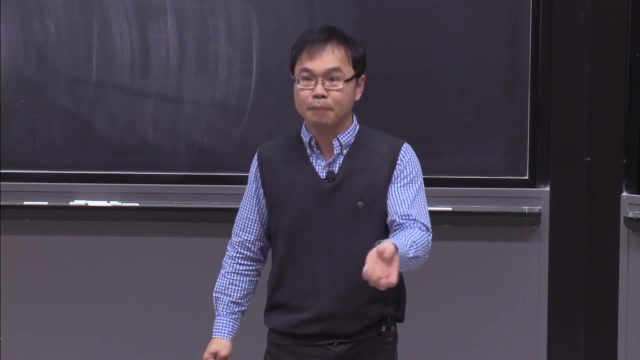 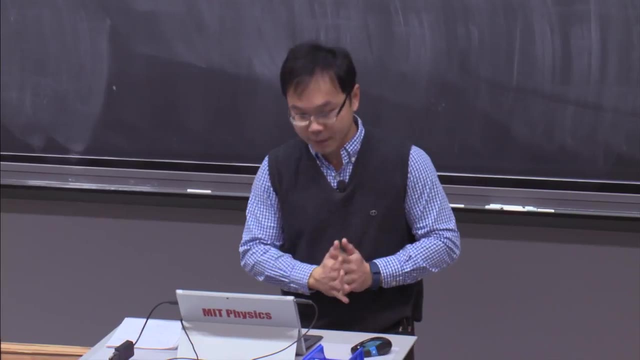 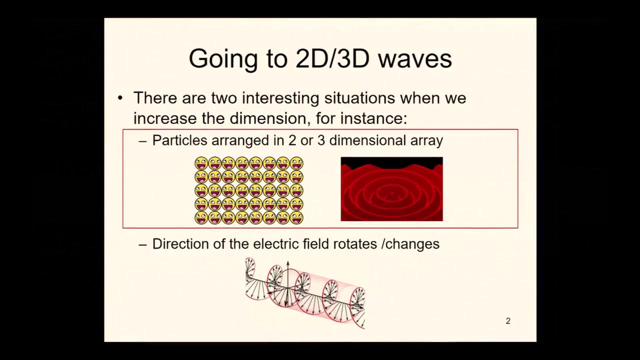 And all those objects are oscillating in just one direction, for example, up and down, in one direction. That's actually one method we can increase the dimension. There's another interesting example which we will talk about today, which is to change the direction of the oscillation. 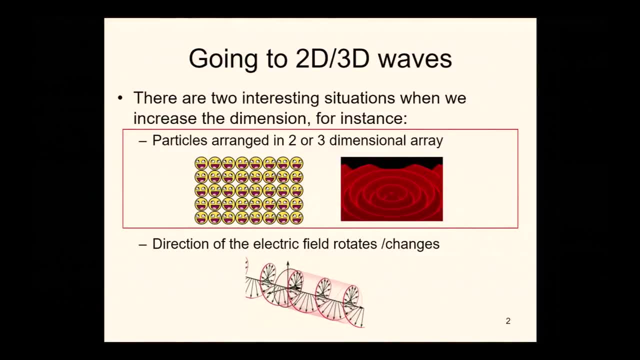 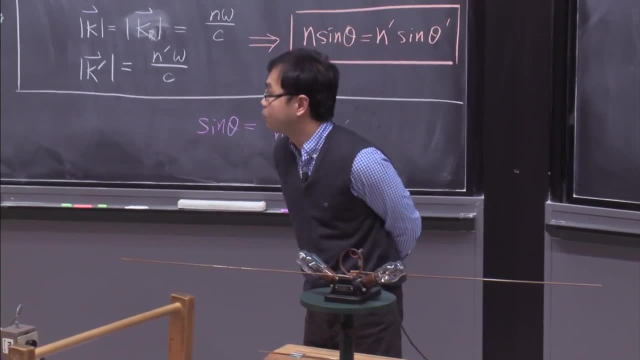 even rotate, the electromagnetic waves, for example- And how can we achieve that And how do we understand this kind of phenomena? That's actually going to be covered by the lecture today. So before we move forward, we will have a short review on what we have learned from last lecture. 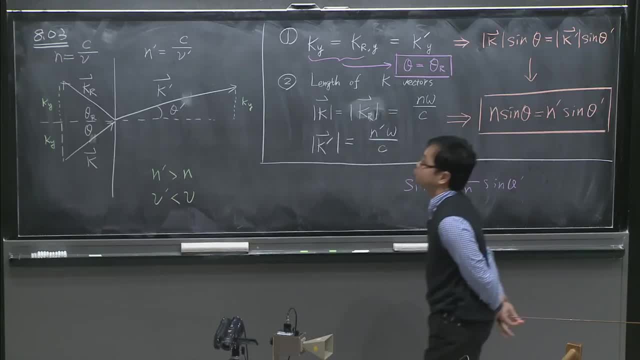 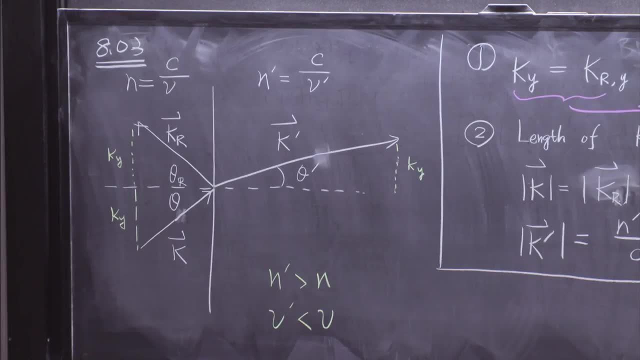 This is actually what we discussed. If I have two materials- the left-hand side and the right-hand side are two different kinds of materials or very same membranes- And if I have an incident wave coming into the boundary of these two materials, which is x equal to 0,, as we discussed last time. 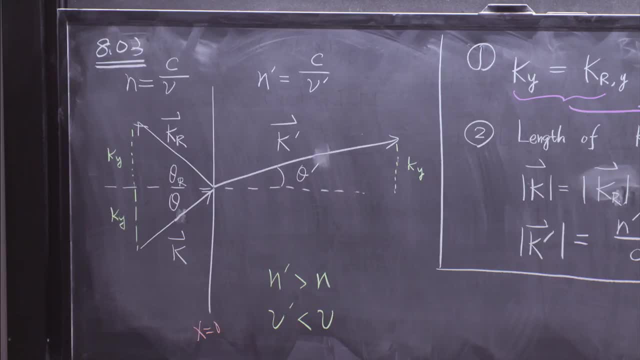 basically, the boundary condition requires that, in order to make sure that the membranes didn't break- That means the k vector- the projection in the y direction of the k vectors has to be the same. That means the projection of the wave in the y direction, which is along this line: 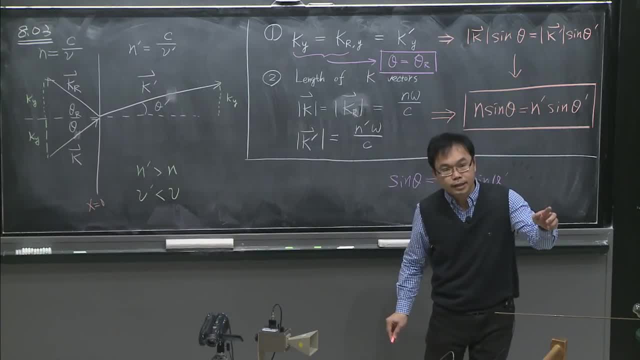 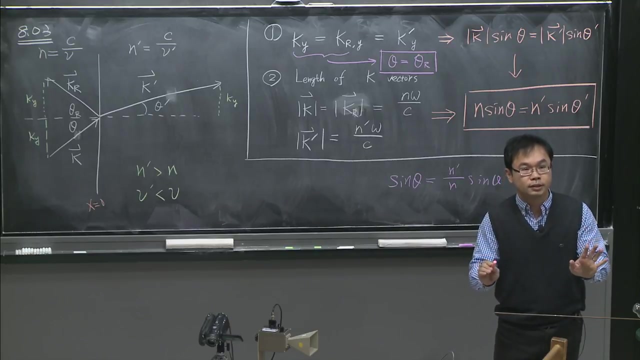 should be the wavelength of all the incident refracted and transmitted wave. The wavelength should be all the same, Otherwise I can change the y and make the membranes break or break the boundary condition. So that's actually the first thing which we learned from the math we were doing last time. 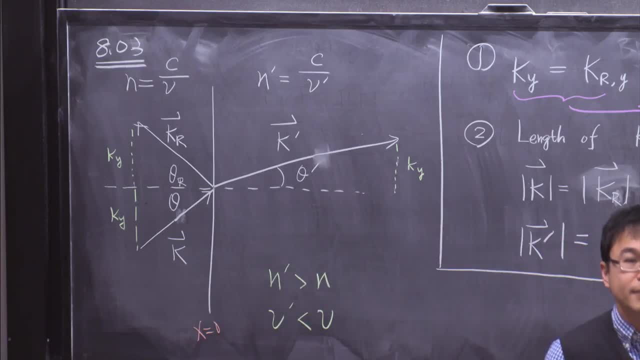 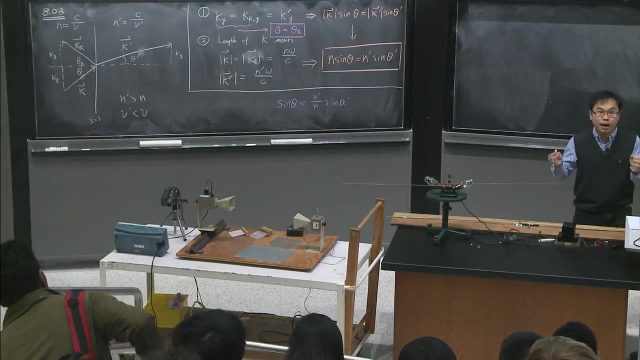 And also the k values are not arbitrary, So we were already assuming that. So all the three waves, all the three plane waves, are oscillating at the same frequency. If they are oscillating at different frequency it doesn't work. 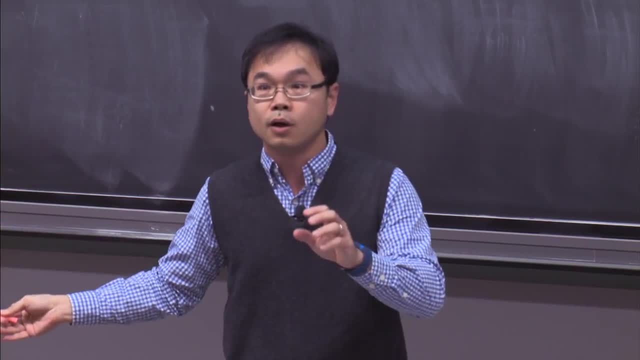 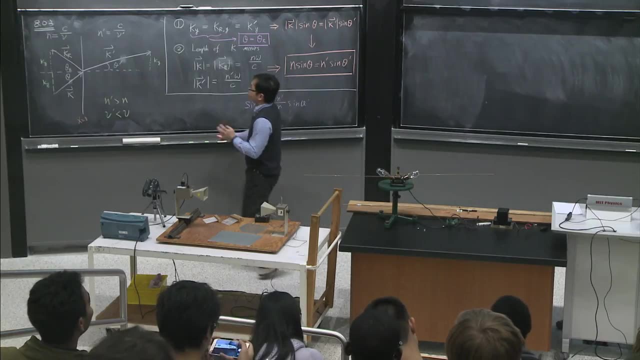 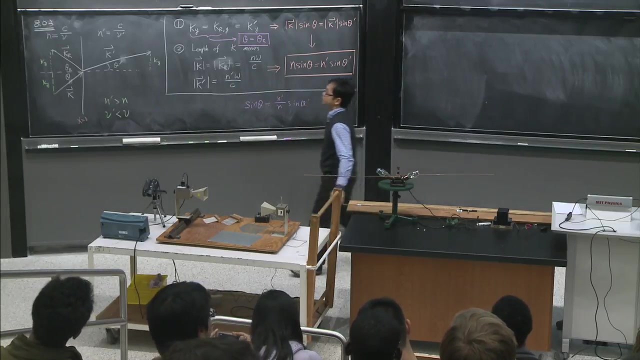 Because I can change time, then make the membranes break. So therefore, all the three plane waves will be oscillating at the same frequency, omega, And according to this formula. so we have defined n, which is actually the refraction index. 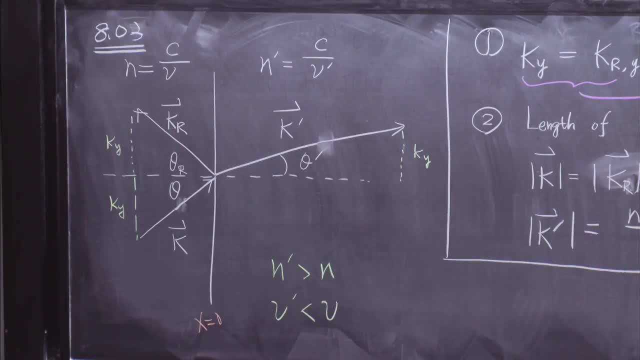 which is actually equal to some constant, c, divided by the speed of the propagation, the phase velocity of the left-hand side material. And we also can define n prime, which is actually equal to c, the same constant, divided by v prime. 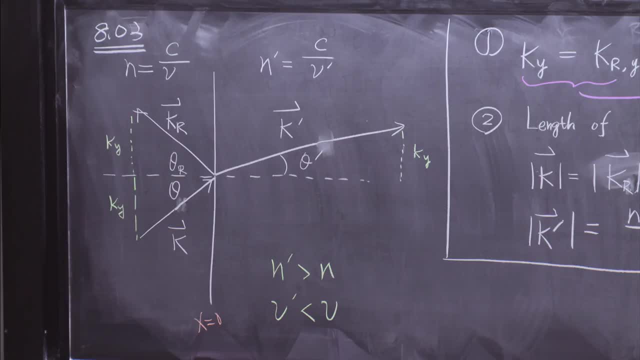 which is the speed of propagation of the right-hand side material, And according to the dispersion relation we can calculate what will be the length if omega is given. The omega for the left-hand side and right-hand side, refracted, transmitted and in certain waves, should be the same. 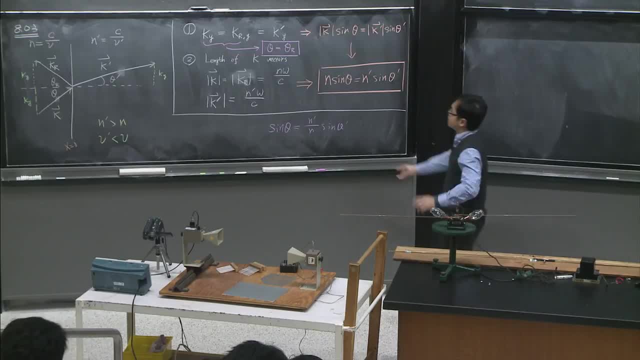 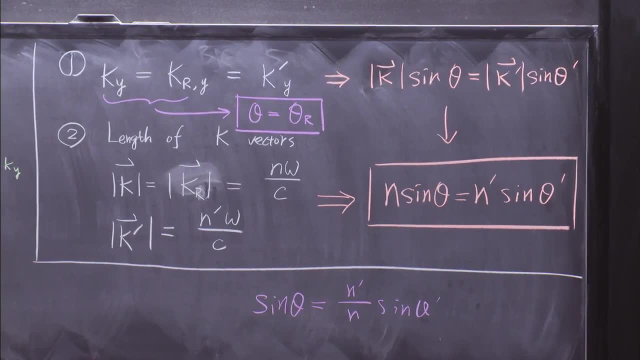 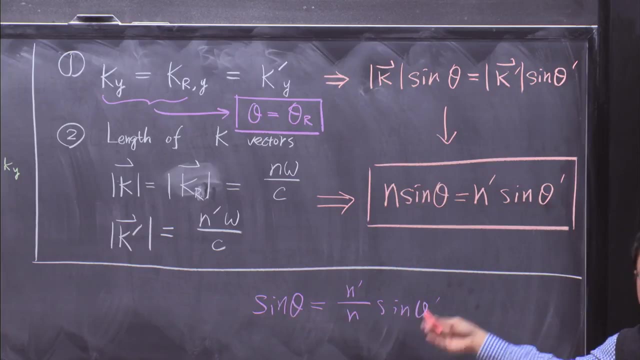 Therefore I can immediately write down what will be the length of the k vector, And that means the length of the k vector will be equal to n times omega over c. So c over n is actually just v. So basically it's just the non-dispersive median. 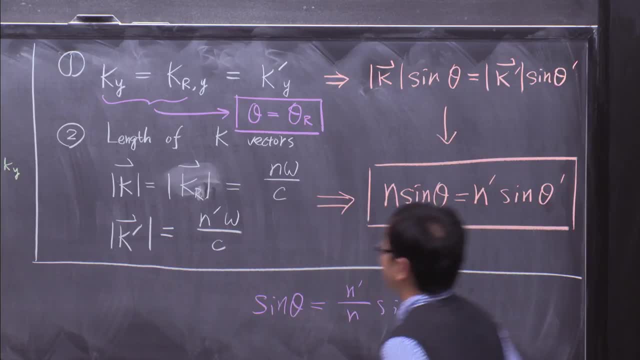 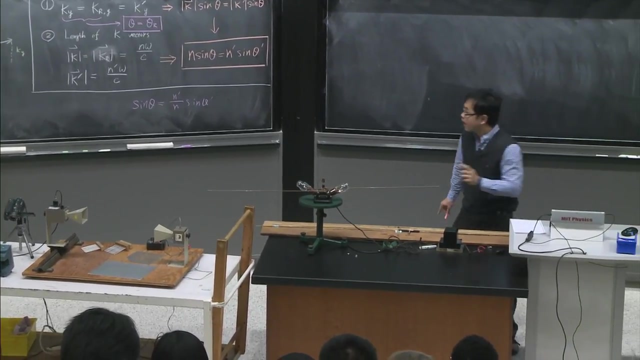 which is the dispersion relation. And also you can go ahead and write down what will be the length of the k prime, And that is actually determined by n prime, omega over c. So, based on these two interesting information, what we can conclude is that huh. 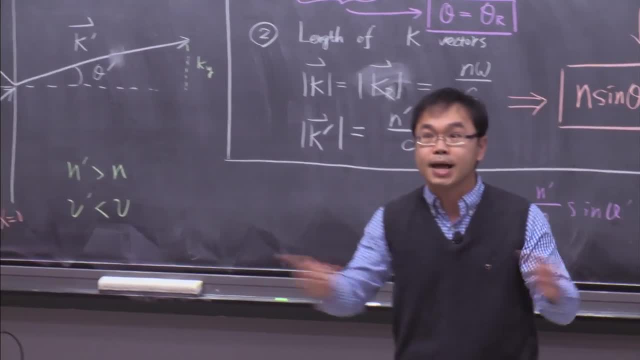 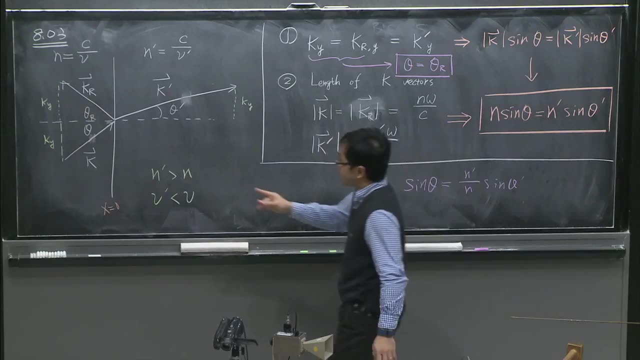 that means k prime and the kr cannot be arbitrary. They have to be aligned to form a specific pattern. So the projection in the y direction should be the same And also at the same time. the length of the k vector is determined by the refraction index. 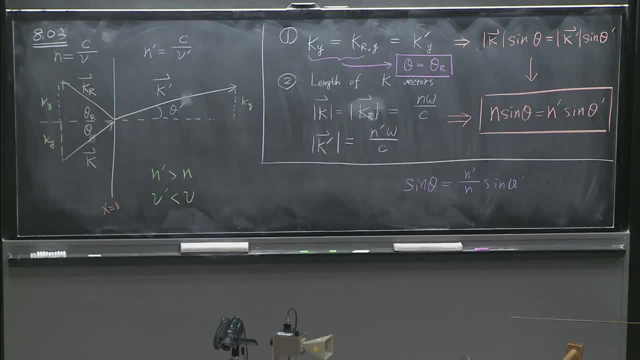 So once we fix all that and put them all together, we can conclude that, based on the projection in the y direction, we will conclude that theta will be equal to theta r, where theta is actually the incident angle and theta r is the refraction angle. 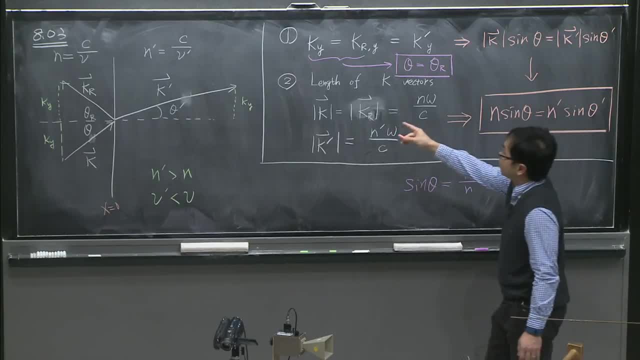 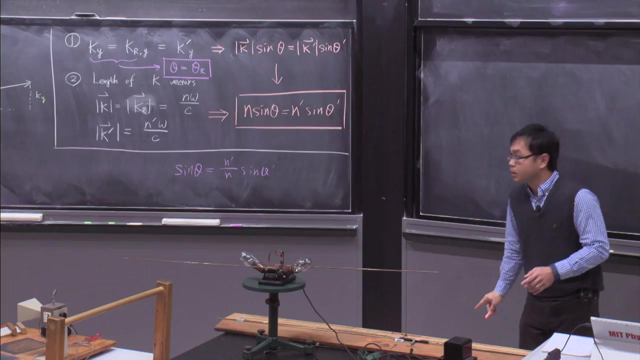 which is describing the direction of the refractive wave, And also the second very interesting information we learned is that, based on the boundary condition, we can conclude that n sine theta will be equal to n prime, sine theta prime. So that's actually the Snell's law. 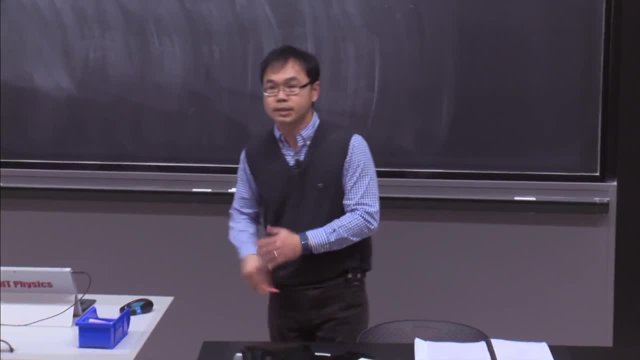 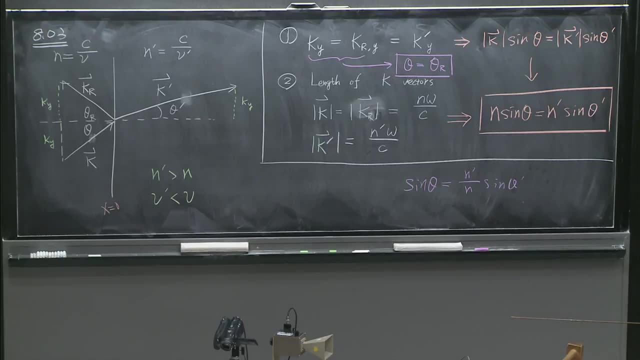 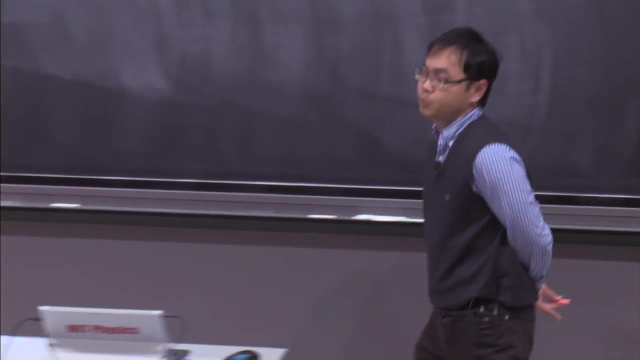 which some of you actually learned from the high school days or from earlier lectures in physics, And these two interesting results forms the basis of geometrical optics laws. That's two of the most important laws we learned from geometrical optics. So that's actually give you some example. 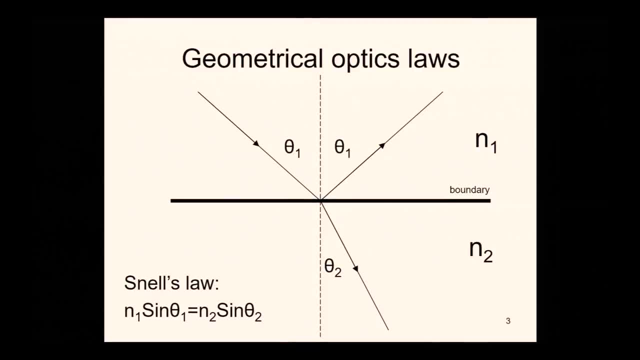 and give you some more feeling about what are we talking about. So what we are talking about is that we have an incident wave coming into this boundary and the incident angle is theta 1. What I would expect based on what we have just derived. 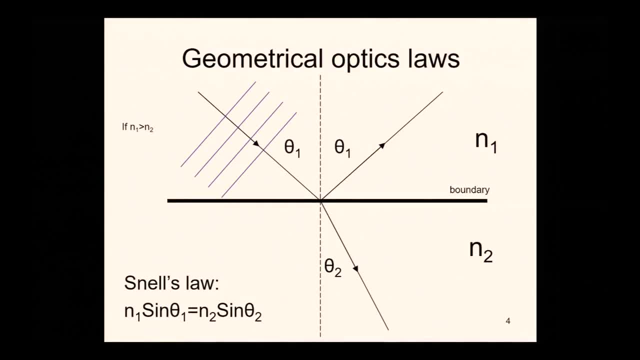 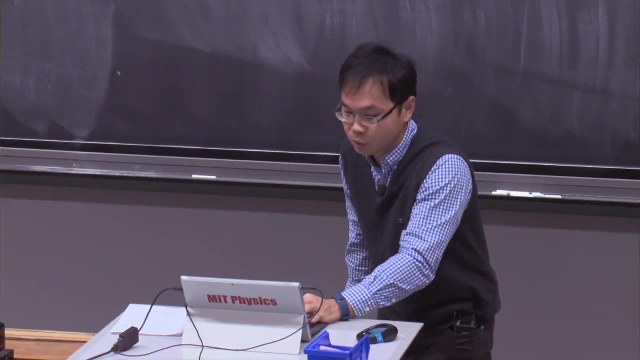 is that the theta r, the refractive wave direction, the refractive wave angle, the refraction angle, would be equal to the incident angle which we have just derived. I was just rotating this by 90 degrees And also we can calculate what would. 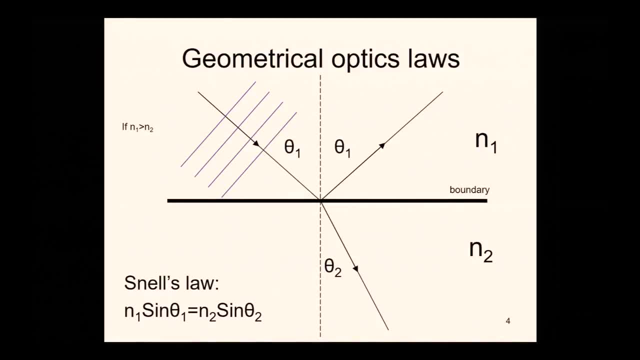 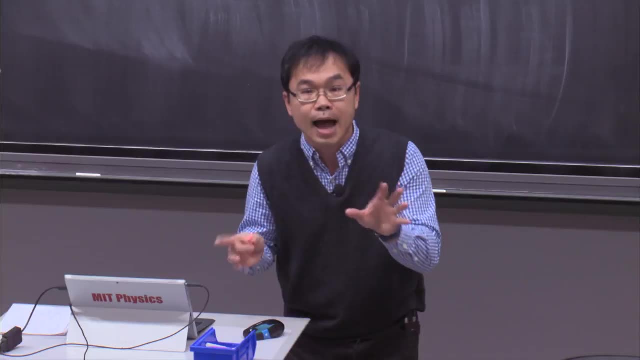 be the theta 2. according to Snell's law, n1 sine theta 1 equal to n2 sine theta 2.. And if I continue and propagate the incident wave here, I assume that n2 is larger If you have a larger refraction index. 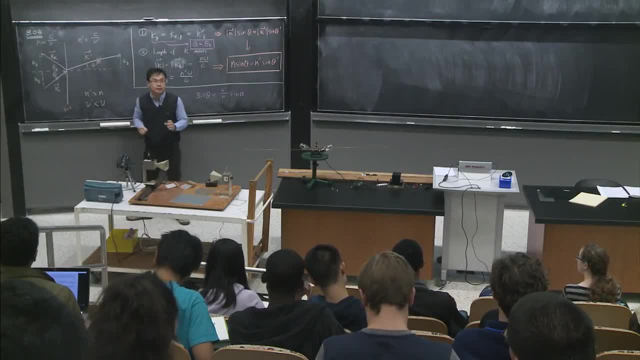 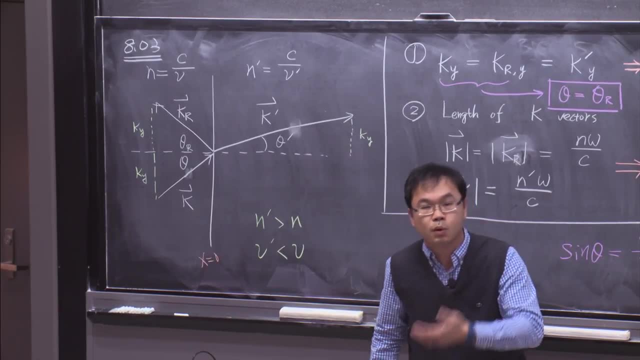 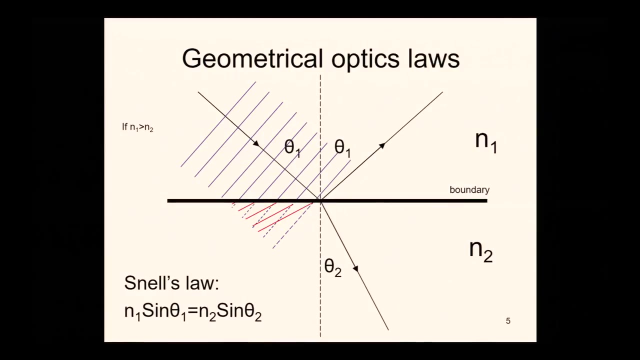 that means the speed of propagation is smaller. Larger n value give you a smaller speed of propagation. Therefore, you can see that the wave front, which is actually the peak value, the position of the peak, actually got delayed compared to the original projection. 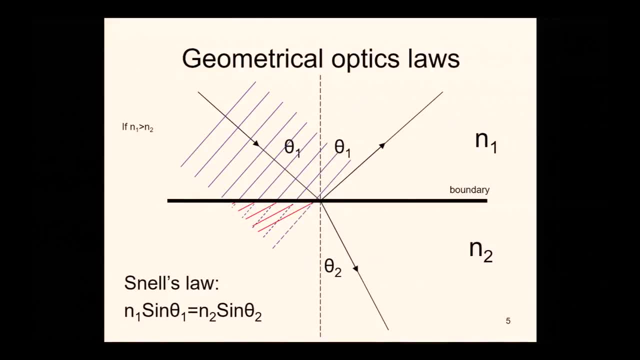 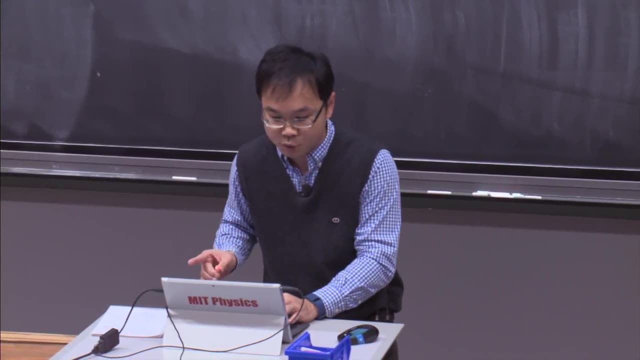 And you can see that the red line is what you would see in the second median. And then we can also continue to propagate And you will see that, huh interesting. That means the plane wave would change direction because of the matching boundary condition. 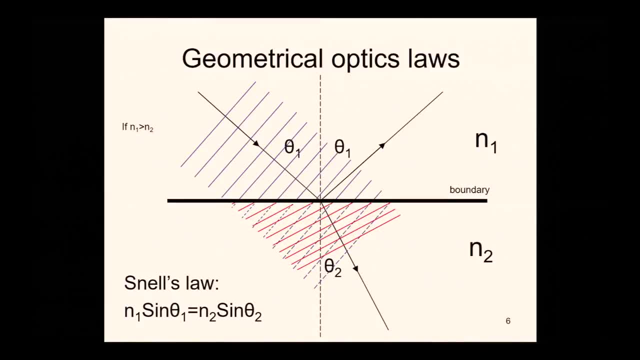 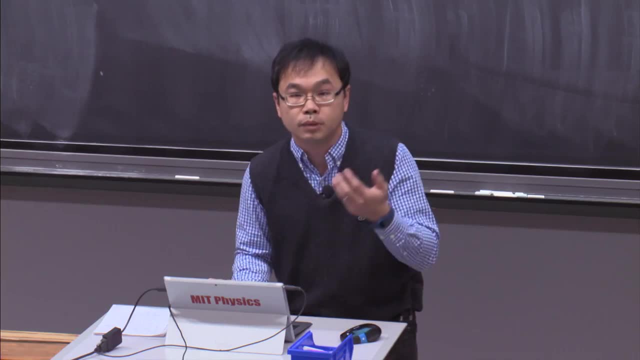 The membranes didn't break. You can see that the peak position match from the median number 1 and median number 2.. So the position which is the position of the line match And also due to the slower speed of propagation. 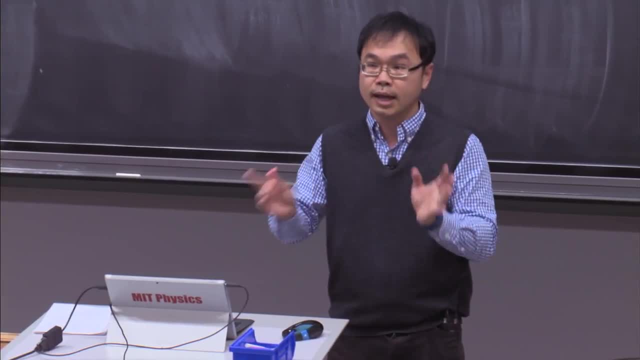 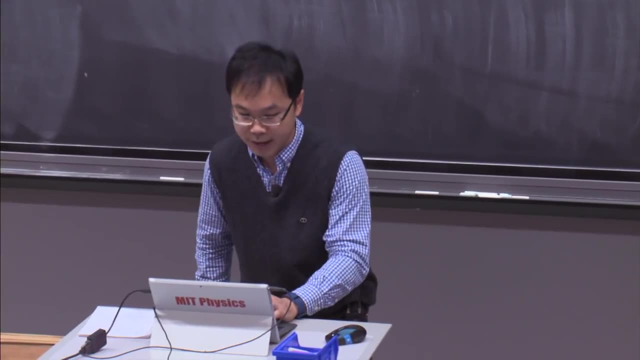 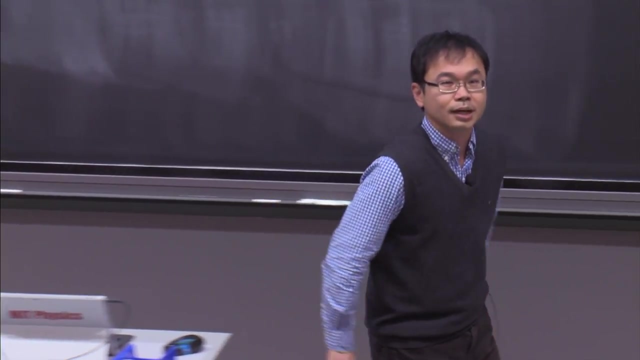 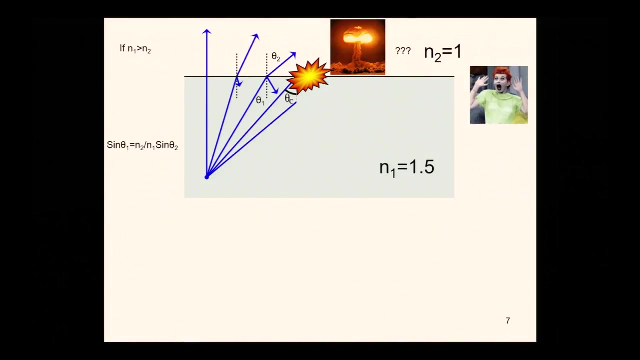 the plane wave actually changed direction. So that's actually how we actually can understand the mathematical result which we derived last time by this interesting example. So let's actually consider a situation which may be interesting to you. So what will happen if I now shoot light? 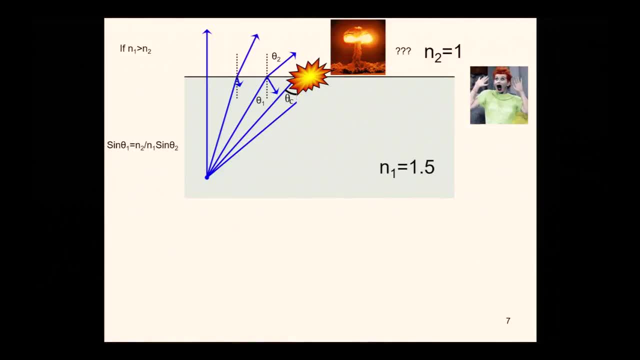 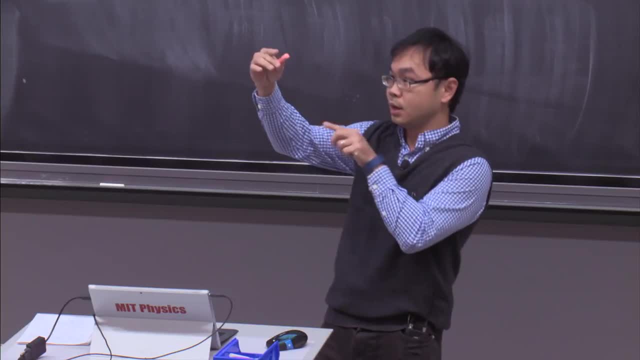 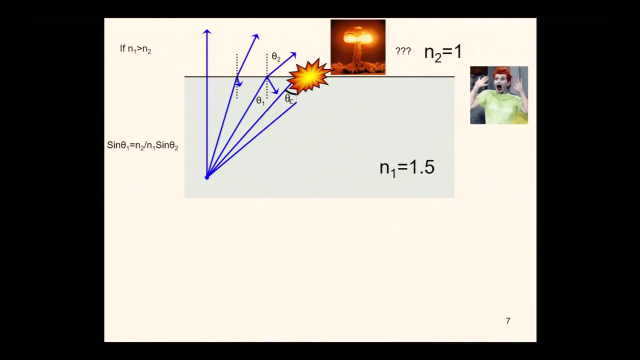 from inside some material which delay the light slightly. For example, n1 is equal to 1.5.. OK, I shoot something through the material. Then in the second material I have higher speed of light, which is actually having the speed of light. 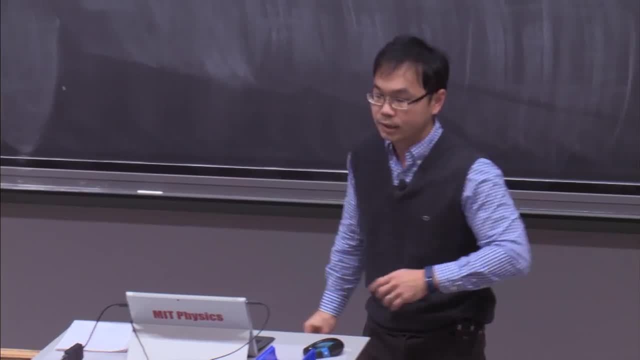 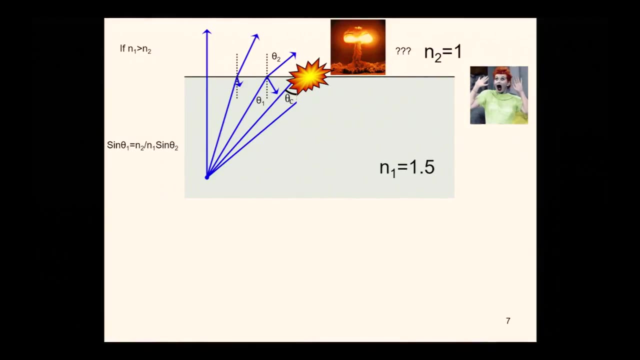 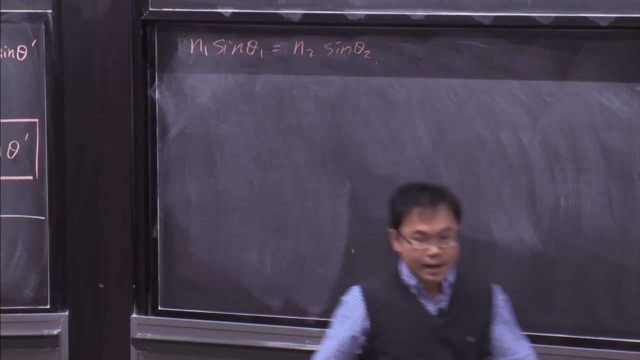 at the vacuum in the vacuum case. So in this example I have n1 greater than n2.. Since n1 sine theta 1 is equal to n2 sine theta 2, so now I can calculate what will be the resulting theta 2. 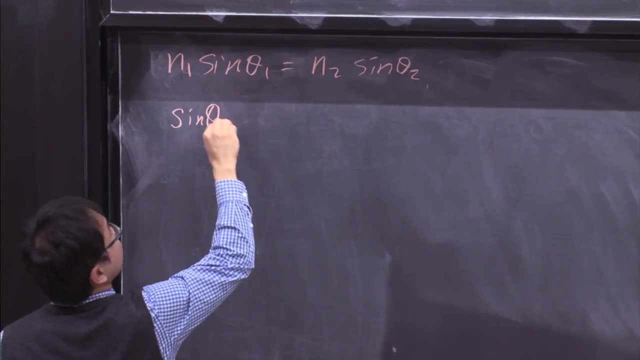 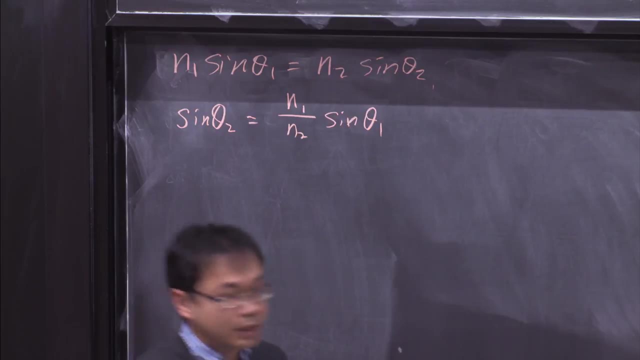 according to this equation, So the resulting theta 2 will be sine theta 2 will be equal to n1 over n2, sine theta 2.. OK, In this case n1 is greater than n2.. Therefore, this term is greater than 1.. 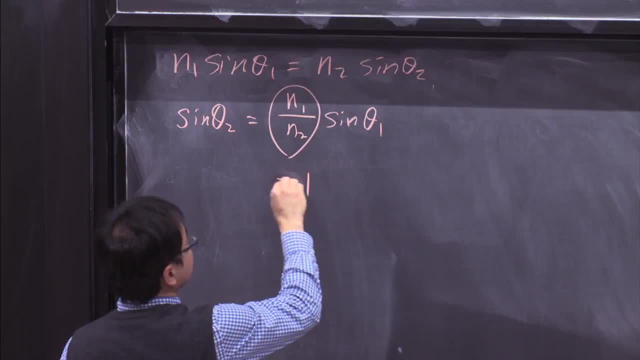 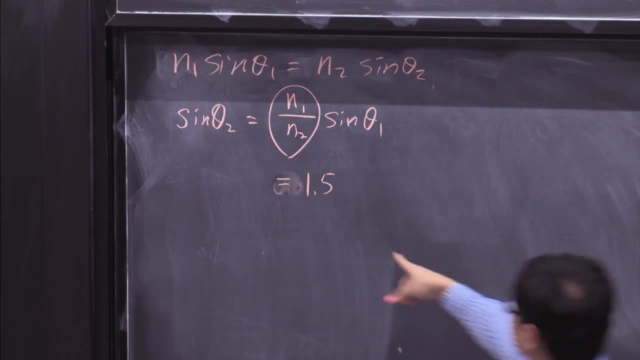 Right, And in this case, actually, this ratio is equal to 1.5.. OK, So this is actually pretty interesting. That means, OK, this factor is actually greater than 1.. I have sine theta 1, which is multiplied in this factor. 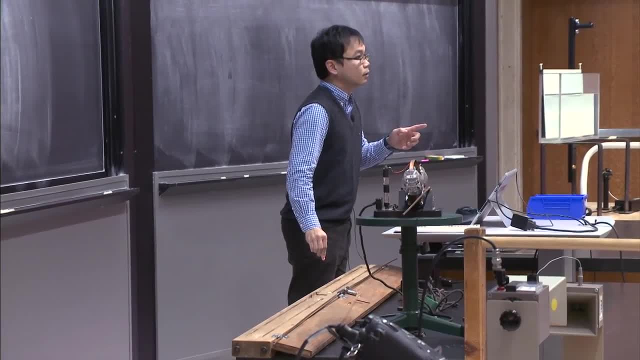 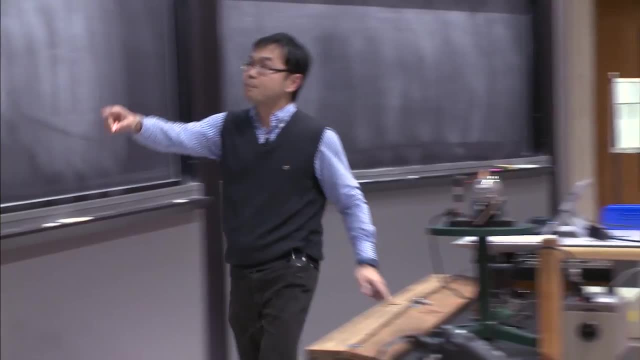 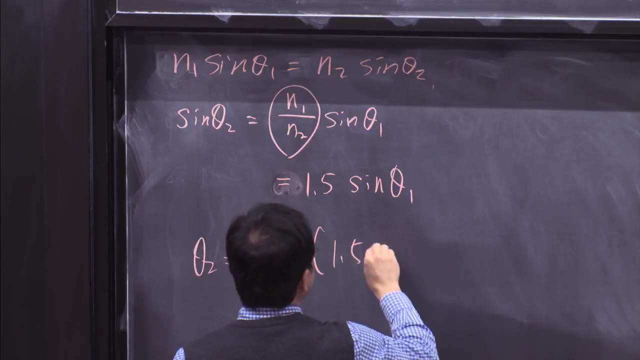 OK. So if I increase theta, OK, theta 1,. if I increase theta 1, at some point I will not be able to get the theta 2, right, Because theta 2 will be x sine 1.5 sine theta 1.. 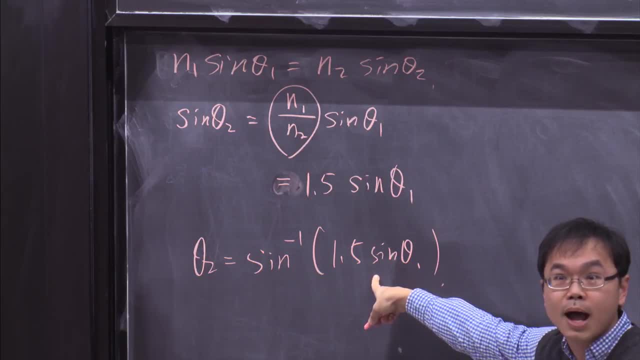 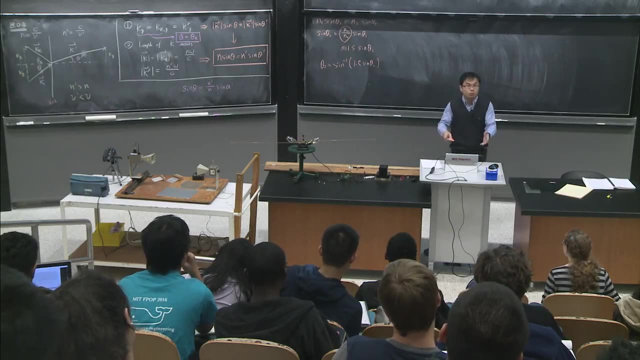 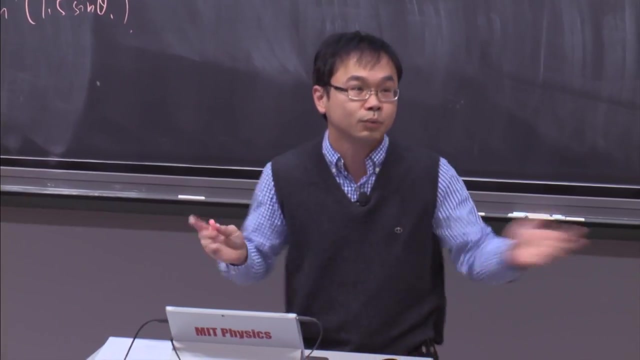 And at some point, 1.5 sine theta 1 will be greater than 1.. Then I don't have a theta 2, which can satisfy this equation. OK, So what will happen? Maybe the whole system explode, I don't know. 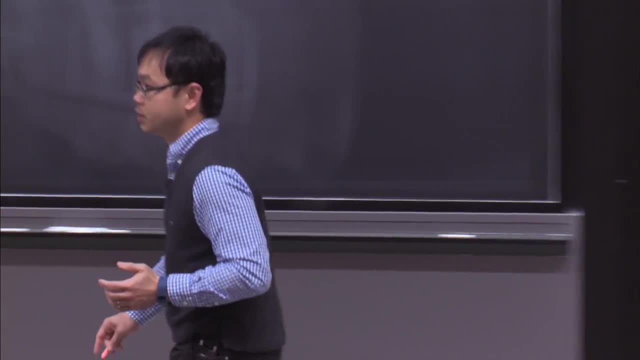 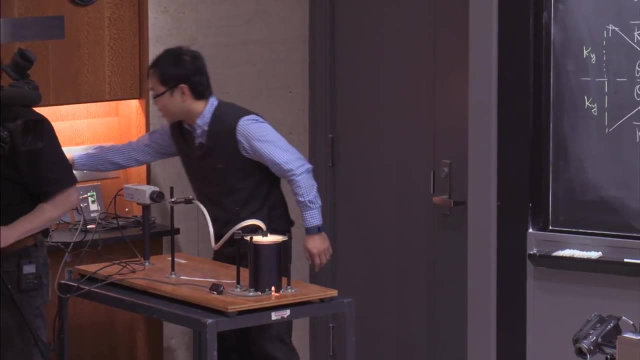 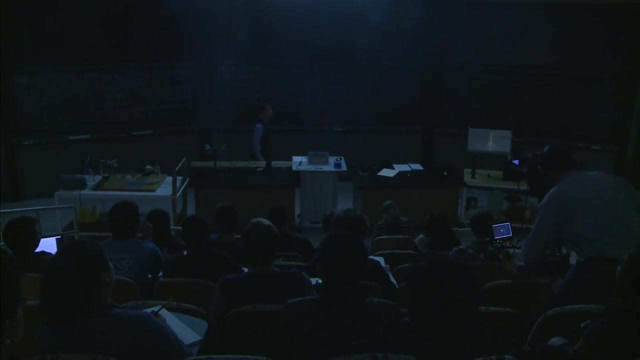 Right, So we are going to do a simple experiment to see what is going to happen. So, before we do this kind of dangerous experiment, we are going to turn this light off And be prepared. Hope everybody will survive. OK, So here I have a laser which is actually shooting. 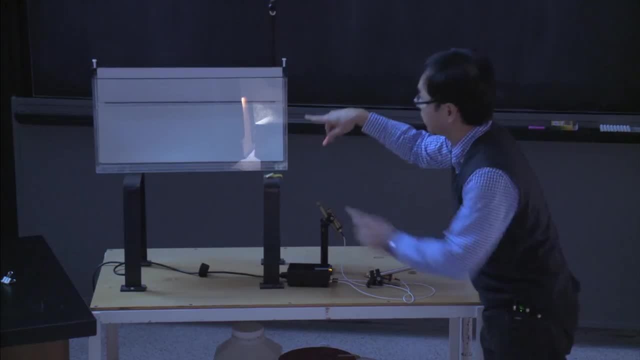 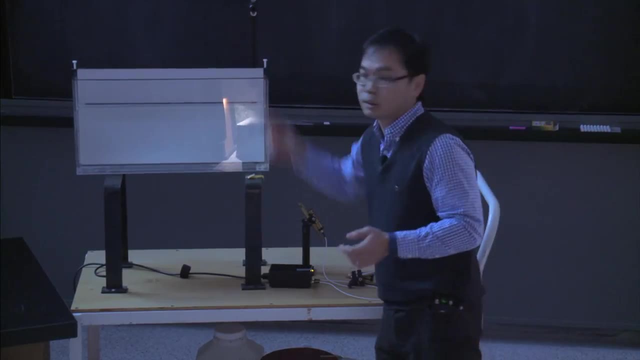 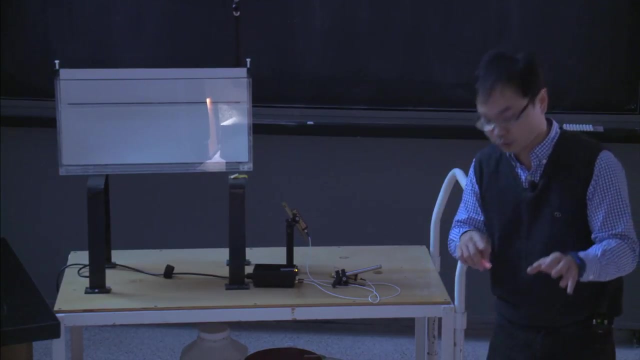 a laser beam through this tank of water. So this is water with n value roughly 1.33.. And outside of the water is air right. So the speed of propagation is roughly equal to the speed of the light, is actually roughly equal to c. 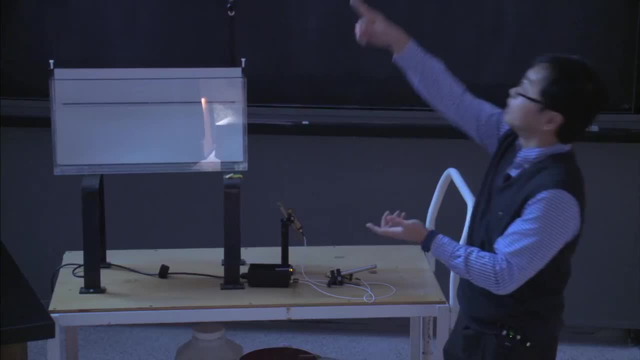 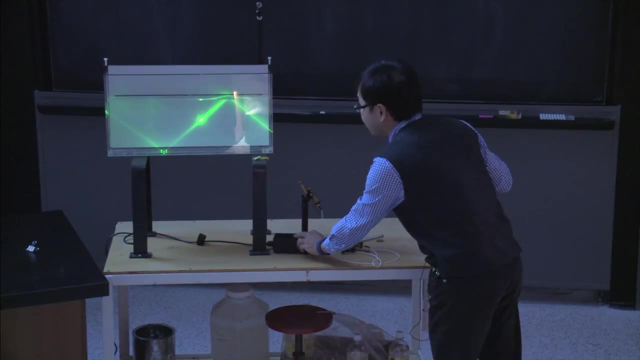 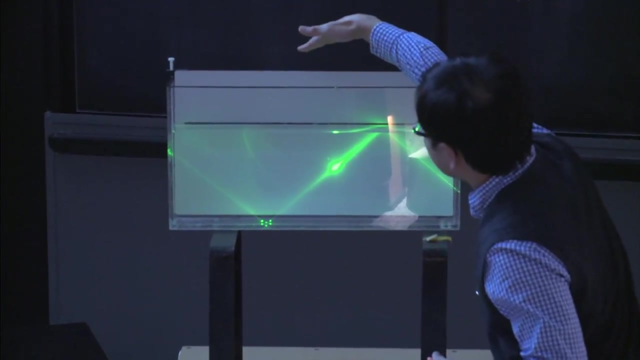 So that's actually roughly 1.. OK, So that's actually exactly the situation we are looking for, And let's turn on this experiment Careful. Wow, Look at this. You can see that here there was no light coming out. 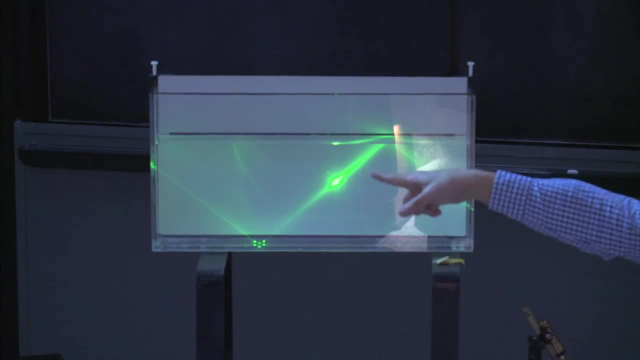 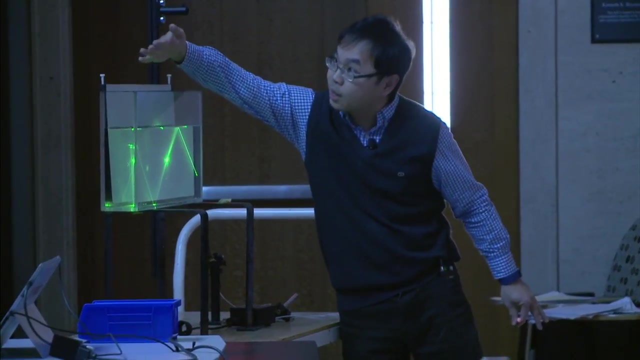 Right. Why is that? Because of the mathematics. Right. The mathematics say that, OK, sorry guys, This is not going to work. OK, Therefore, there will be no light really coming out. You can see my hand, OK. 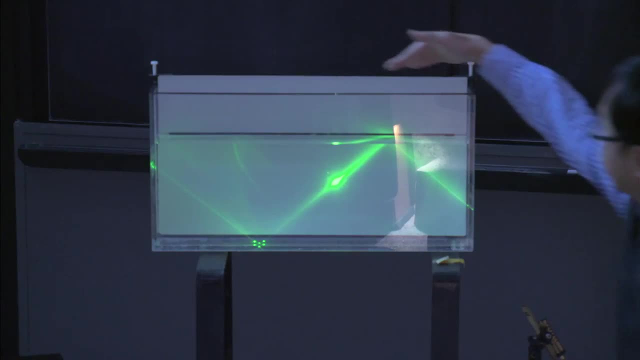 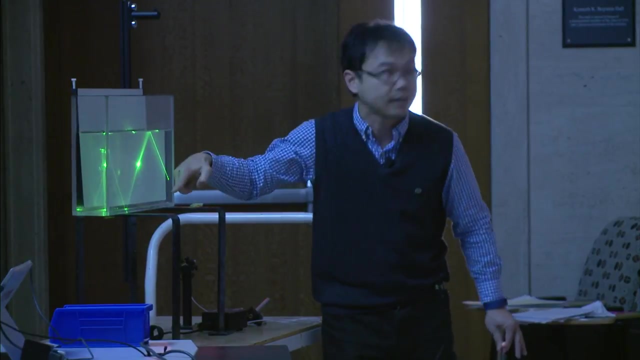 You can see the light here, right, When I put my hand here it's not burning my hand, But that is OK, All right. And you can see that nothing really comes out And all the energy are bounced back into the water. 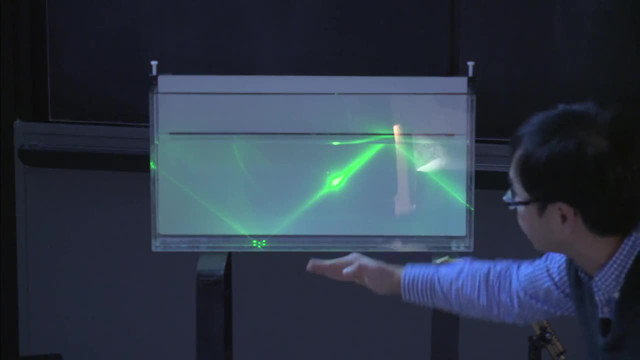 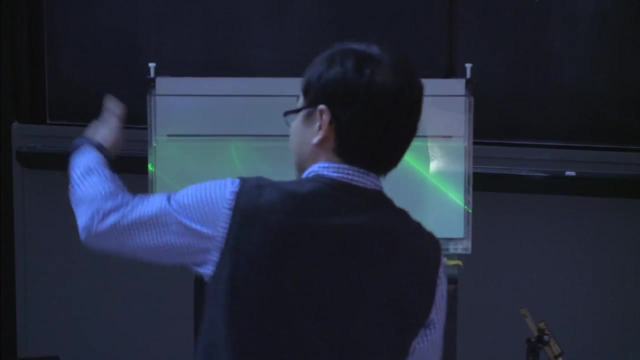 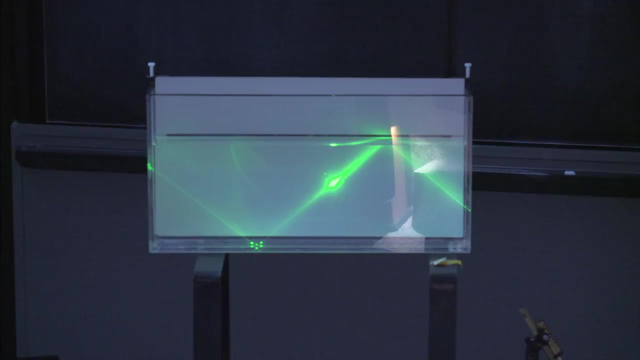 OK, The same thing also happened here. You can see that the light is actually bouncing back and forth and moving into where In the opposite direction, Until it passed through here, maybe because it's actually still bouncing around inside this tank. OK, 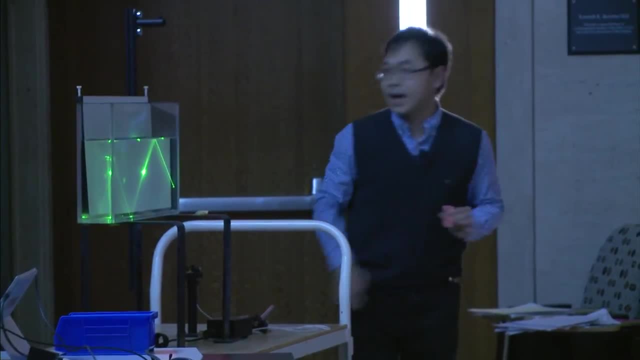 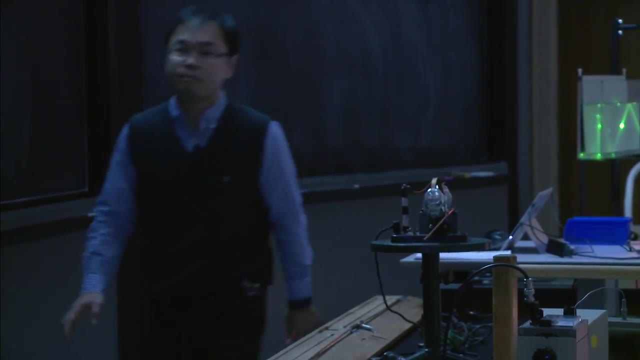 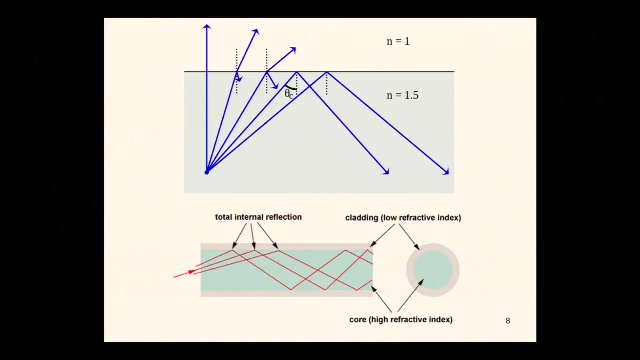 So the good news is that no explosion like what we have here. OK, The interesting thing we found is that all the energy will be bounced back if you have large enough particles. in this situation, As you can see from here, you can see that all the light energy 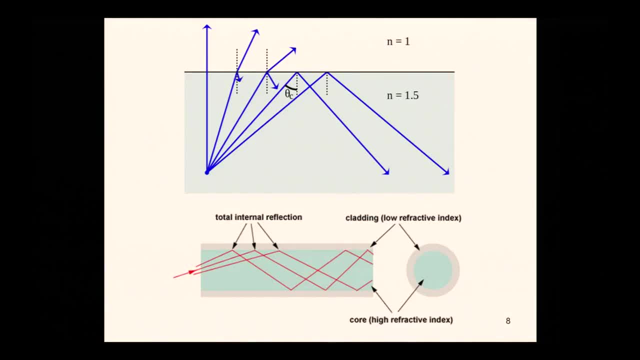 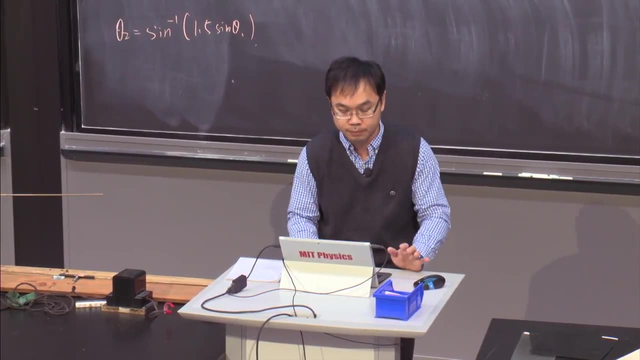 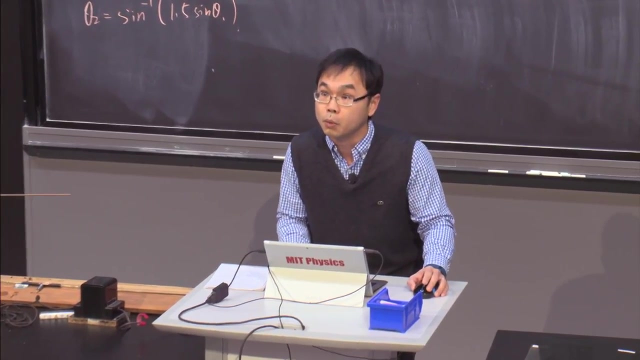 are bounced back into water. So that's actually very, very interesting, And that means we can probably make use of this property to send light. We can actually send some large material Right. So that's actually how optical fiber works, OK. 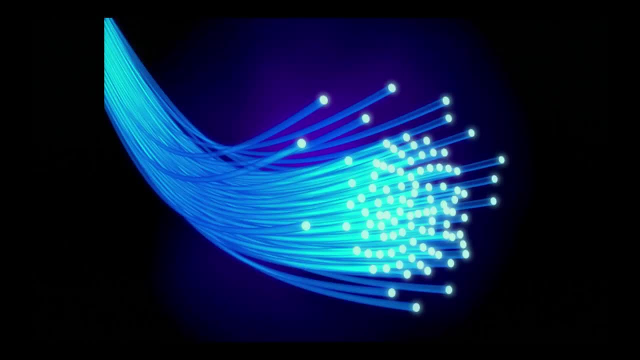 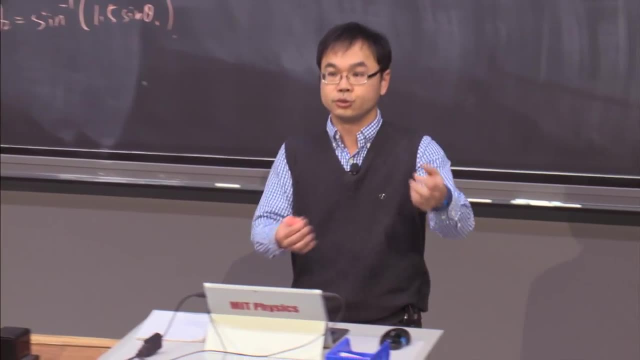 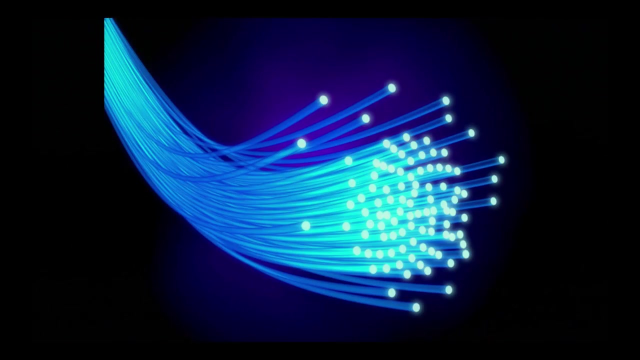 So basically, you can actually shoot the light into the optical fiber And the light is going to be bouncing back and forth between the boundaries inside the fiber And then you can actually send those information through light by this kind of mechanism. OK, So that's actually how the optical fiber actually works. 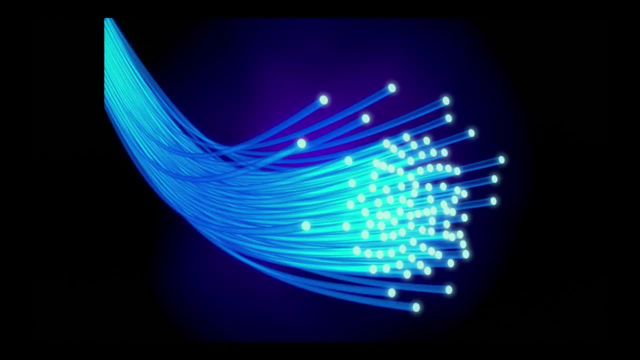 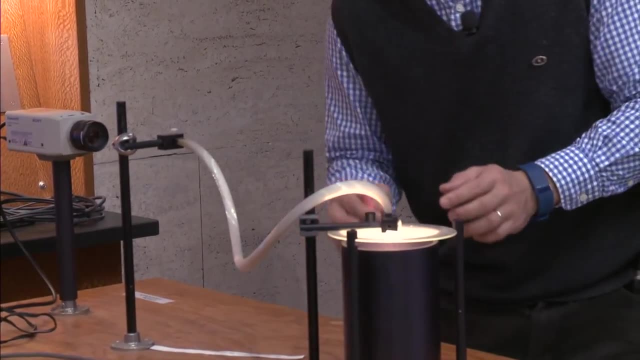 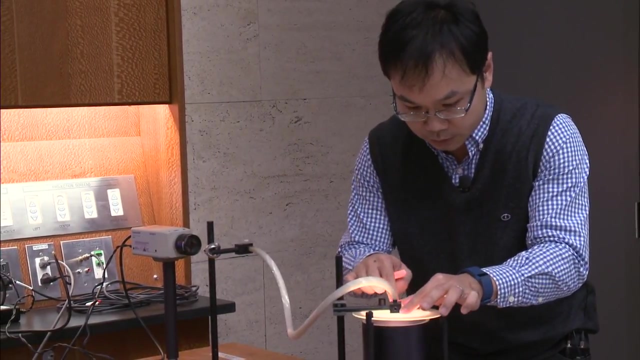 And here we do have a setup which I have light here shooting light into the optical fiber, And I have paper here which actually try to block part of the light. OK, So you can see from here, you can see the text which: 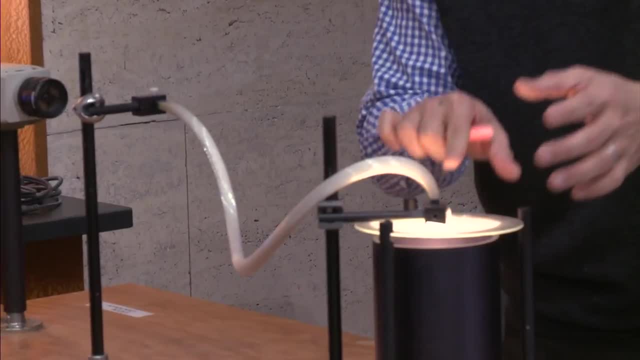 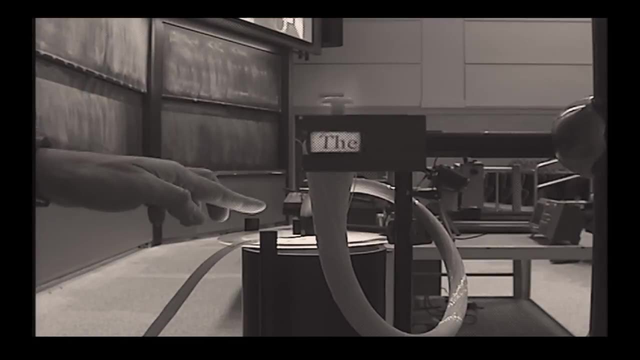 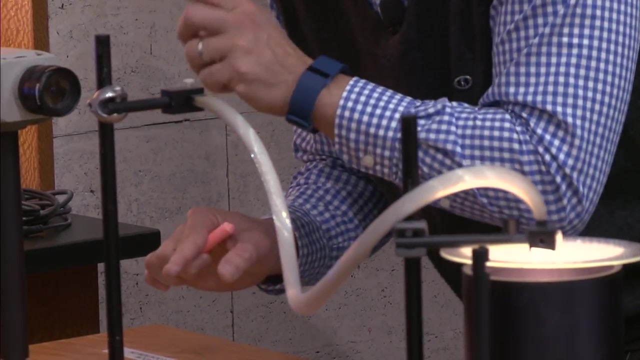 I put on the paper And you can see the text actually, because some of the light is actually blocked by this paper, the text on the paper And this light actually goes through this optical fiber OK, And continue and propagate and it. 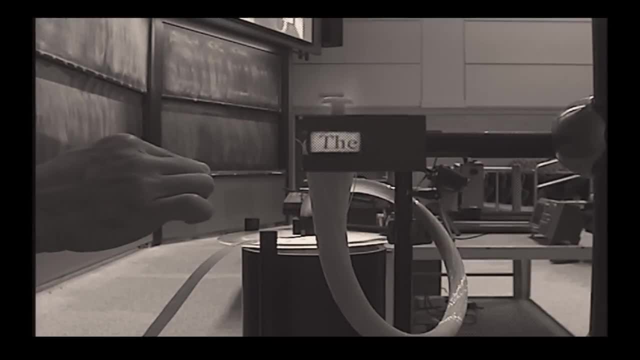 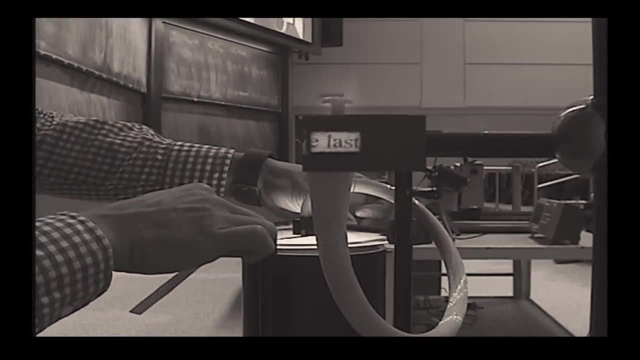 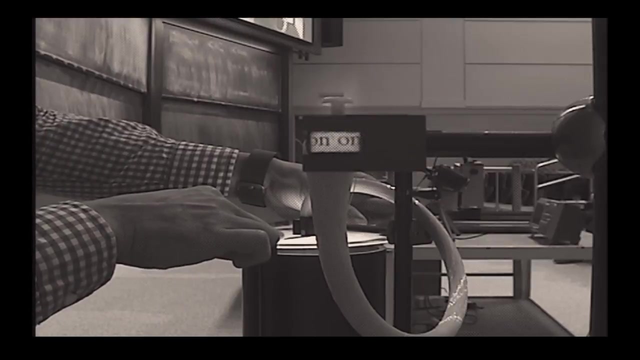 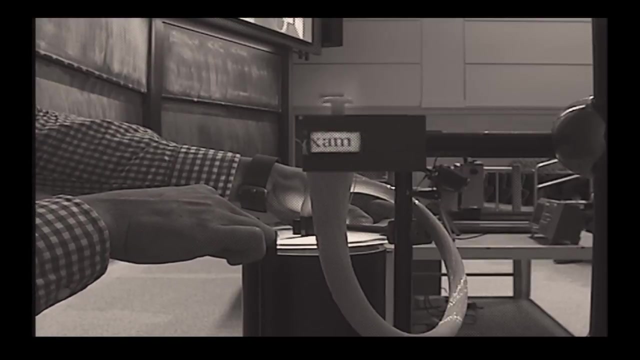 got captured by the camera. OK, So you can see what this actually is. Can you read loud what is actually written there? Can you see it Loud? So the exact is: oh no, no, no, no, no. 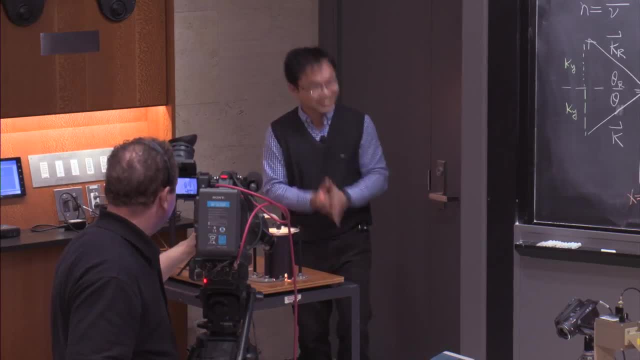 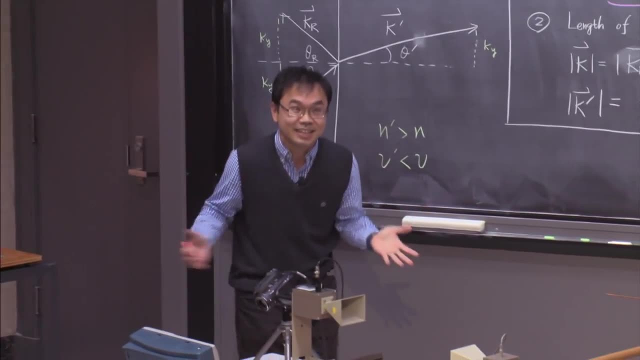 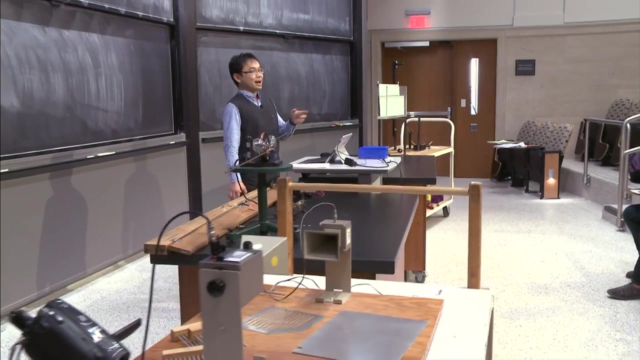 Transmission interrupted. Oh my god, All right. So I'm sorry It didn't work, But it worked in the beginning, right, And so you can see that this is a wonderful way to send optical signal And we actually do that, right. 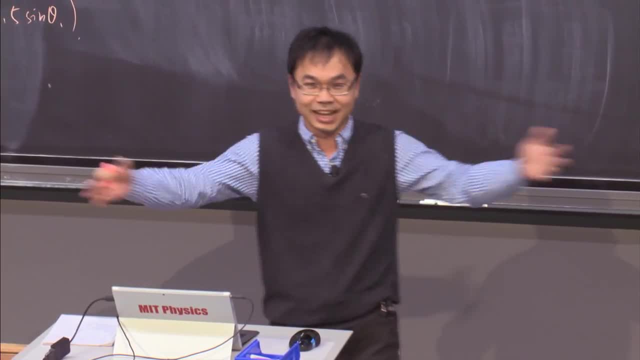 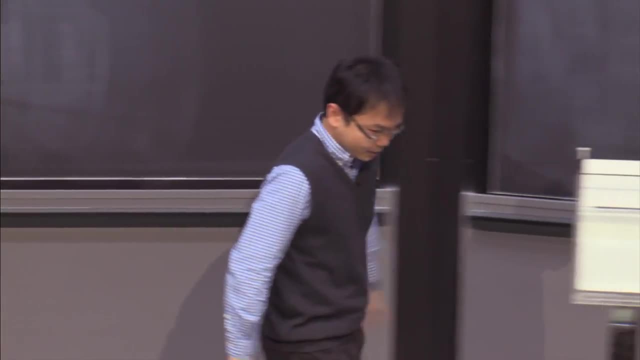 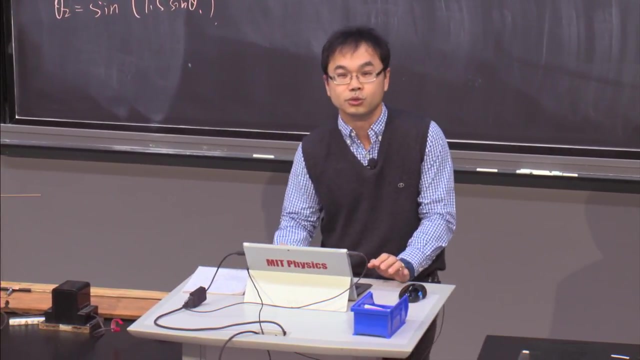 We send signal from US to Asia through all those crazy lines under the sea, right, So that's really cool. And finally, before we change the topic, I ensure that you enjoy doing the practice in your PSA 8. Because you are going to learn that. OK, this. 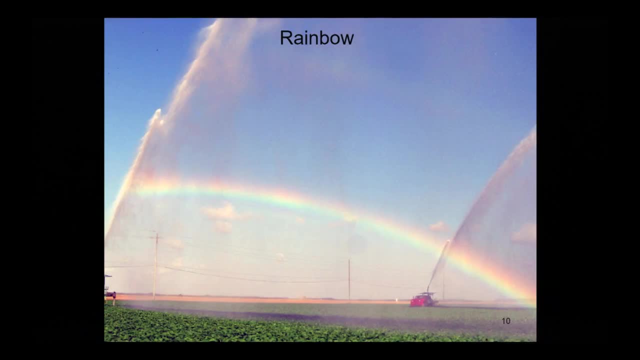 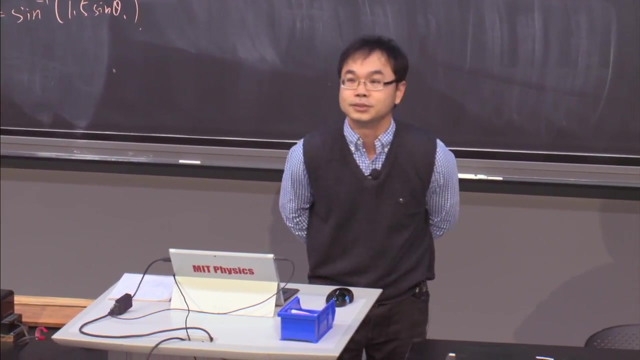 is actually highly related to beautiful phenomena we see in our daily life. The rainbow is actually really related to Snell's law And you are going to actually solve this problem in the PSA, All right. so any questions so far related to Snell's law and the refraction index, et cetera. 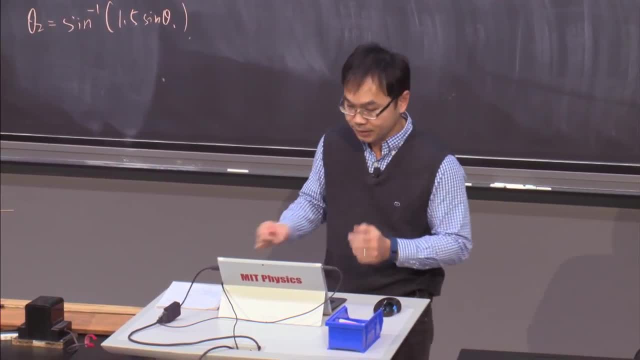 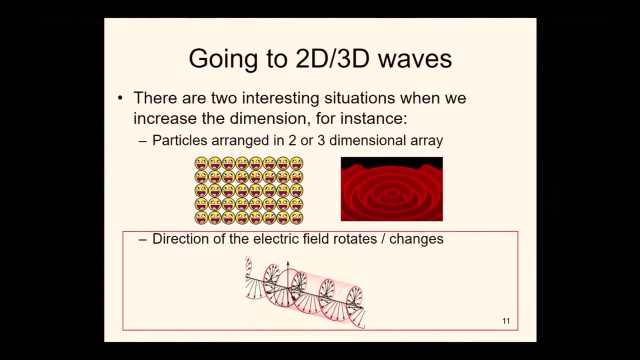 All right, So if not, we will go through. So let's go ahead and talk about the second example. The second example is that, OK, instead of introducing more objects in this array, we could change the direction of the oscillation as a function of time and see what is going to happen. 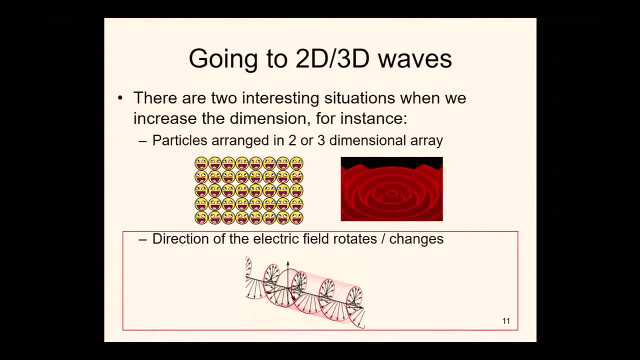 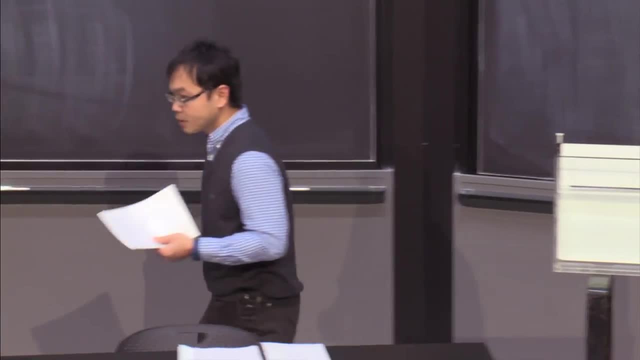 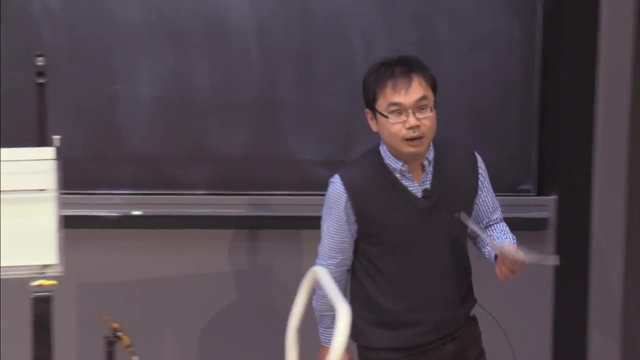 So the direction of, for example, the direction of the electric field, I can make it rotate or change as a function of time. So this is called circularly polarized wave, And that means we are going to talk about polarization today Before we start the lecture. what we are going to do is that 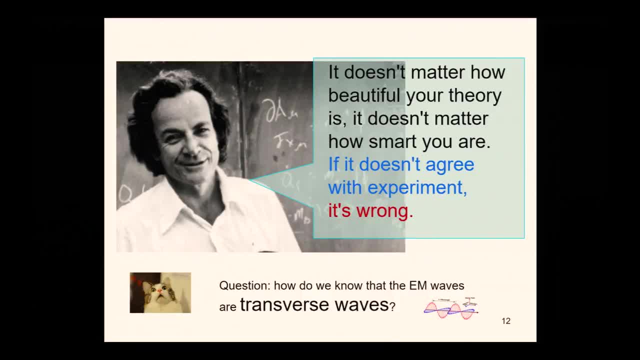 I will quote a word from Feynman: It doesn't matter how beautiful your theory is, It doesn't matter how smart you are, But if it doesn't agree with experiment, it's wrong. OK, So this is a very important lesson. 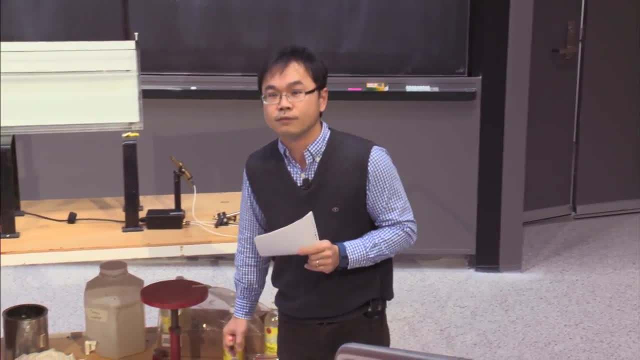 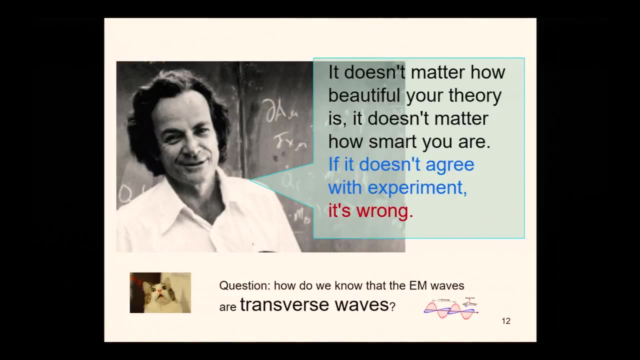 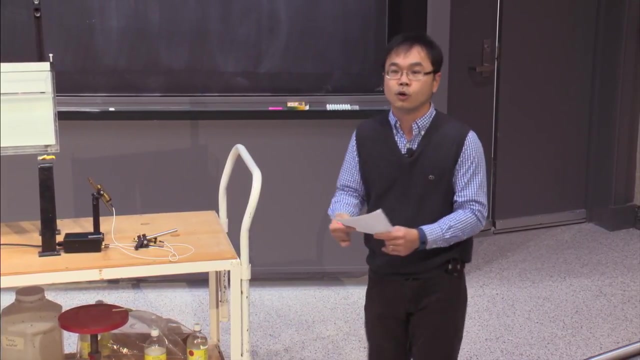 And I have been telling you that electromagnetic wave is predicted to be oscillating in the transverse direction, as you can see from that little figure right. So if the direction of propagation is to the right-hand side, so that means electric field and the magnetic field. 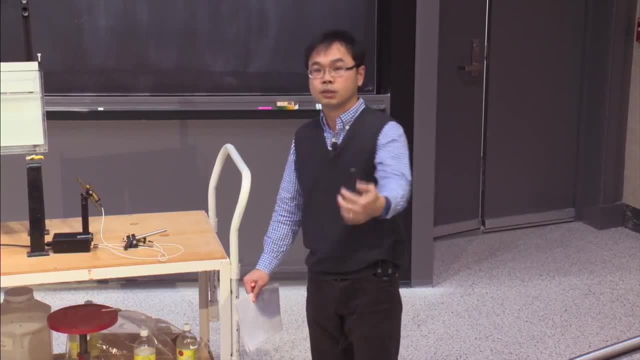 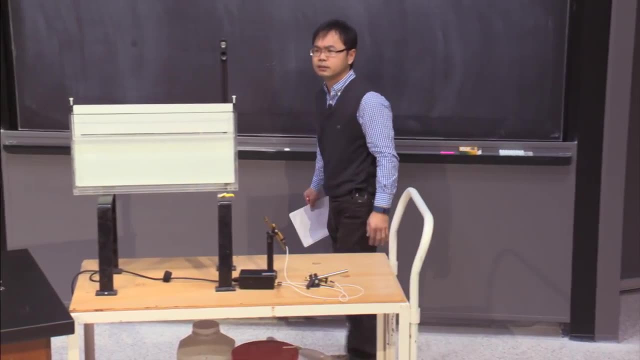 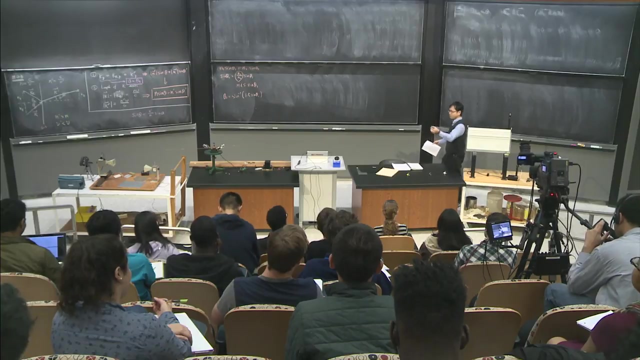 can only be oscillating in a plane which is perpendicular to the direction of propagation. That's actually what we have learned from Maxwell's equation. So all those things are theory right. Do you believe those theory? I'm not sure. Maybe light is actually oscillating. 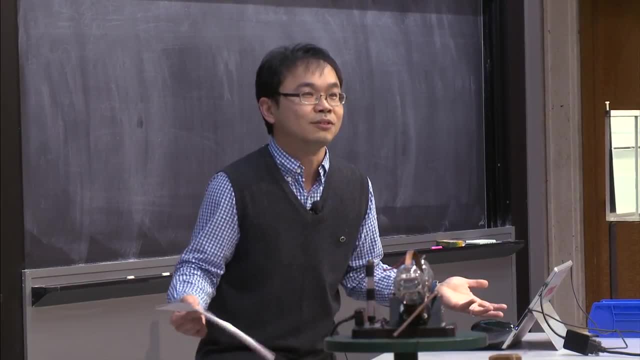 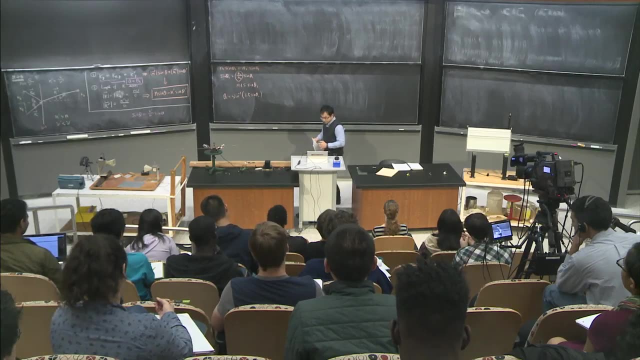 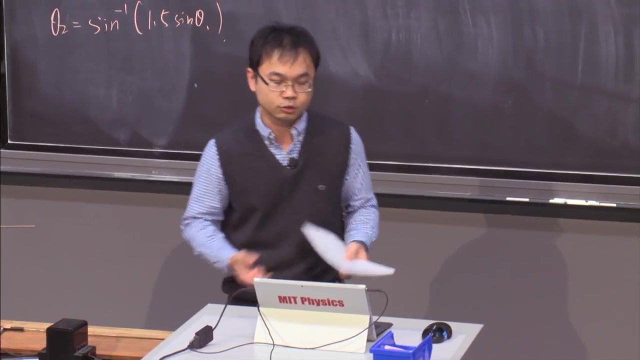 in the longitudinal direction, right? If you are a physicist, you should ask this question, right? Maybe you find something which is actually inconsistent with the theory. Then you feel really happy, right, OK, So the question we are trying to answer is: how do we know the electromagnetic wave are? 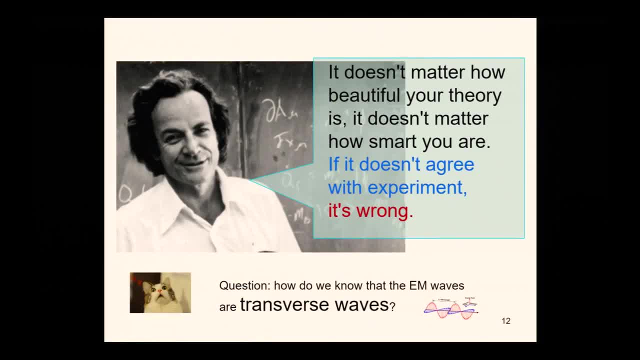 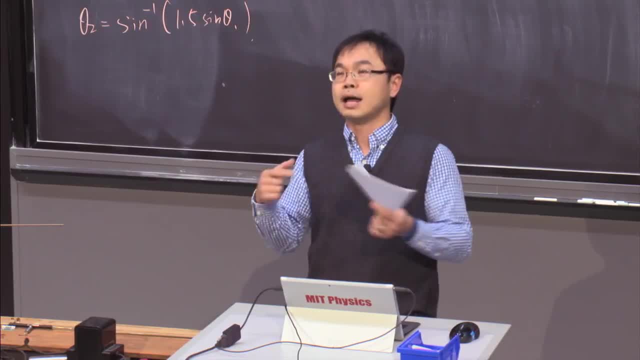 oscillating in the transverse waves right, And we are going to walk through a few examples and to convince ourselves: OK, maybe that's the case, Maybe we have some hint. Of course we cannot prove 100%, but very likely. 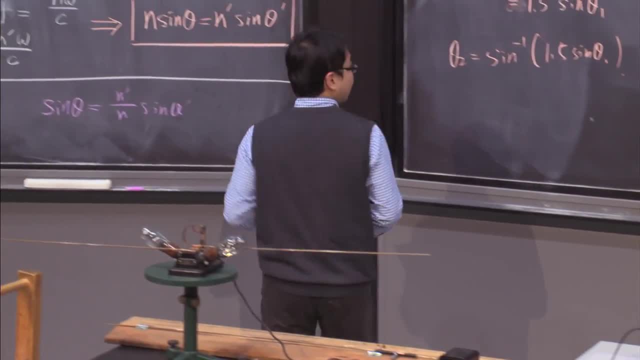 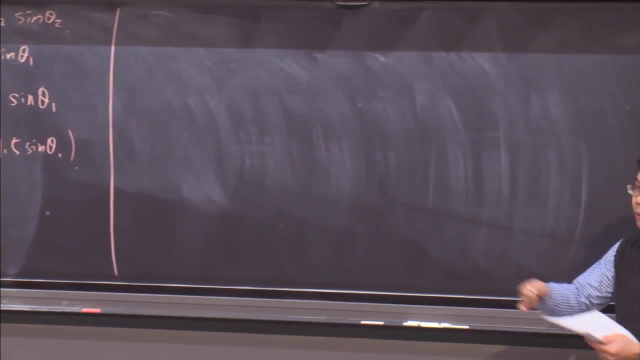 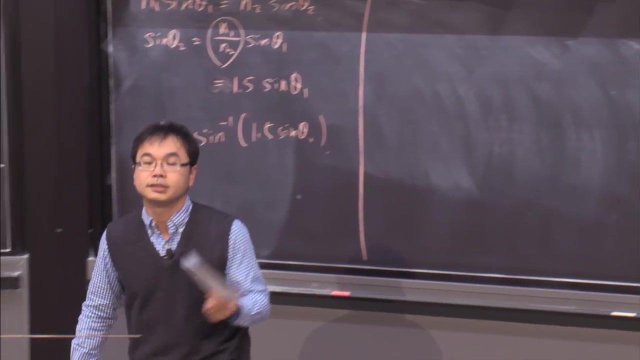 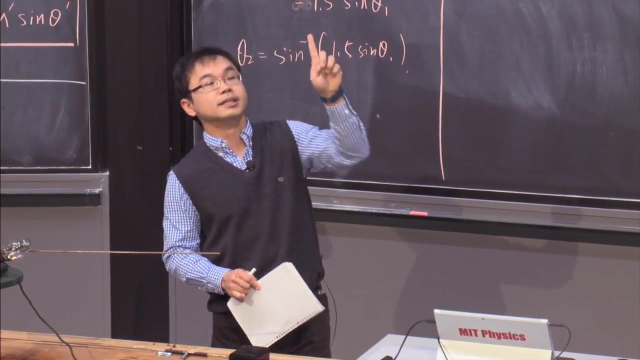 this is probably the case. OK, So let's go ahead and start the discussion today. So, instead of adding one more dimension by arranging materials, we can actually actually discuss how the direction of the oscillation, how the pointing direction of the electric field. 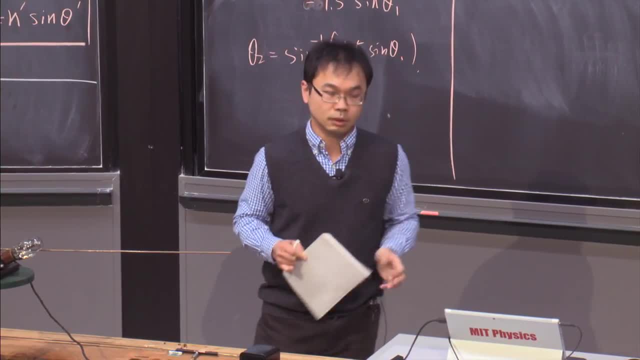 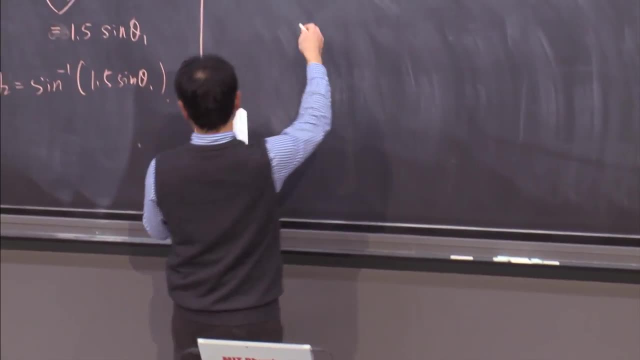 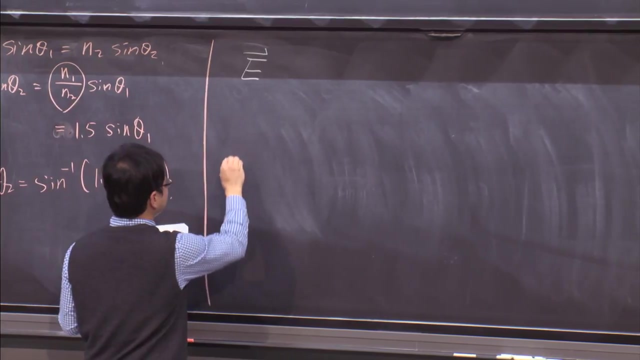 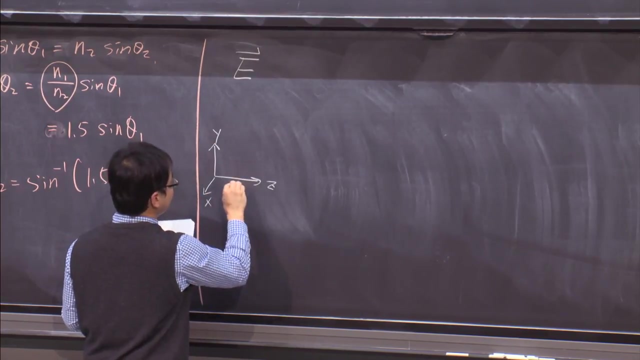 change or depends as a function of time, right? So in order to do that, I need to remind you how to write down electric field for the electromagnetic wave. So in a previous lecture, if I organize myself like this, the electromagnetic field is going in the z direction. OK, 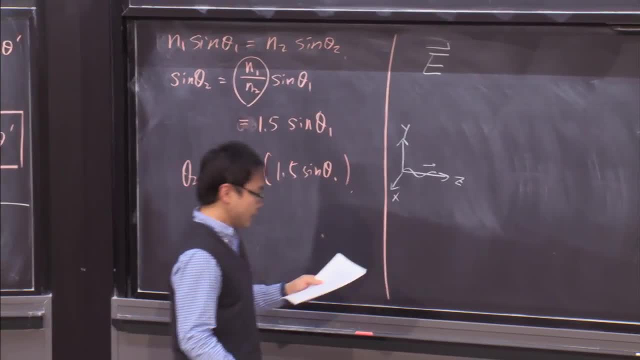 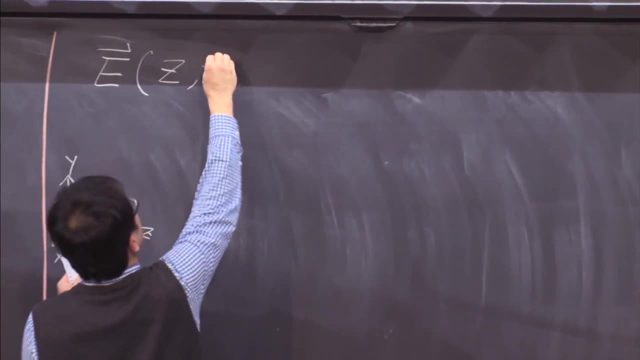 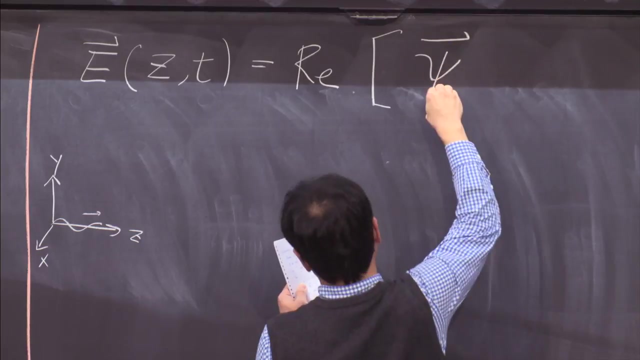 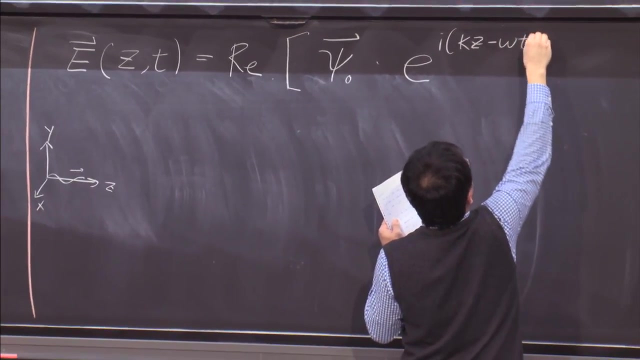 The electromagnetic field is going in the z direction. OK, All right, If I choose that, then basically the electric field as a function of z and the time will be equal to a real part of some vector psi, 0 times i kz minus omega t. 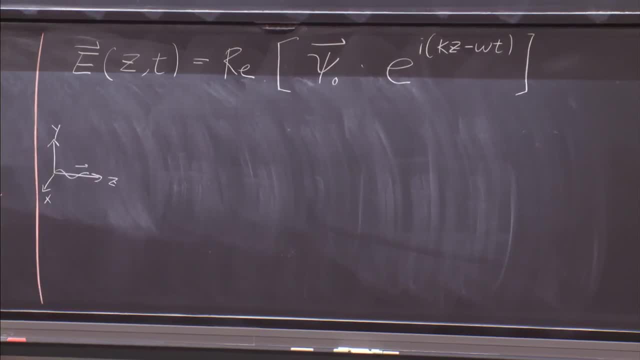 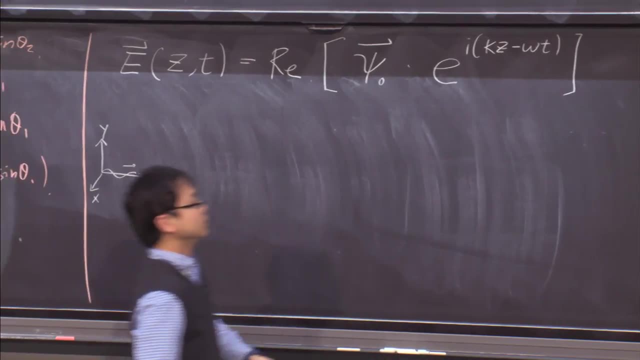 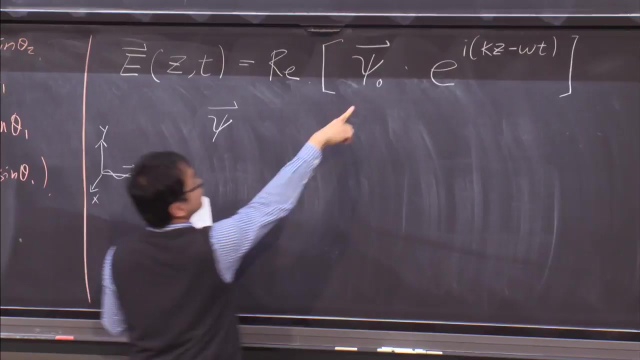 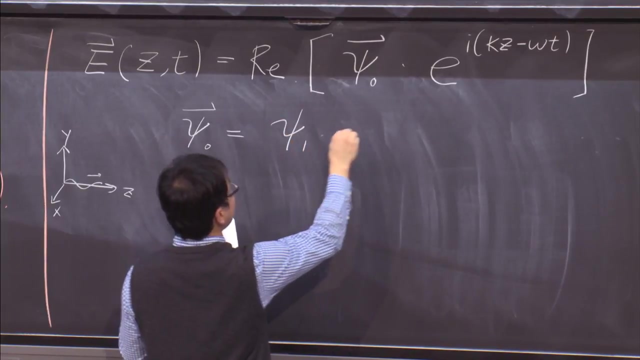 If I assume that this electromagnetic field is actually propagating toward the z direction, right, So by now you should get used to this already. This is actually going to the positive z direction. OK, Where I intentionally write psi 0, there is actually a vector which contains two components. 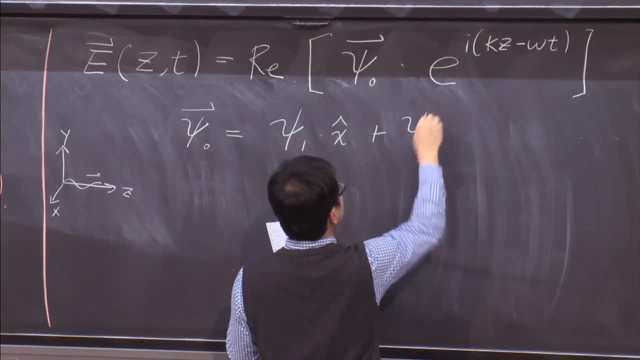 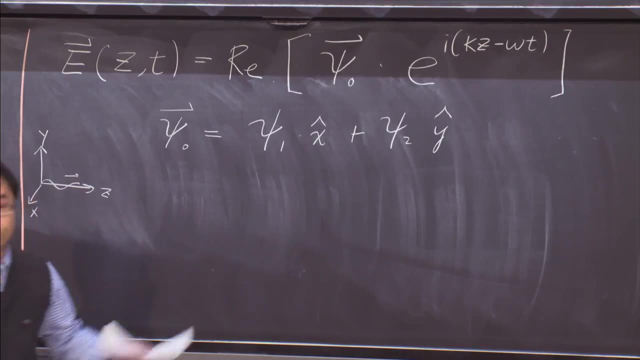 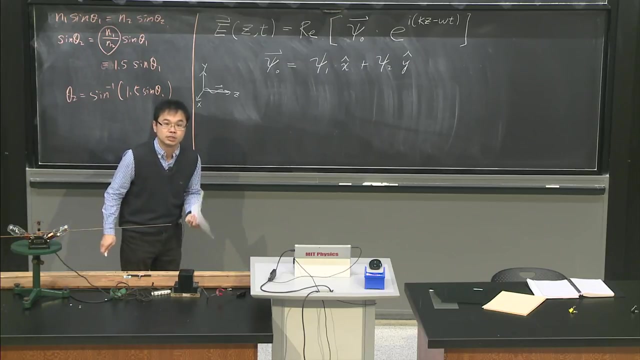 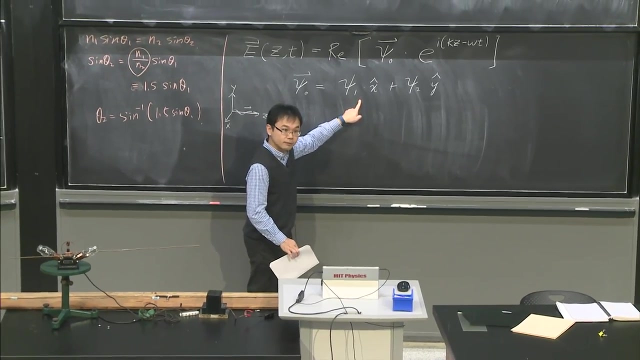 psi 1 in the x direction and psi 2 in the y direction. OK, And you can see from here that you can immediately recognize that this can be written as a superposition of two waves, right, So one is actually the electromagnetic wave. 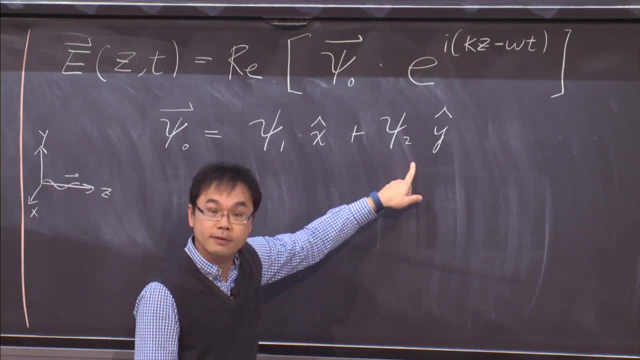 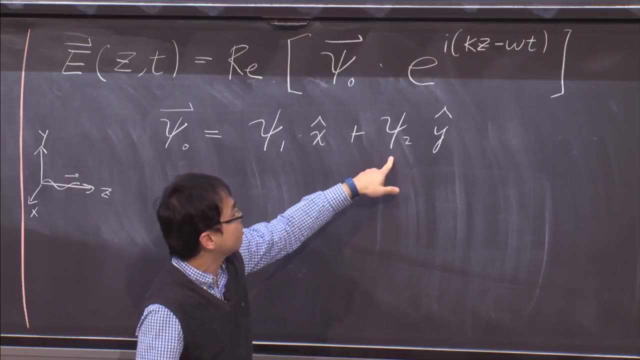 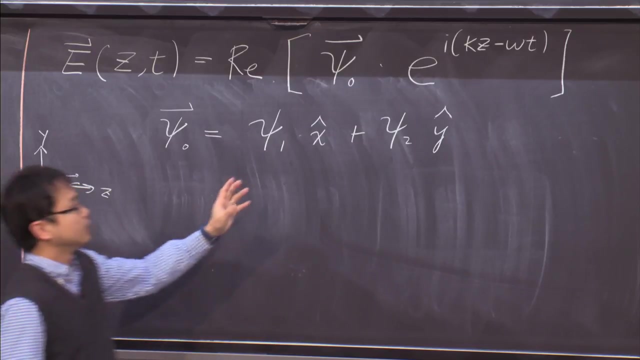 with electric field in the x direction And the other electromagnetic wave is actually oscillating with electric field in the y direction and with amplitude psi 2, OK. So that is actually what you can actually get immediately because of the superposition principle, OK. 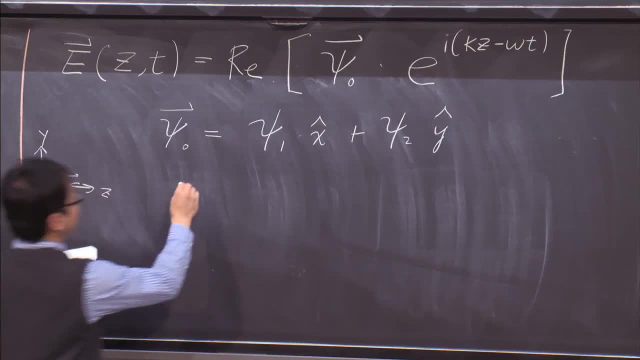 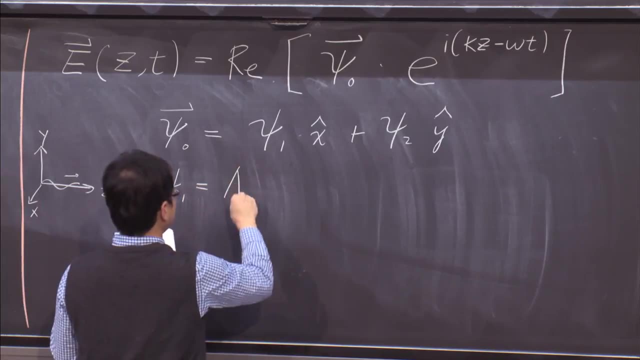 So it's actually a superposition of two electromagnetic wave And of course in this case I take the real part of this vector right. So in general, psi 1.. So psi 1 can be A1, exponential, i phi 1.. 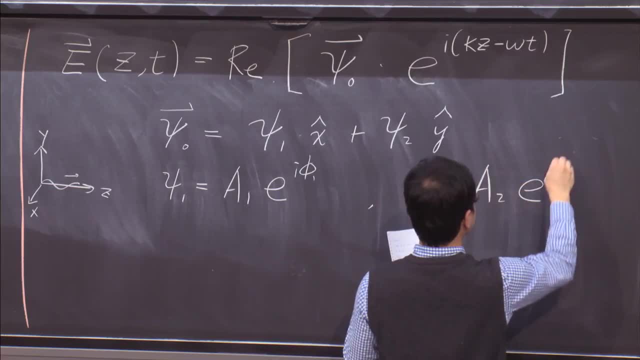 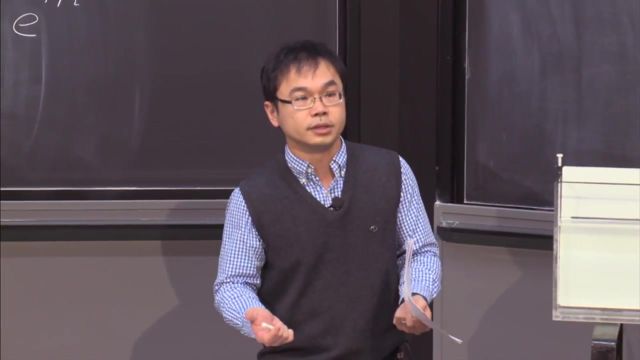 And in general psi 2 can be A2, exponential i phi 2, OK. So in this notation, basically we write everything in terms of vector And sometimes we actually write those things in terms of matrix, right, And that actually sometimes serves a better. 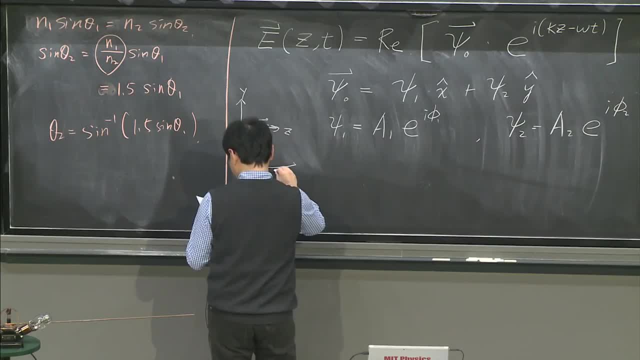 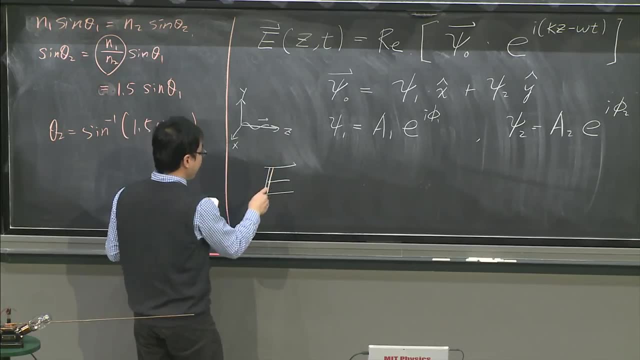 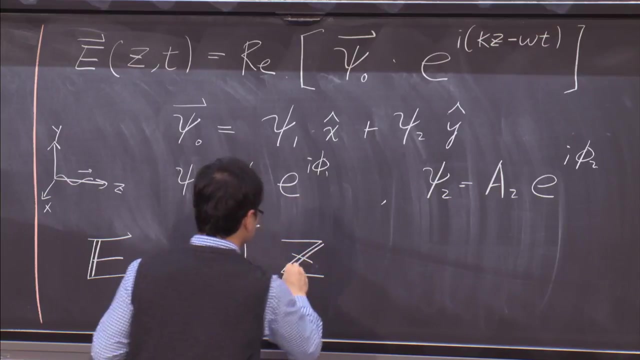 purpose for calculation. So we can also rewrite this thing in the matrix form. So I have a matrix E which have two components, Ex and Ey, And this is actually equal to a real part of some z vector- Sorry z matrix- which also contain two component. 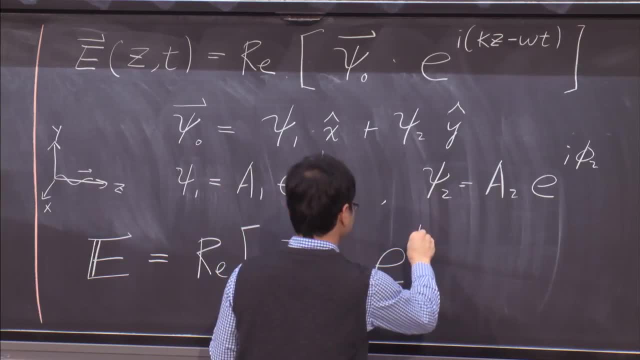 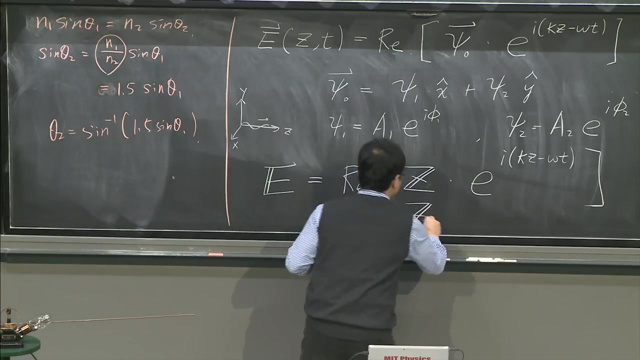 psi 1 times a scalar which is actually exponential: i kz minus omega t. OK, So, as you can see, I am now just setting up the language we want to speak right, So that we communicate right. So in this case, the z matrix is written as psi 1 and psi 2,. 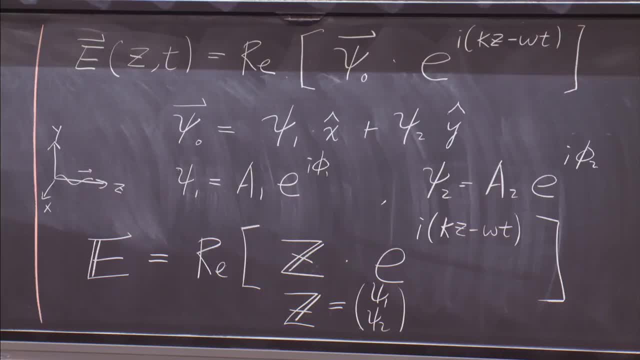 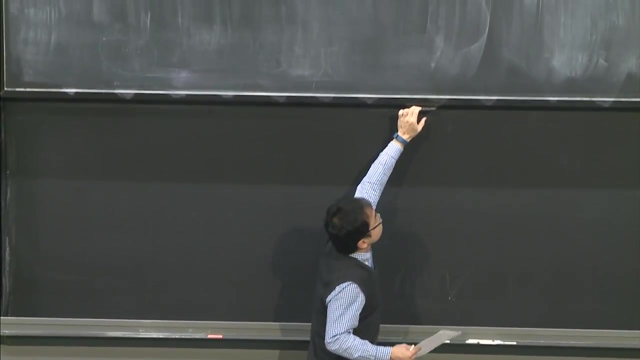 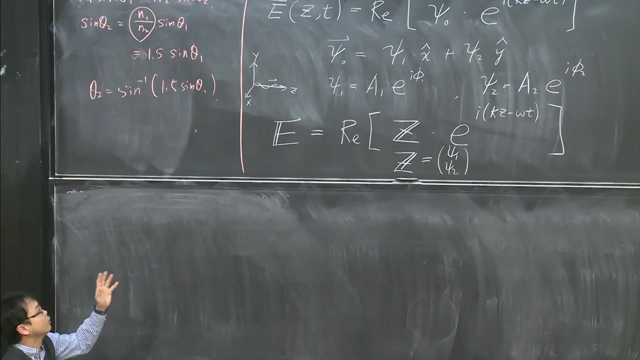 which are the two components? One is actually in the x direction, The other one is in the y direction. OK, And we are going to use this language and see what can we learn from this. So you can see that we have been doing. 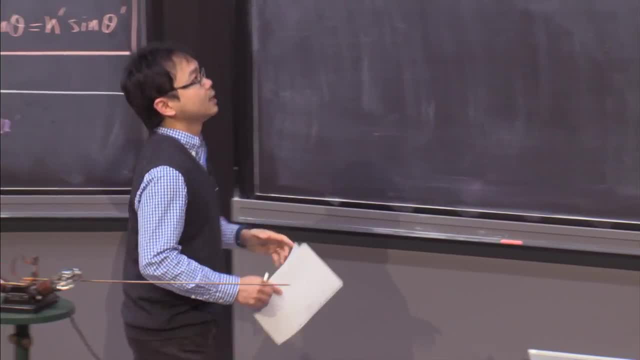 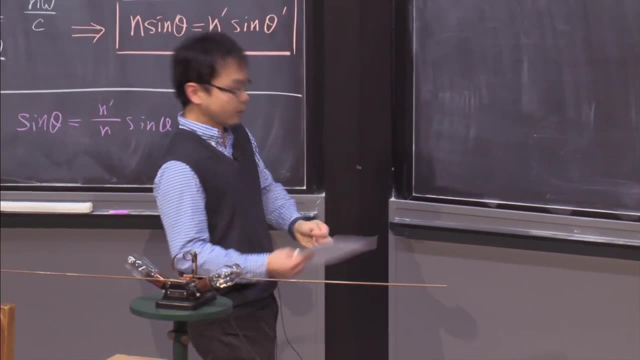 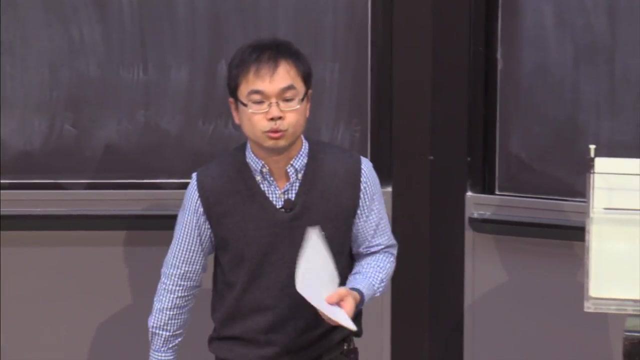 we have been discussing electromagnetic wave which is propagating toward the positive z direction, And I have two components which I can have: x direction electric field and y direction electric field. OK, So let me try to go through some example and see what we can actually learn from this. 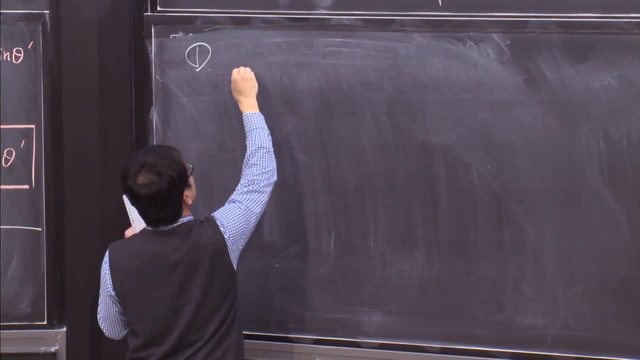 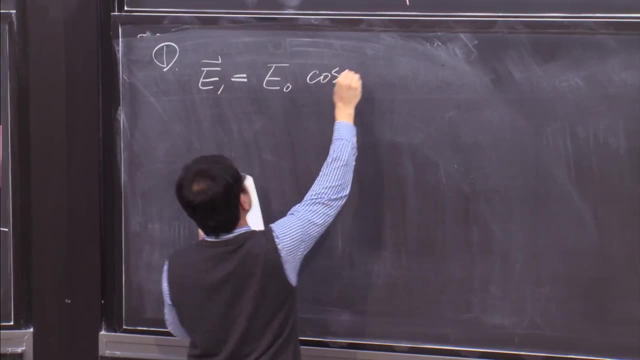 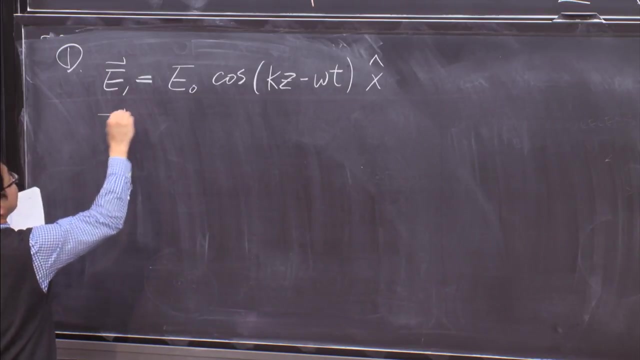 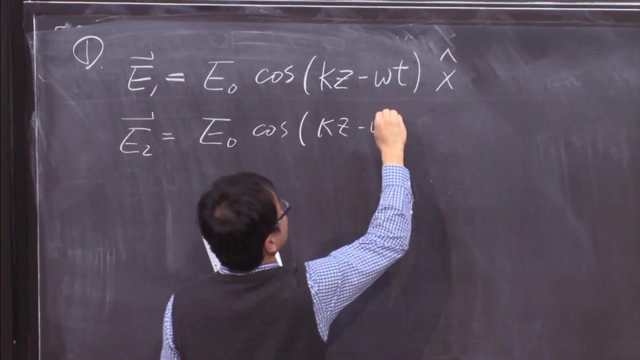 So the first example I would like to talk about is that if I have two waves E1,, the first wave is actually E0- cosine kz minus omega t in the x direction, OK. And then the second wave is E2, equal to E0- cosine kz minus. 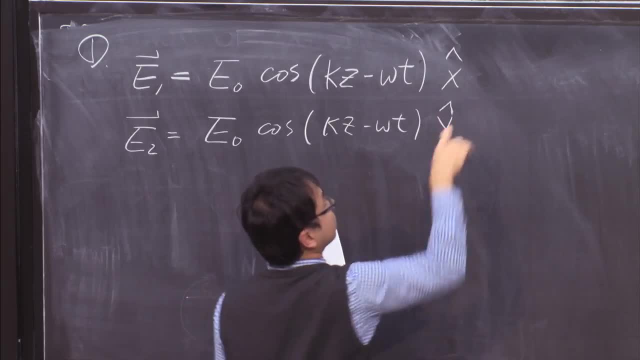 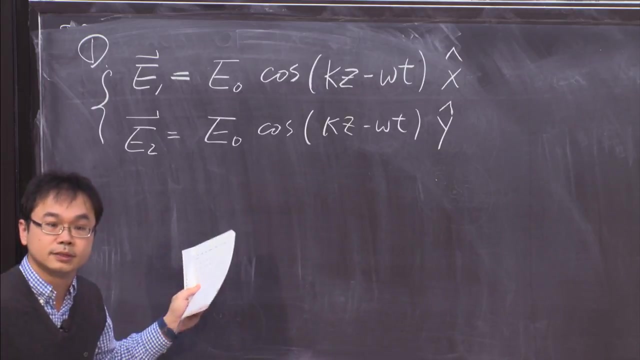 omega t in the y direction. OK, Careful, The direction of the electric field is different for the first and the second plane wave. OK, And if you notice, if you actually notice from this expression, these two waves are in phase. 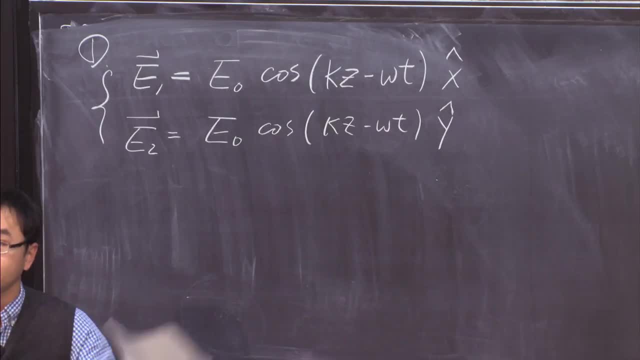 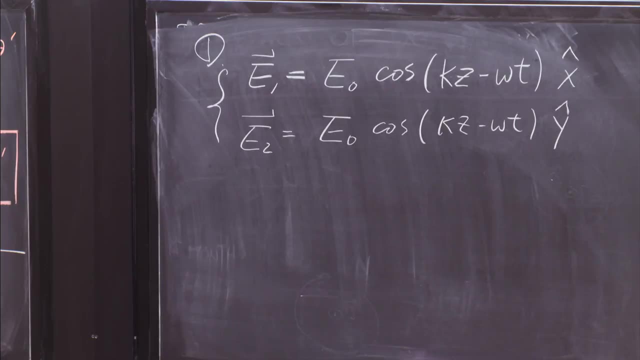 Right, So in phase means that they reach maxima at the same time. OK, So in this case, if I add two waves with no phase difference, what is going to happen? So I am going to have an E vector which is actually E1 plus E2.. 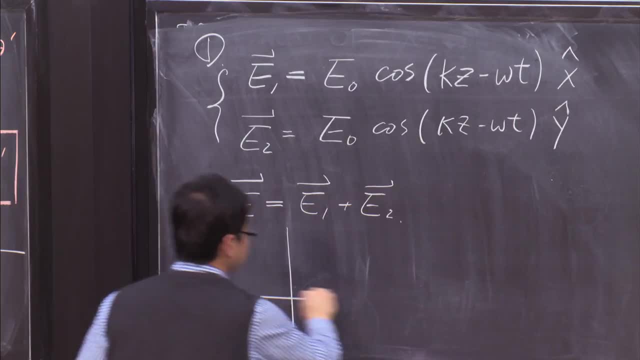 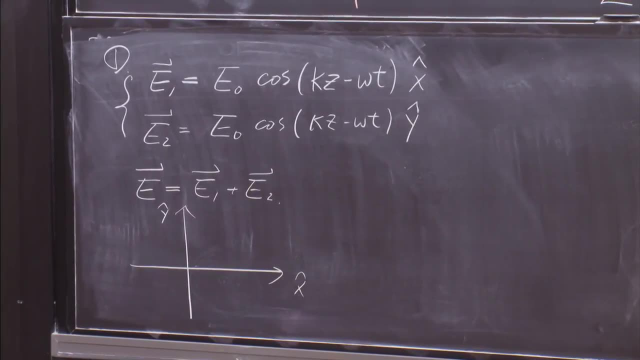 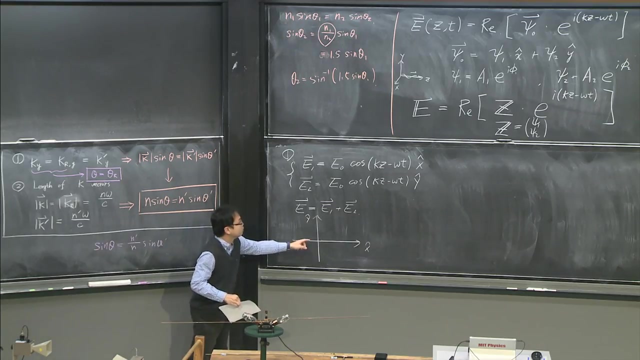 Right, And if I plot the locus of this kind of electric field which is in the two-dimensional space x and y? so now I am fixing my z position, for example, at 0.. And I would like to see how the locus of the E 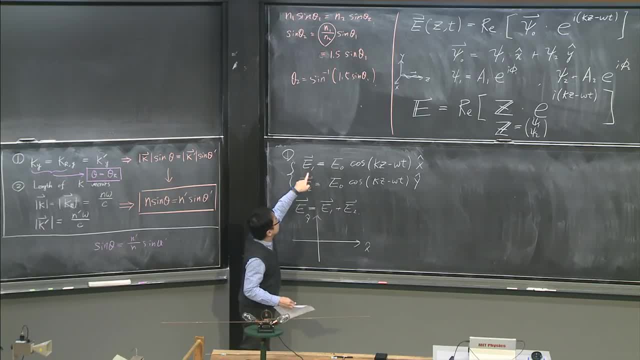 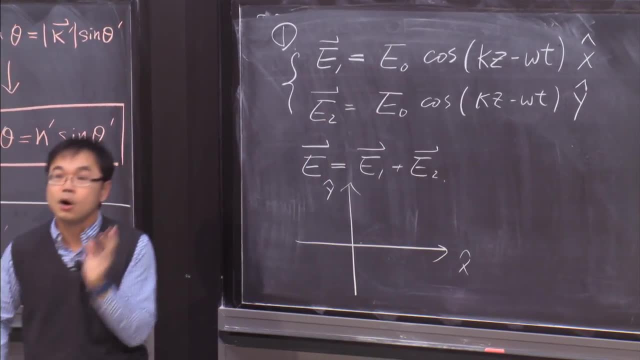 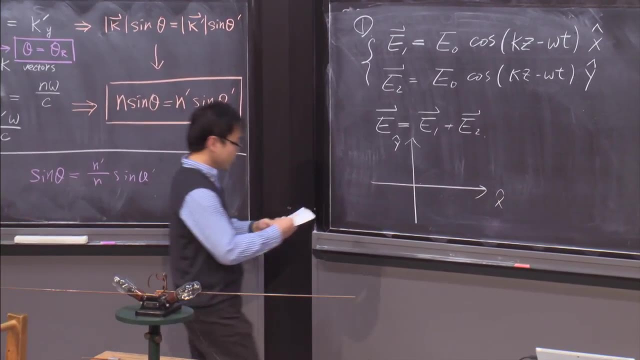 vary as a function of time. OK, In this case, since E1 and E2 have the same amplitude, which is E0. So they have no phase difference. That means they reach maxima simultaneously. So that means originally, for example, in the beginning: 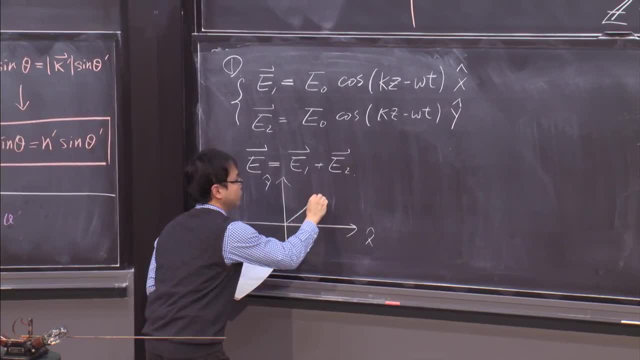 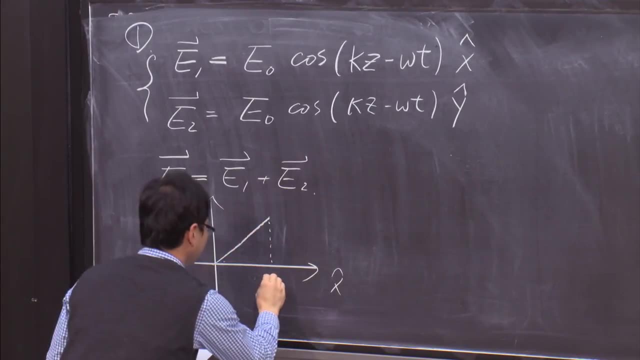 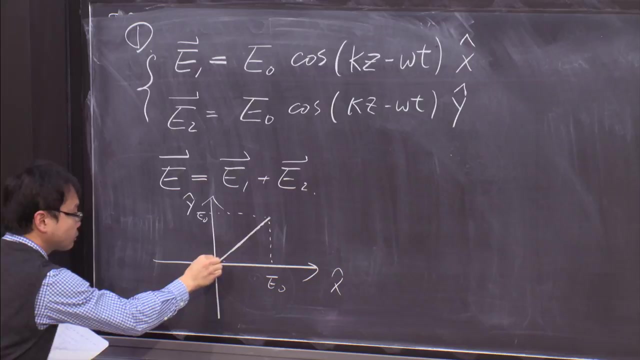 the electric field is 0. And this electric field projection to the xy plane will increase until some maxima. At the maxima this will be E0.. The x and y projection will be E0. Then it goes back, Right. 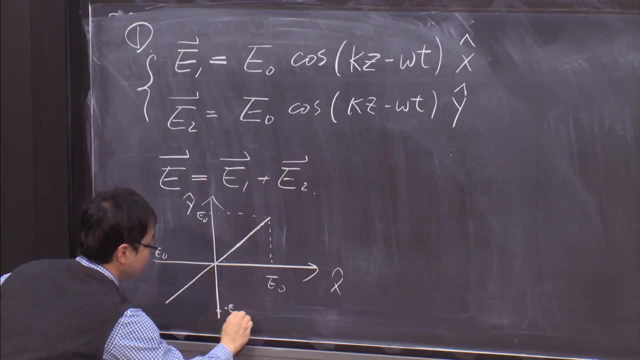 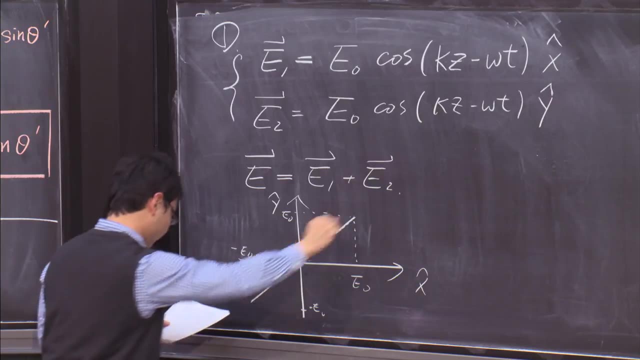 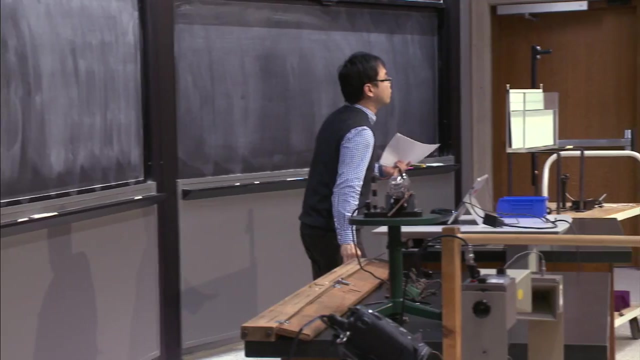 To minus E0,, minus E0 in the x and y direction projection, And it goes back and forth. OK, So in this case this is actually still not very different from what we had discussed before, Right, Because the electric field is actually still 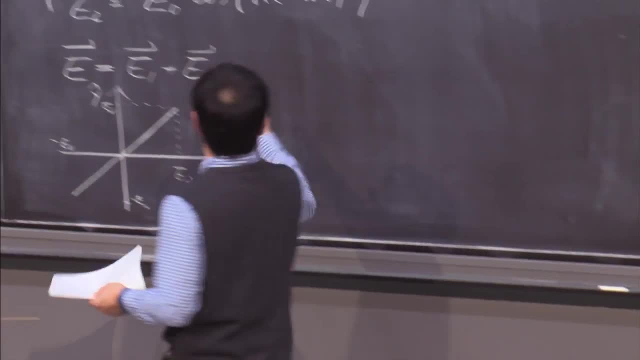 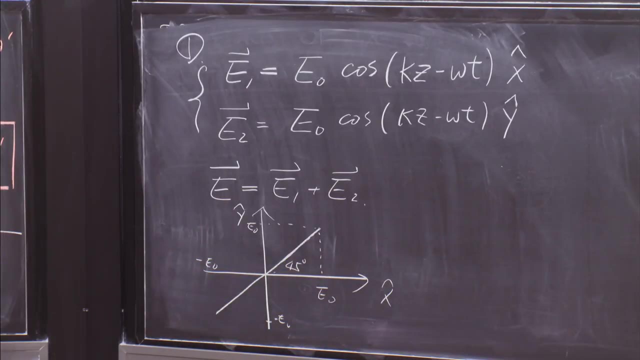 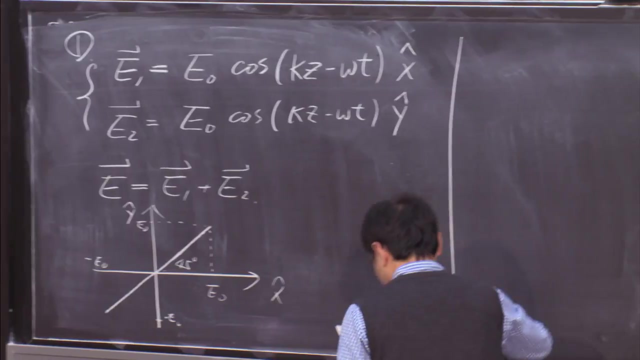 oscillating up and down, But the difference is that it's not oscillating at the x-axis or y-axis, but in an axis which is actually 45 degrees with respect to the x or y-axis. OK, And now we can do an exercise to write it down. 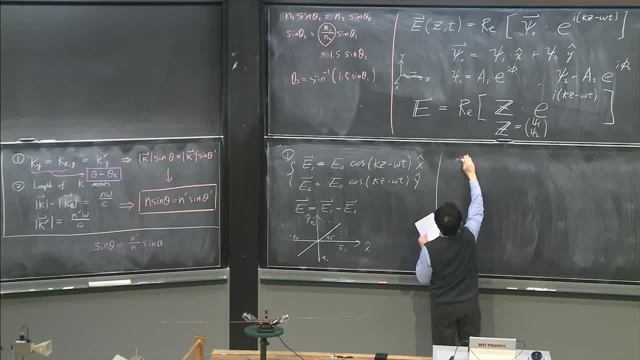 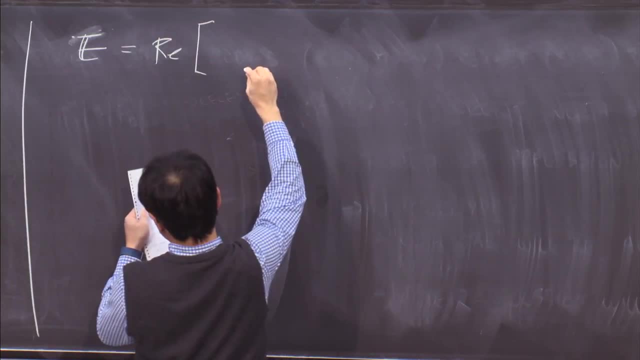 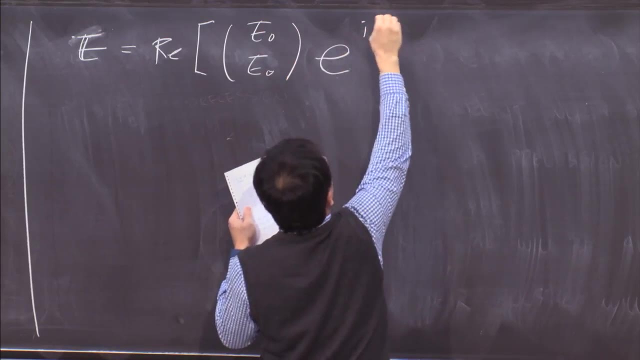 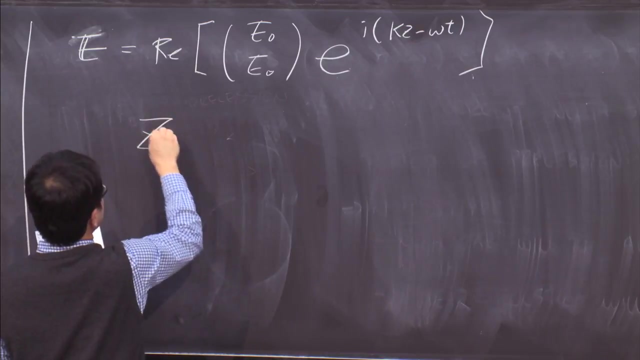 in the matrix notation. OK, Now I have this: E matrix will be equal to the real part of E0, E0.. And both E0s are real exponential i, kz minus omega t, And basically I can conclude that z will be equal to E0, E0.. 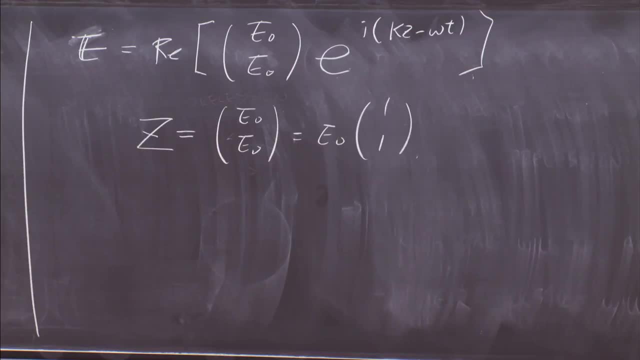 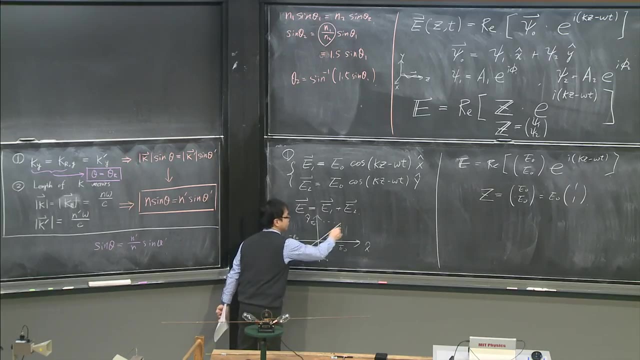 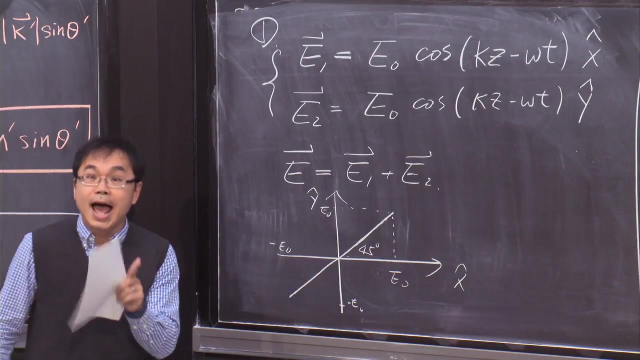 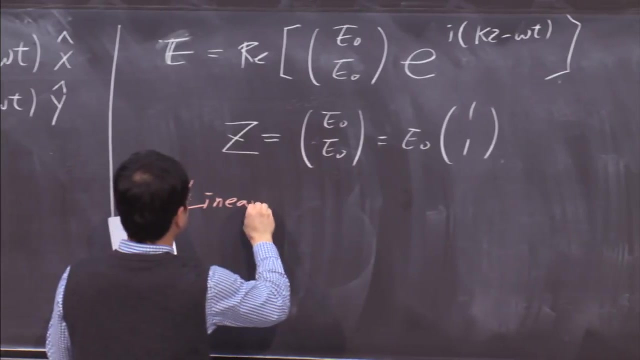 And this will be E0,, 1,, 1.. OK, In this kind of situation the electric field is oscillating as a function of time. The projection to xy plane is a line. When that happens, we call it linearly polarized. 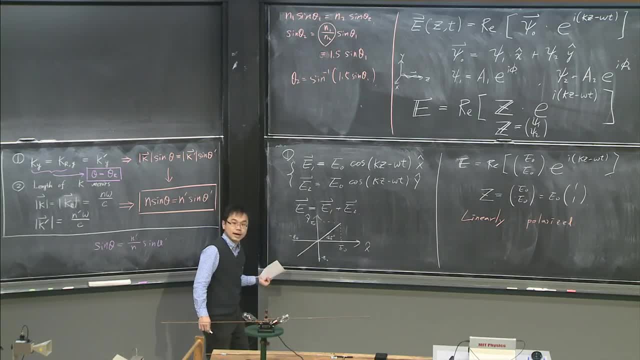 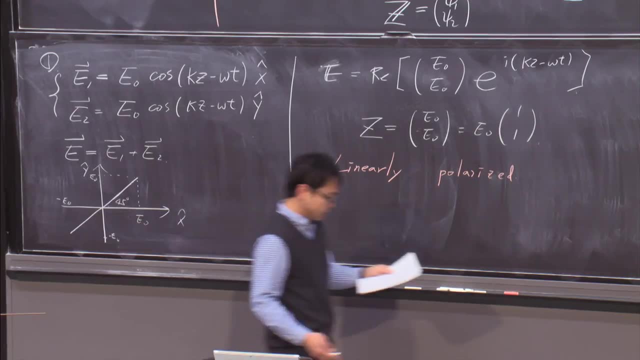 OK, So this is actually just a name, But indeed the locus of the electric field in the xy plane is a linear line. OK, So that actually we call it linearly polarized, OK, And of course you can say: OK, this is actually. 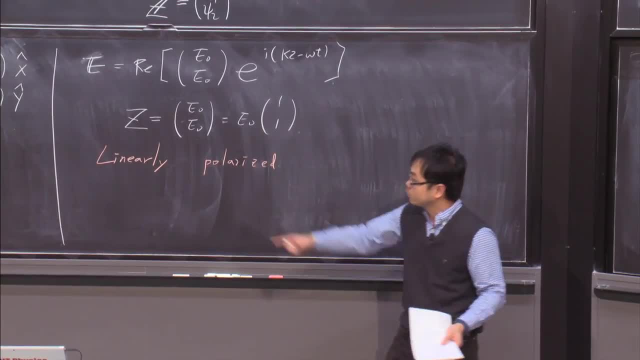 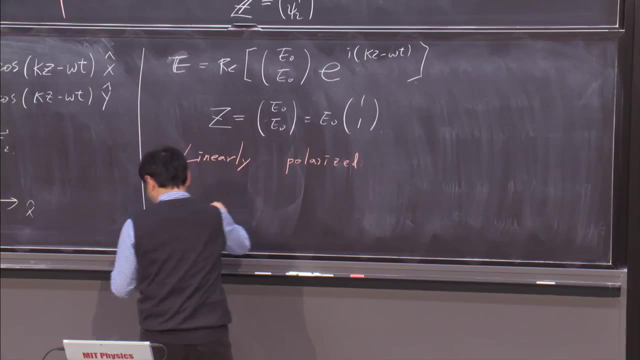 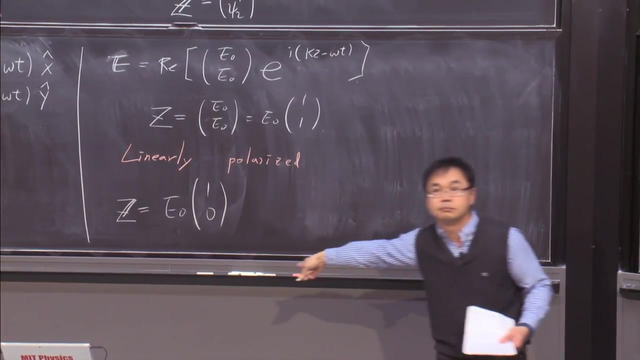 just one example Right. I can have many, many examples which you also create a line when you plot the locus Right. So, for example, I can have z equal to E0, 1, 0.. Can somebody tell me what does that notation mean? 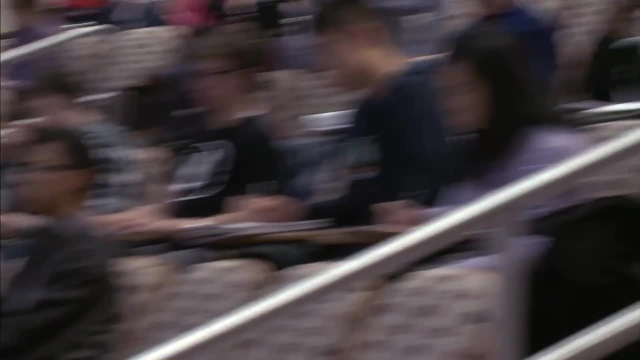 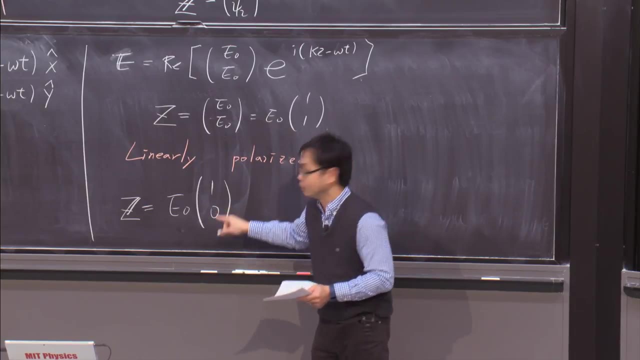 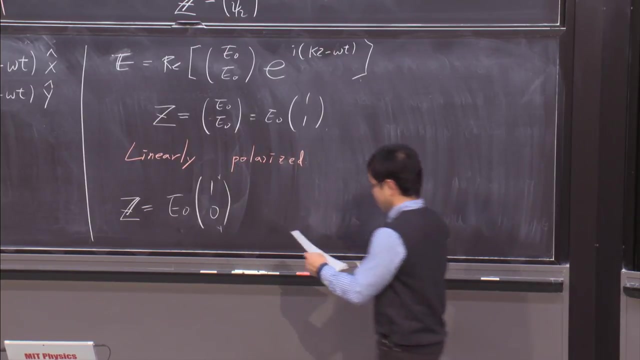 That just means one direction, That's right. So that means you only have electric field in the x direction, Right? So this is the x direction, This is y direction And this is also linearly polarized. OK, Of course you can have very similarly E0,, 0,, 1.. 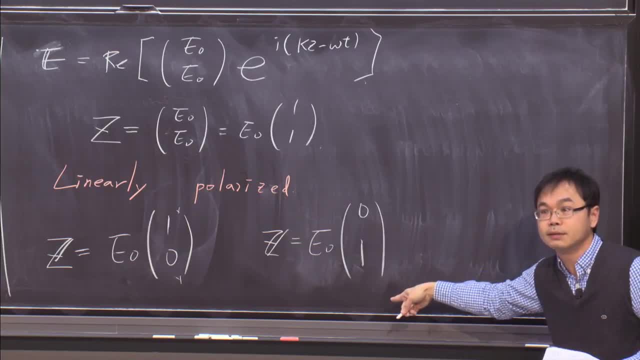 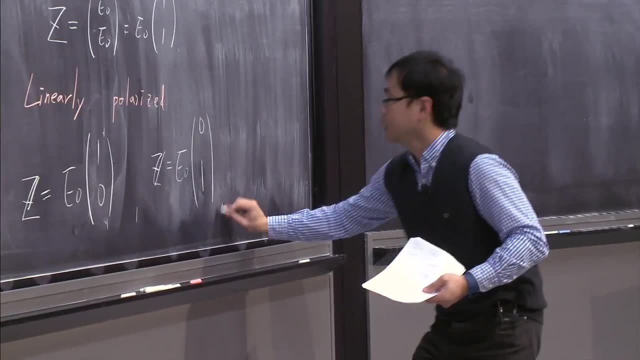 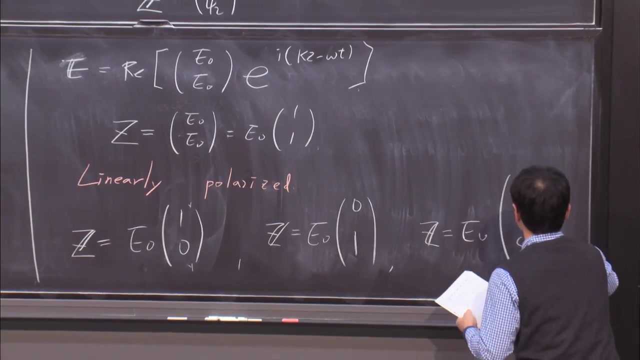 And in this case you only have electric field in the y direction. OK, So I don't want to tell you my language. OK, I'm introducing here. OK, So that we communicate. And of course you can have z equal to E0, cosine theta sine. 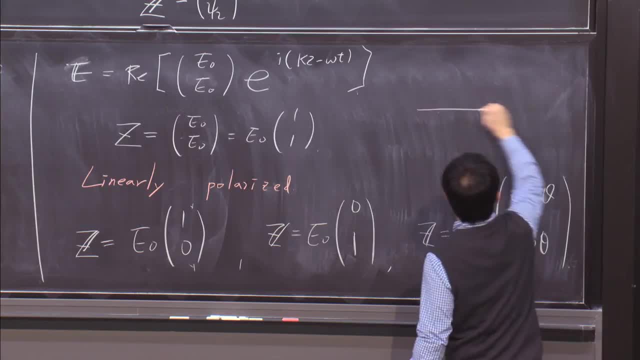 theta. What does that mean? This means that when I plot the locus on the xy plane, I'm going to have a straight line still, But now the angle between this line and the x is going to be theta. OK, So all those examples. you can see that in the first case. 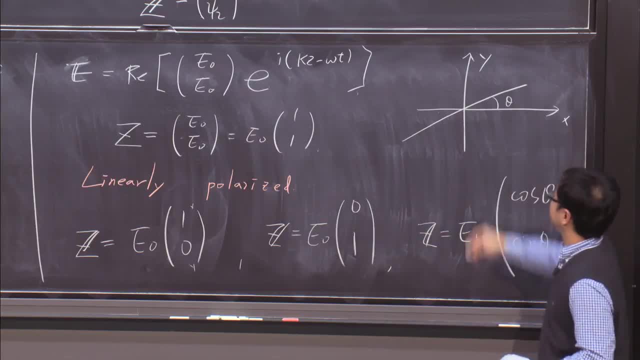 the oscillation is in the x direction, And in the second case the oscillation is in the y direction, And then in the third case it can be in an arbitrary line, theta angle away from the x-axis Right. So all those things are linearly polarized. 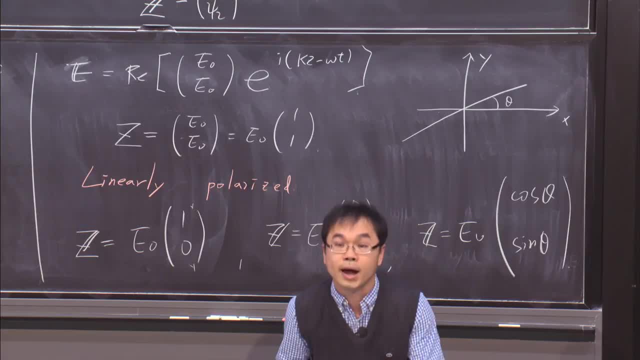 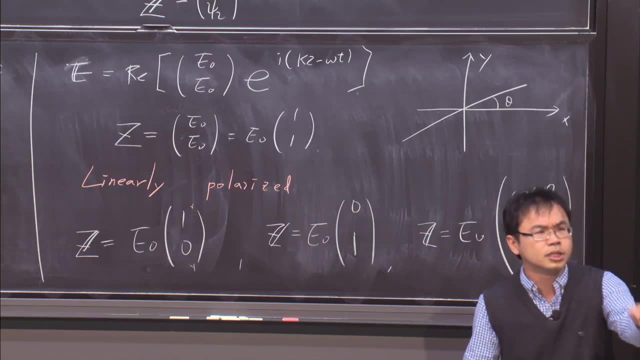 OK, So there's nothing to surprise you, Right? So that's actually what we have been talking about, And you can say that. oh, Professor Li, you were just not doing a very good job. You didn't rotate the axis, right. 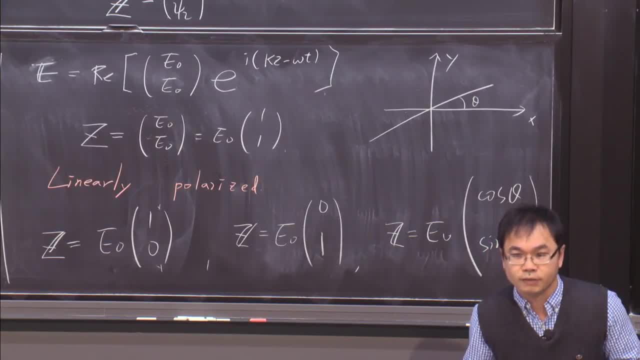 Right, So that all the electric field is in the x direction Right. So in principle, for the discussion of the linearly polarized wave, you can do a good job by rotating your axis so that you only have one component in the x direction. 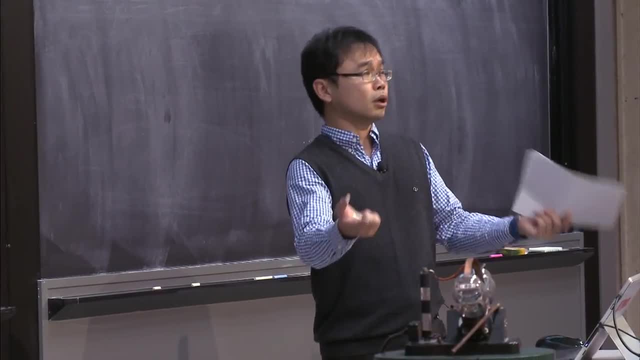 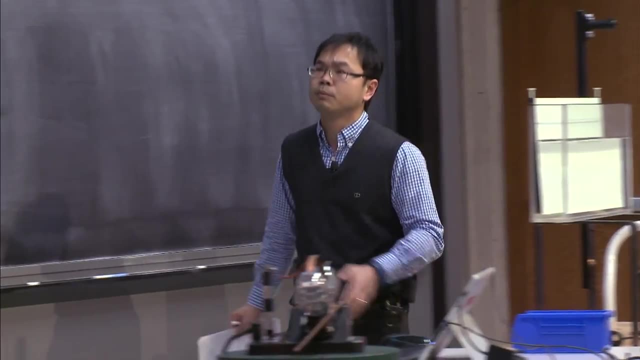 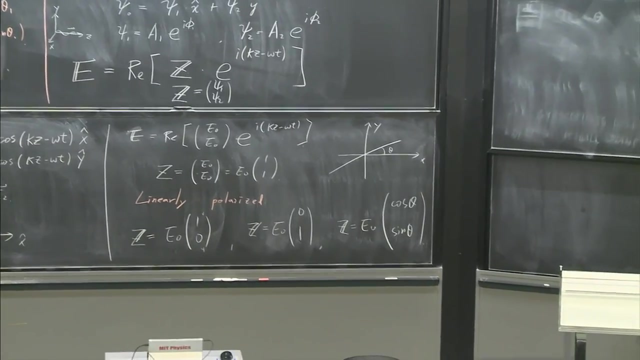 OK. So I say OK, yes, I agree, But this is useful discussion, Right? OK, All right, So now maybe you're bored. They have no phase difference, Right? So how about we introduce some phase difference and see what will happen? 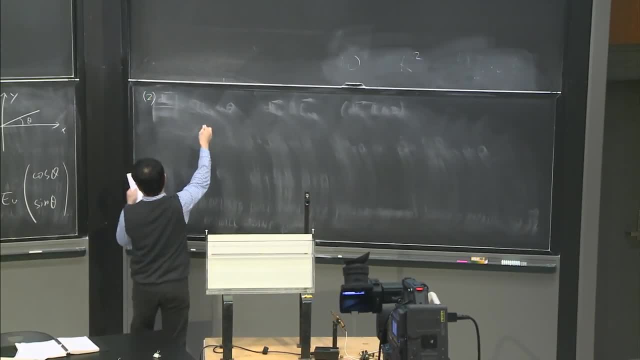 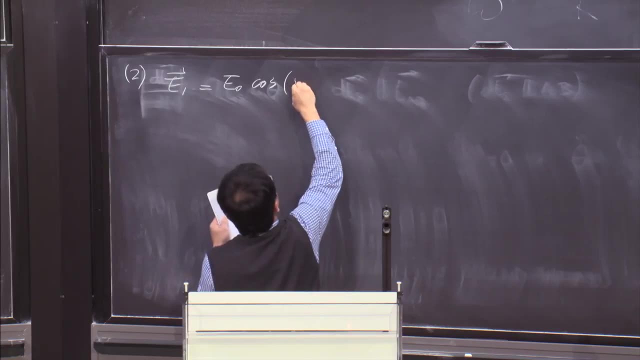 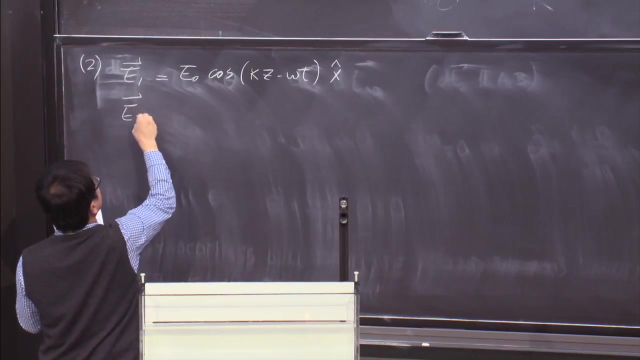 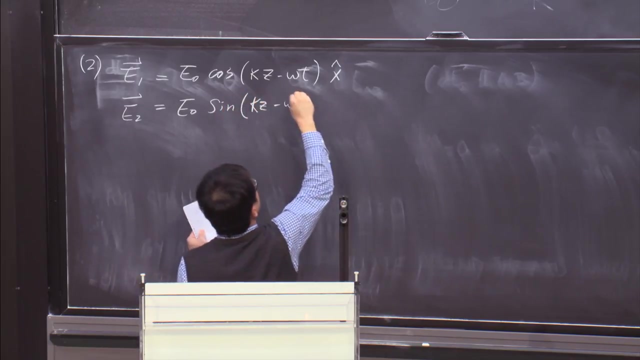 OK. So now, if I consider the second situation I have, E1 is equal to E1.. E1 is equal to 0 cosine kz minus omega t in the x direction. Now I consider E2.. This will be E0 sine kz minus omega t in the y direction. 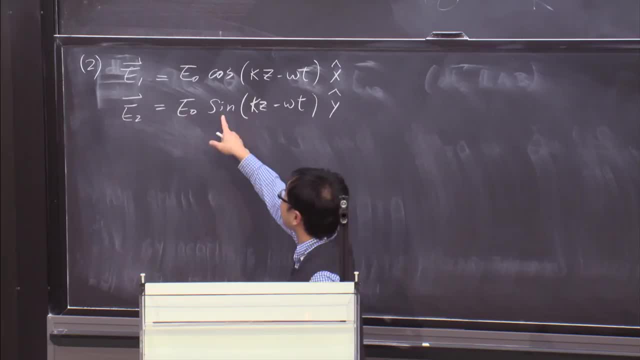 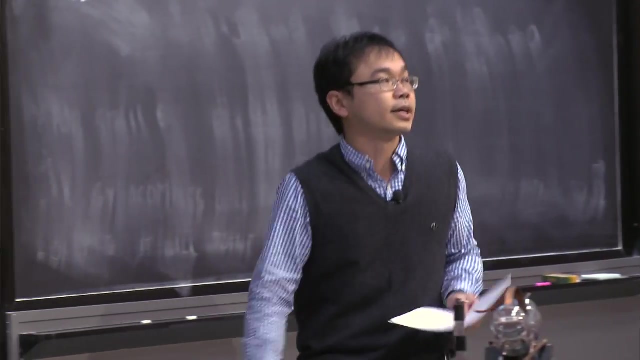 OK, I hope you can see it And you can see that now they reach the x component and the y component And you can feel they reach maxima at different time because of the phase difference. Right, How big is the phase difference? 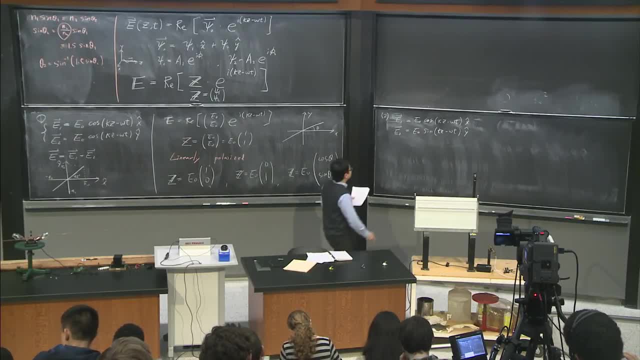 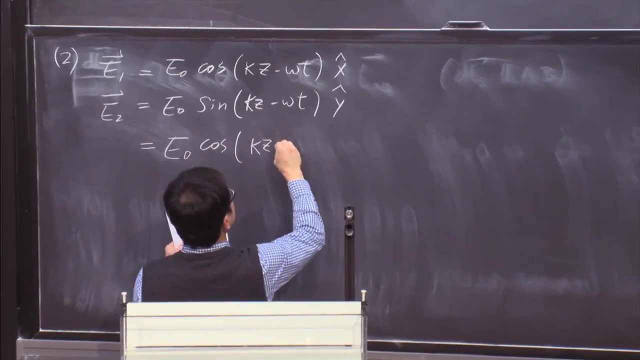 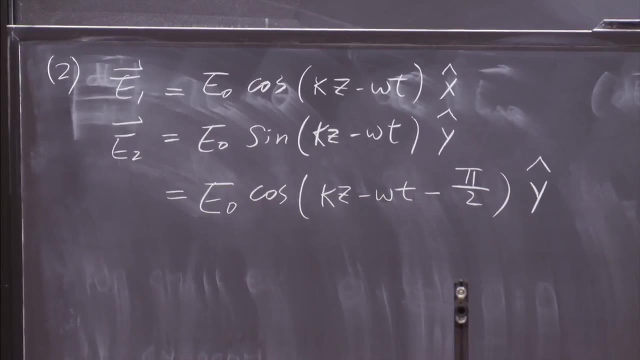 Can somebody actually remind me, Yeah, Pi over 2.. Very good, All right. So this I can write it down as E0 cosine kz minus omega t, minus pi over 2,, as you actually already figured out, Right, And then I can actually also again: 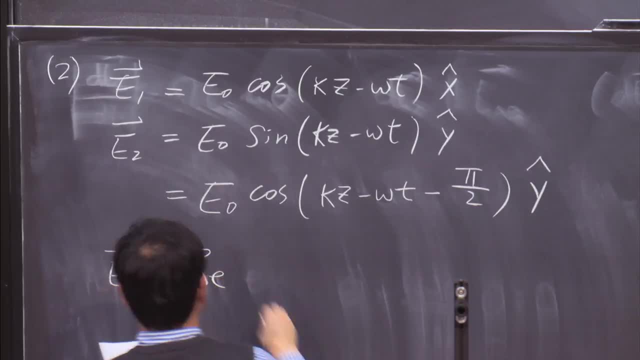 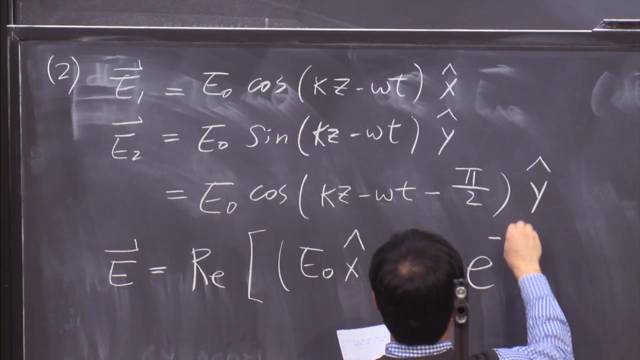 write it in the language I like, the matrix format And I can write it down already Before I achieve that. I can write it as a real part of E0 in the x direction plus E0 exponential, minus i pi over 2.. 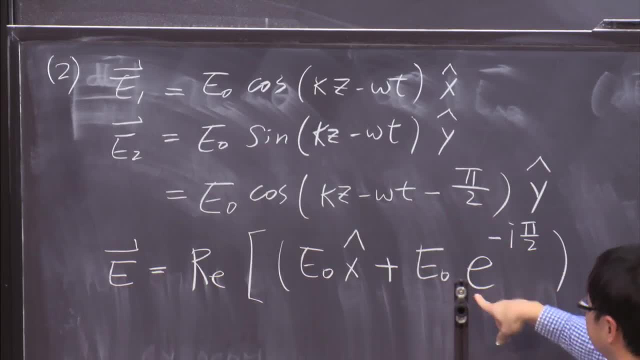 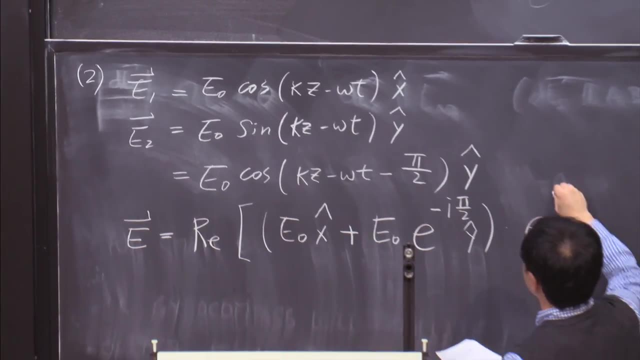 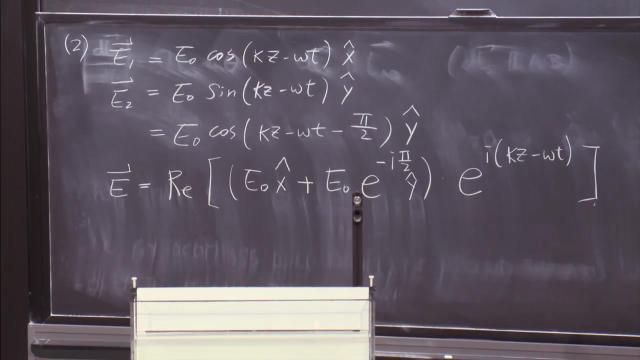 Right, Because this minus pi over 2 sign I can write for the y direction. OK, And all those things are multiplied by exponential i kz minus omega t. Right, Both of them are actually oscillating at the same omega angular frequency. 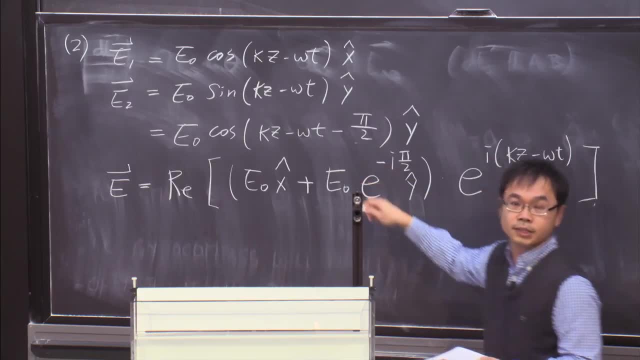 OK, And you can see that now I can collect this phase difference back into a complex factor here. exponential minus i pi over 2.. OK, And this is minus i. exponential minus i pi over 2 is actually just minus i Right. 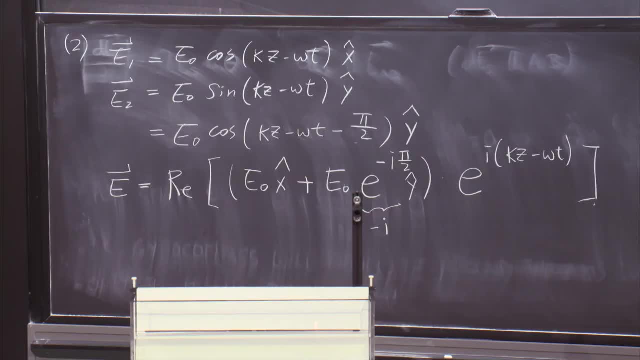 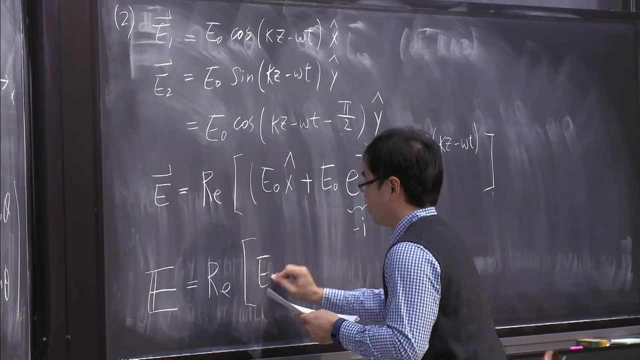 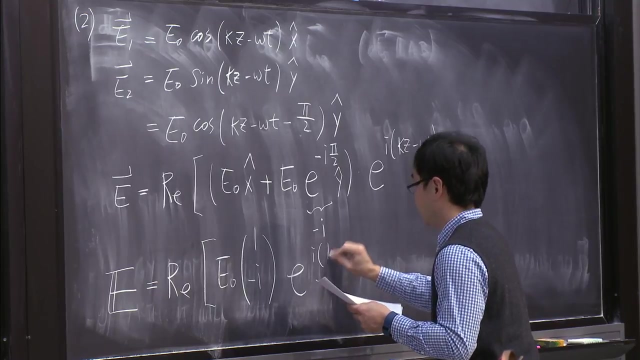 Because exponential. yeah, so basically you can figure out that it's actually just minus i, Right, OK, So then I can write down my expression for the E matrix. This will look like real part E0.. So 1 minus i, exponential, i kz minus omega t. 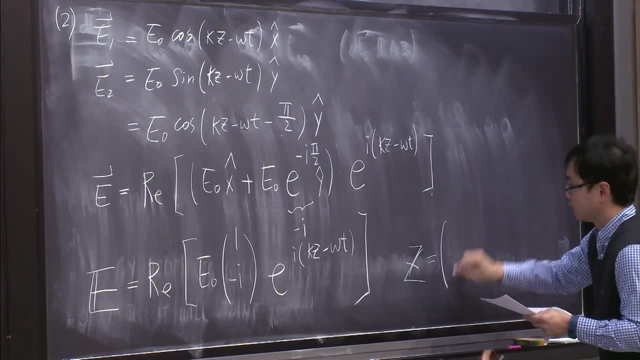 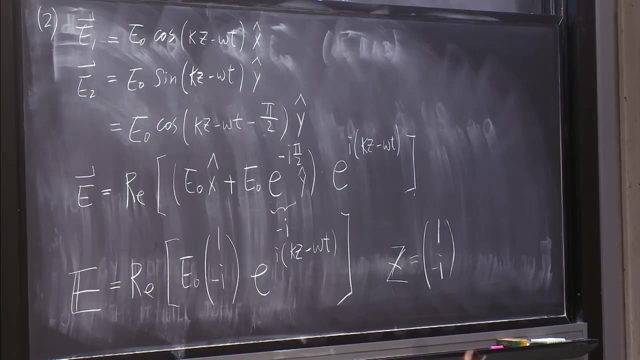 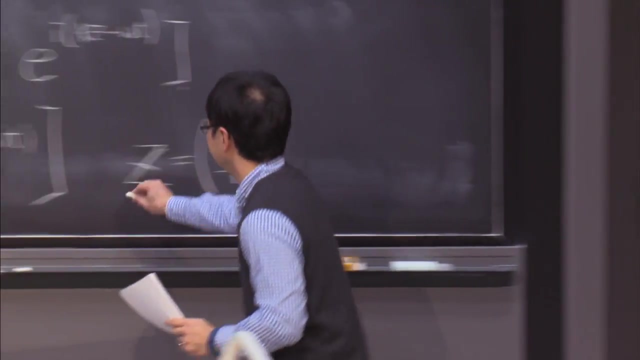 And in this case, z vector will be 1 minus i in the language which I introduced today. OK, Everybody is following. Am I going too fast? OK, Thank you. Thank you for the feedback. OK, So now I'm going to do the same thing. 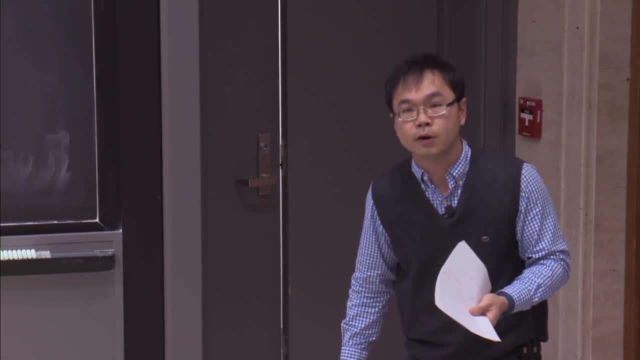 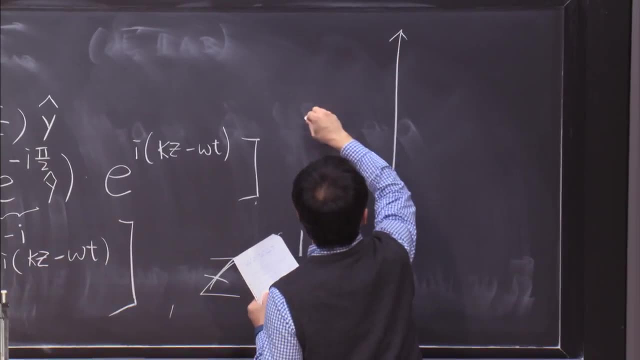 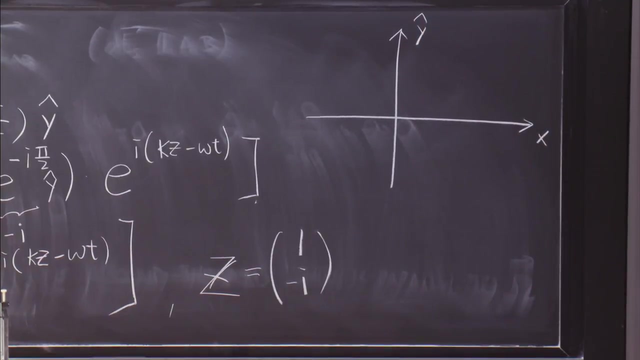 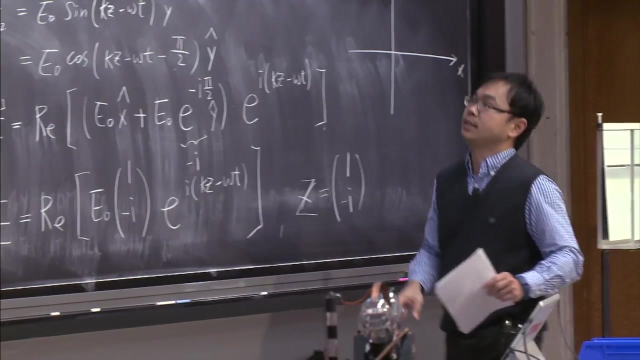 to plot the locus of the electric field as a function of time on the xy plane. OK, So now you can see that it's pretty interesting. So if I have a cosine and sine, OK, I assume that t is equal to 0, z is equal to 0,. 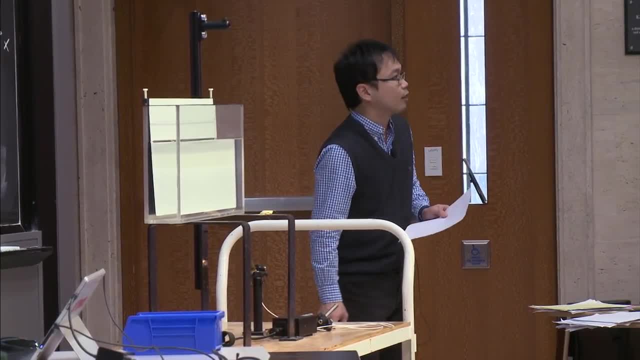 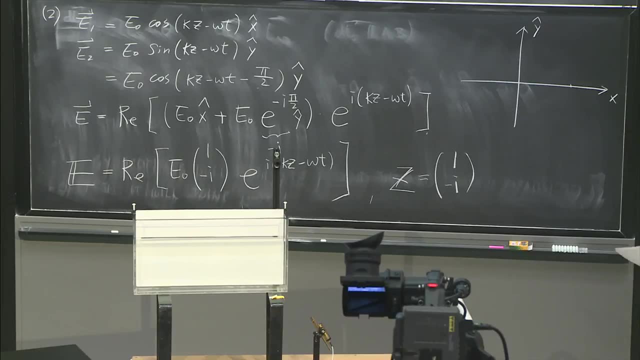 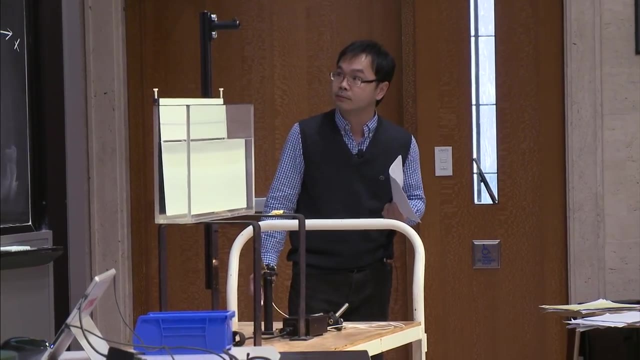 then I will only have electric field in the x direction, Right? So this is actually when t is equal to 0. All right, And if I increase time, I fix the z to be equal to 0. OK, If I increase the time? OK. 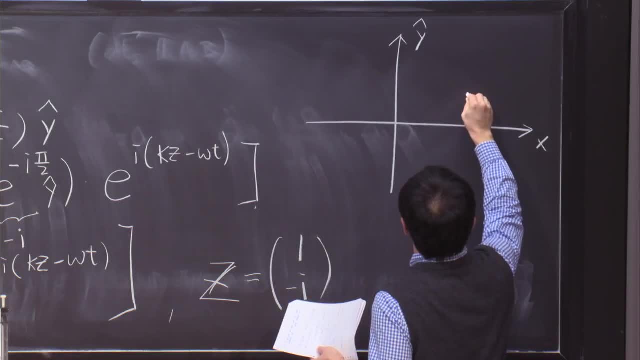 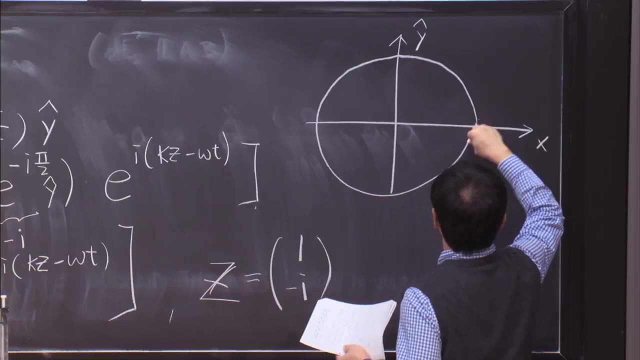 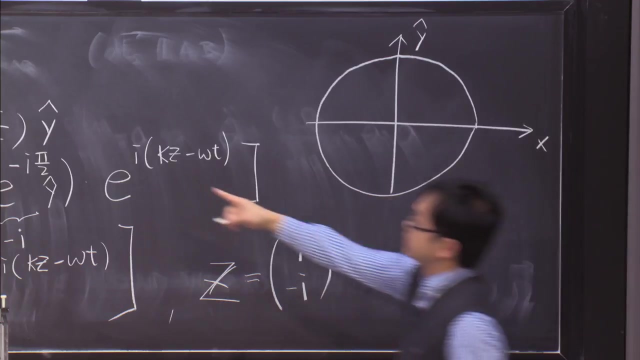 So this locus is going to do an interesting thing. It's going to be rotating until it finishes one period. OK, Why is that happening? Because what I am plotting is actually the locus of the electric field, Right, And you can see that if I set z equal to 0, OK, 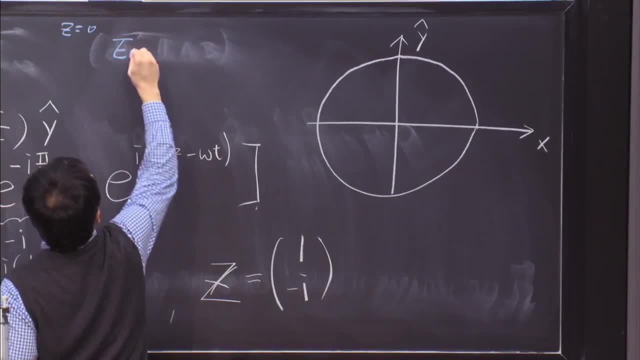 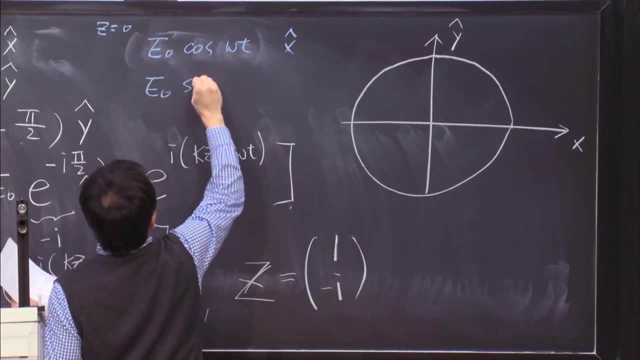 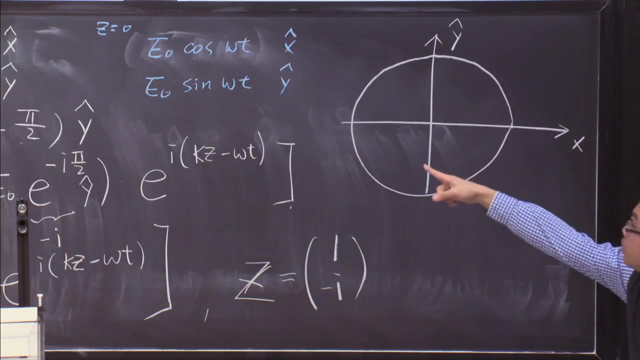 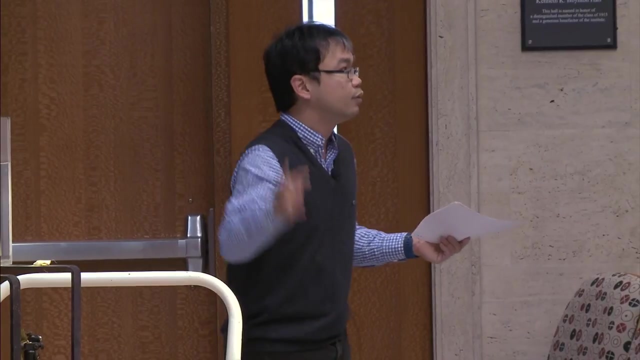 when z is equal to 0,. this will give you E0 cosine omega t in the x direction and E0 sine omega t in the y direction. OK, So E0 cosine omega t, E0 sine omega t. wow, this reminds you about the previous discussion, right? 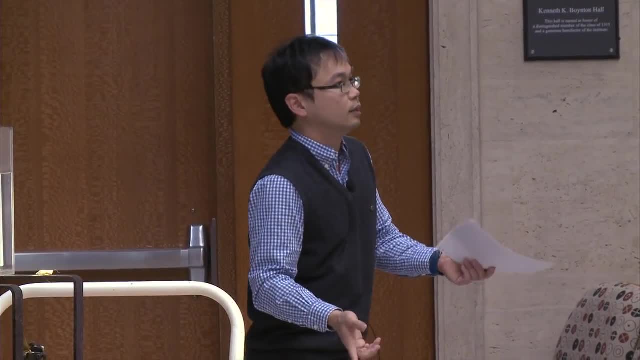 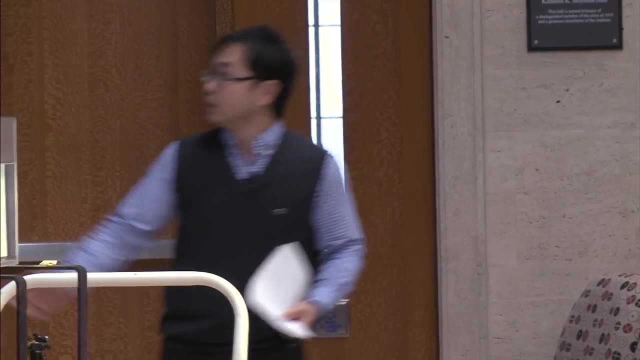 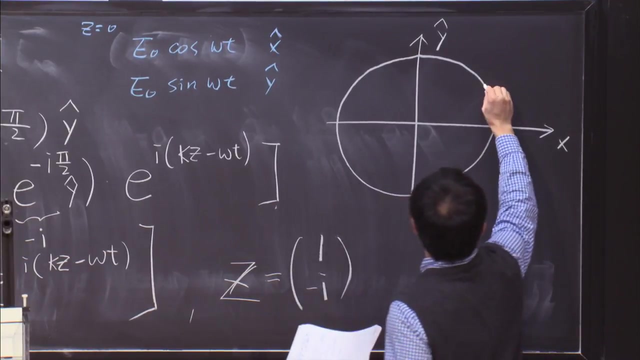 If you have a cosine and a sine, they work together in a different direction. That's going to get you a circle, Right. So that's actually why in this locus you see a circle And it's actually rotating in the counterclockwise direction. 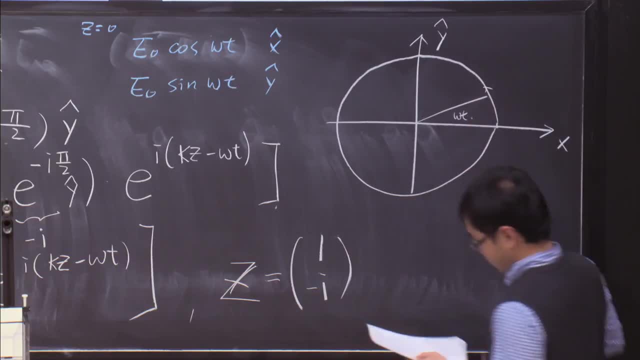 OK, And the speed of the rotation is related to the omega t And OK. So if you look at increase the time, then this point is going to be going in the counterclockwise direction. OK, And you may be super surprised. 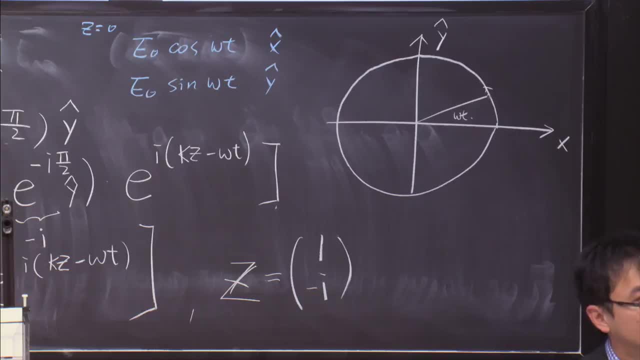 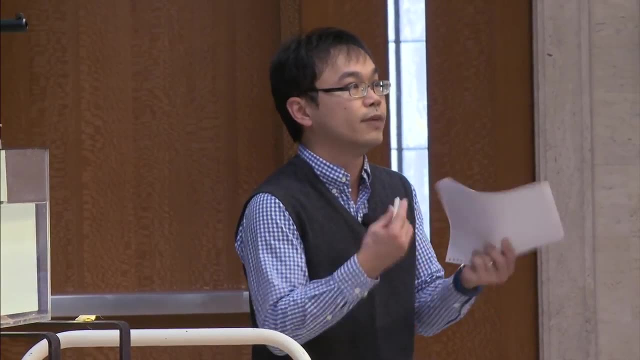 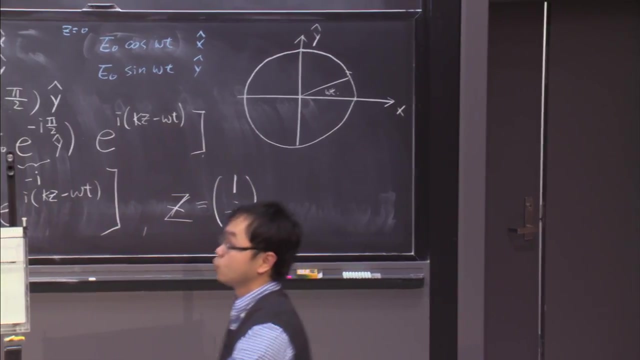 Because what I have been doing is to add two linearly polarized waves together. The only thing which I always say, the magic I have been doing is to introduce a phase difference. OK, So instead of going up and down, up and down as a function of time, now it's actually doing rotation. 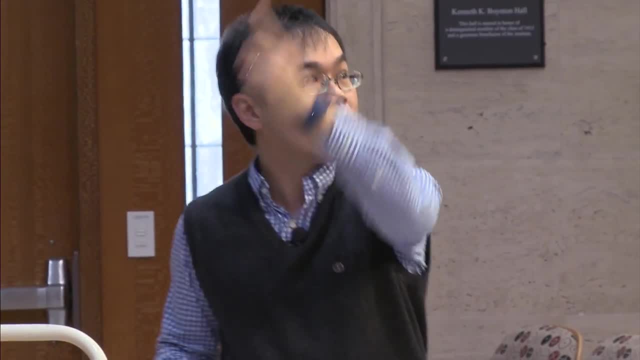 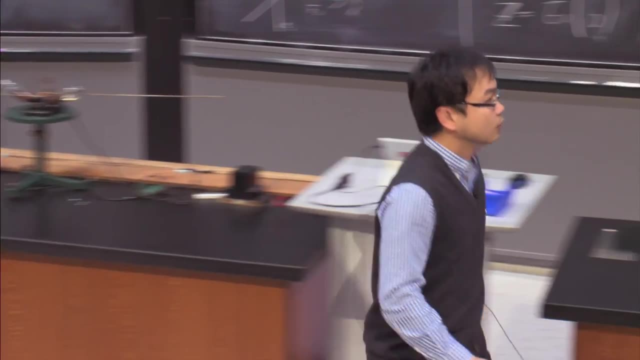 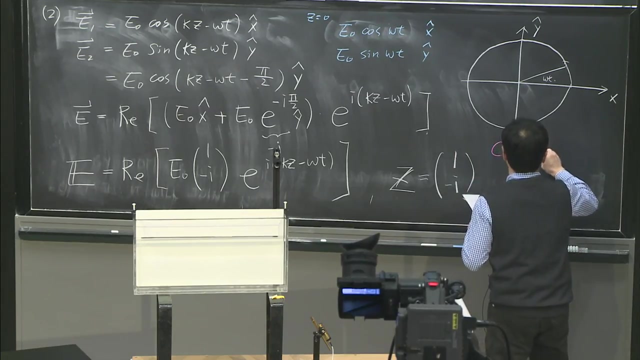 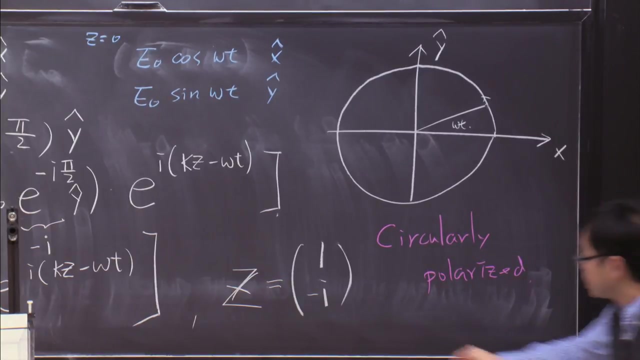 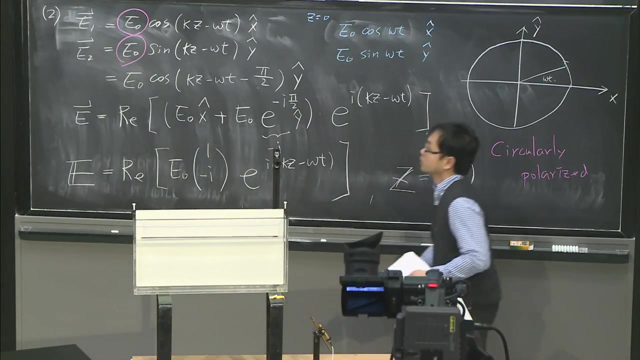 So what is going to happen is that, as a function of time, the direction of the electric field is going to rotate as a function of time. So we call this situation circularly polarized- OK, By the way, because of the initial two components. 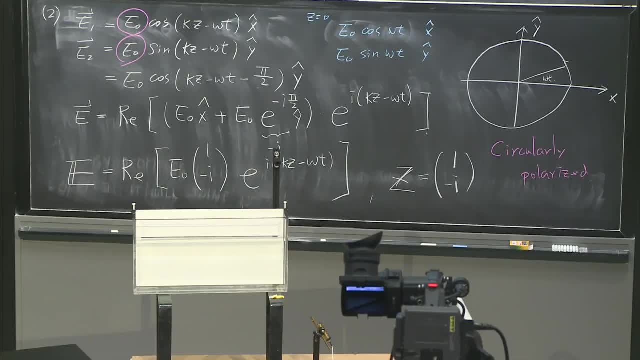 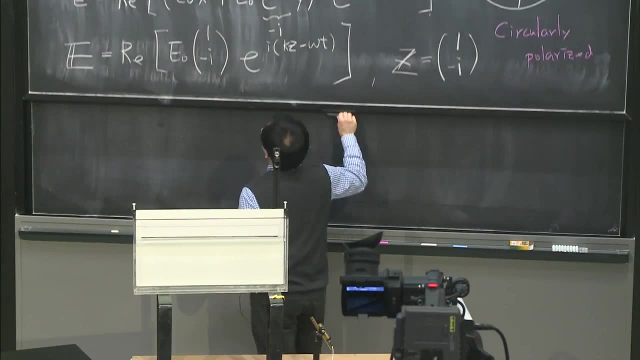 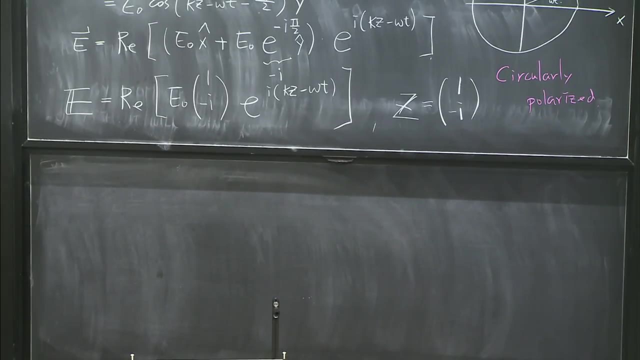 I put in, both of them have amplitude E0. Therefore it's circularly polarized Right. I can also try to do something different. For example, I can change the x direction. OK, So the third situation is that I can change the first x. 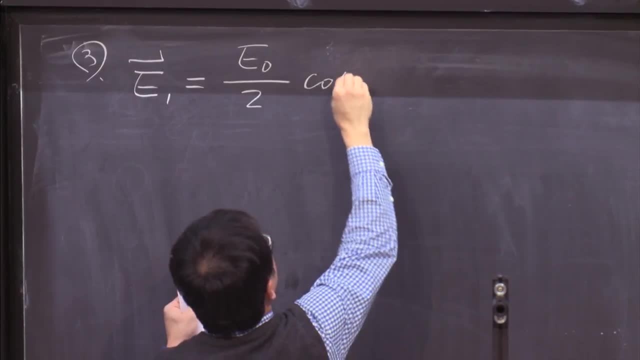 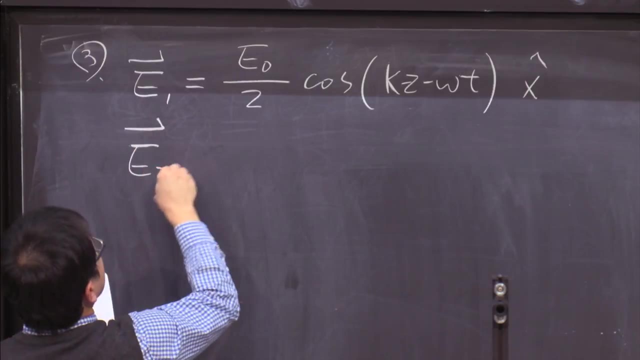 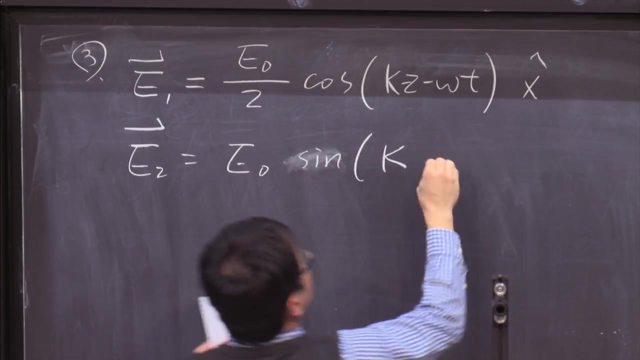 direction amplitude from E0 to E0 over 2.. Then what I'm going to get is something like this: The only thing which I change with respect to 2 is that I change the amplitude of the electric field in the x direction by a factor of 2.. 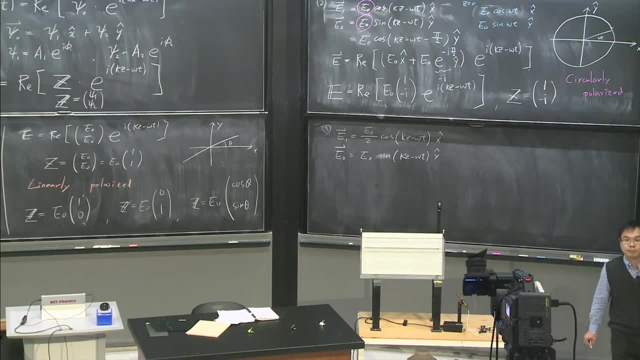 OK, Can somebody actually tell me what is going to happen in this situation? What will happen to the locus? OK, Yeah, it's going to squish in right, So in the x direction. right, Yeah, that's right. 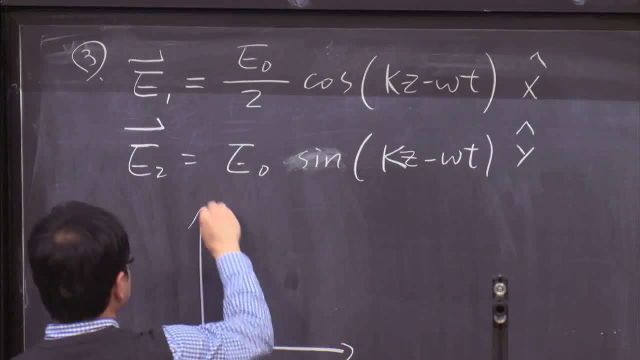 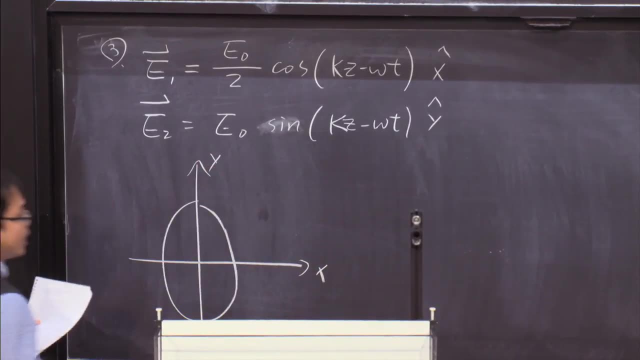 Very good. So what I'm going to get is that, instead of a circle, you get something like this: So this is the x direction and this is the y direction, And this will give you a maxima x equal to E0 over 2.. 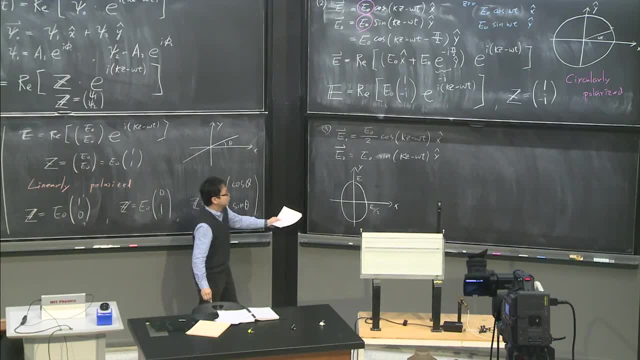 And of course the original amplitude in the y direction didn't change, And that gives you a maxima value of E0. So this becomes an elliptically polarized wave. OK, So in this kind of situation it's called elliptically polarized. 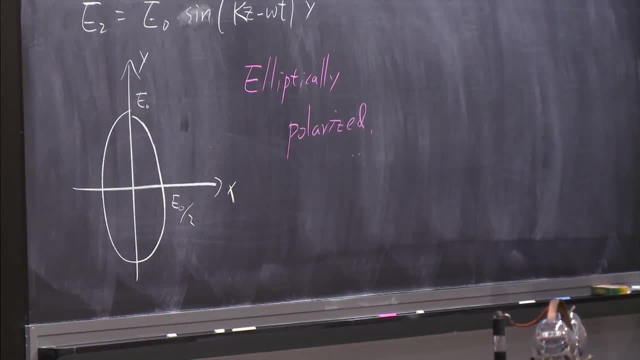 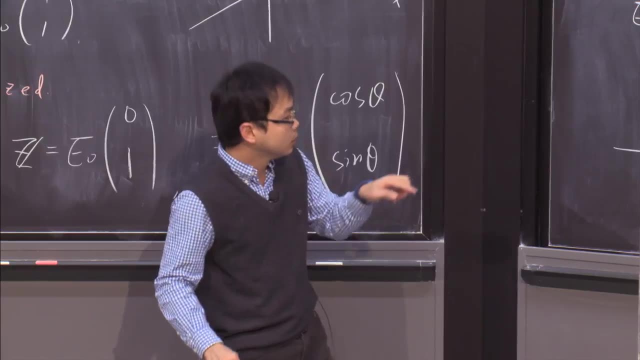 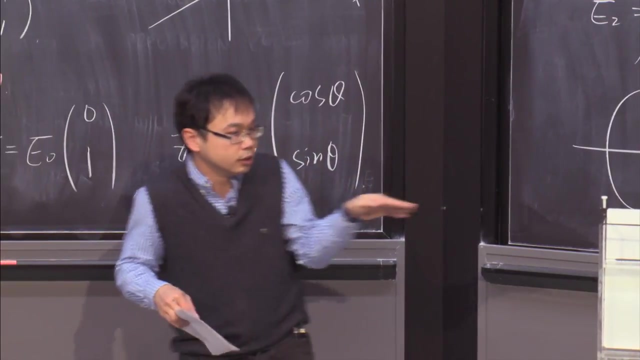 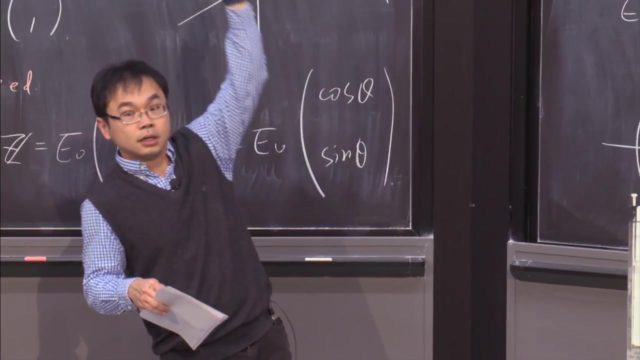 How do we actually visualize this situation? OK, So that means, as in the beginning, when the electric field is aligned with the x-axis, it's pointing in the x-axis it has a shorter length And when it rotates, rotates as a function of time to the y-axis. 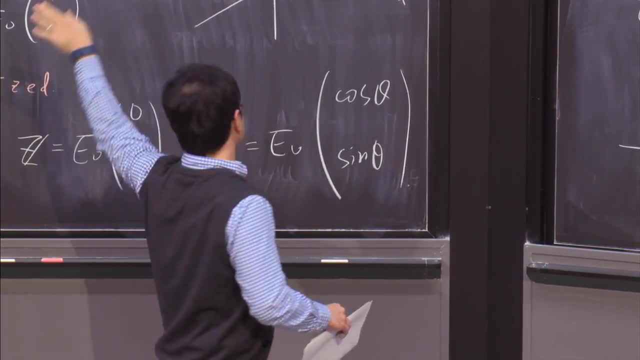 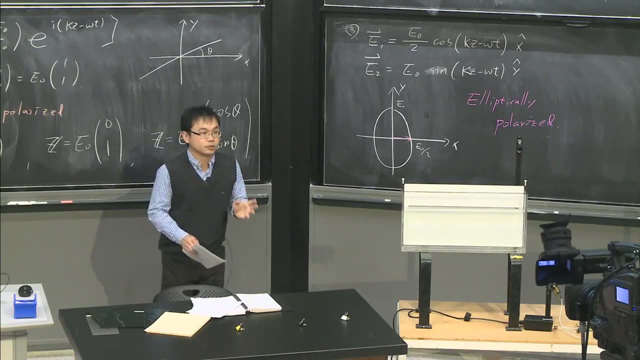 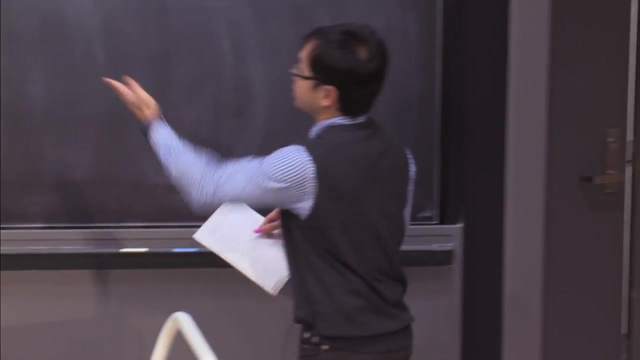 the amplitude becomes bigger, And it gets smaller again, And it increases again, It becomes bigger. OK, So you can see the amplitude is actually increasing as a function of time. When you have this kind of situation, they have different amplitude, although they 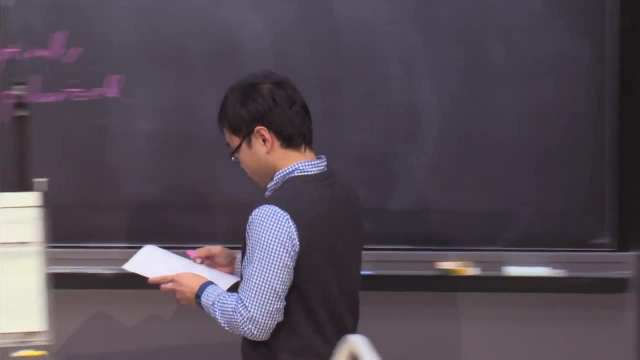 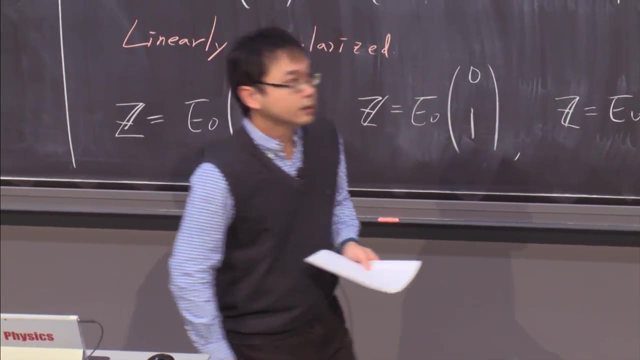 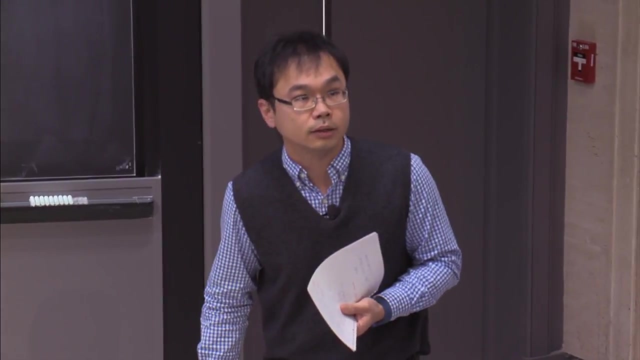 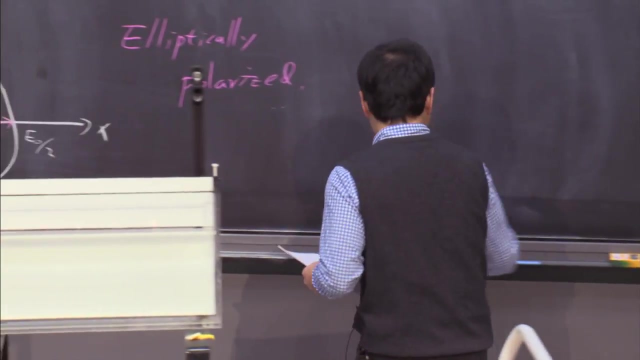 have a fixed phase difference of pi over 2.. OK, Any questions so far? OK, So if you noticed that there's actually another way to produce elliptically polarized wave, OK, What we could do is that, instead of changing the phase, 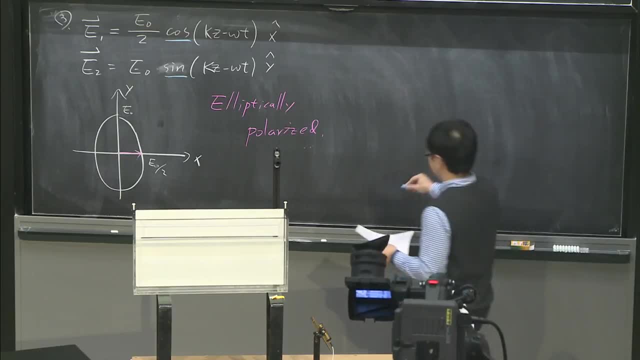 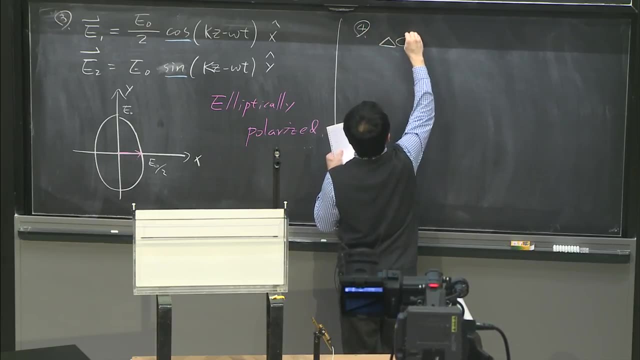 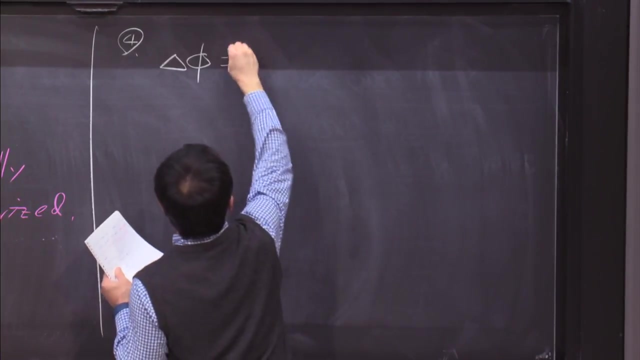 by a factor of pi over 2, we can change the phase difference. The phase difference can be delta. phi, which is the phase difference, can be a different value, arbitrary value, So 2 pi over 2 or 3 pi over 2.. 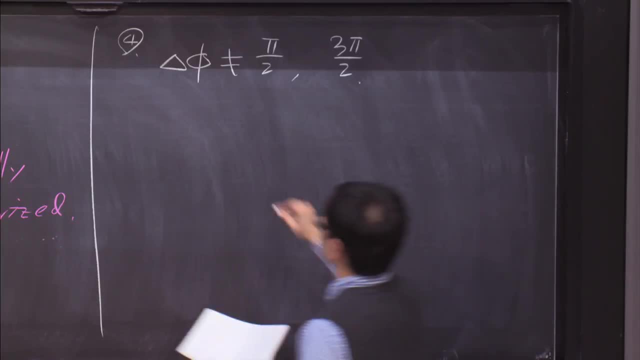 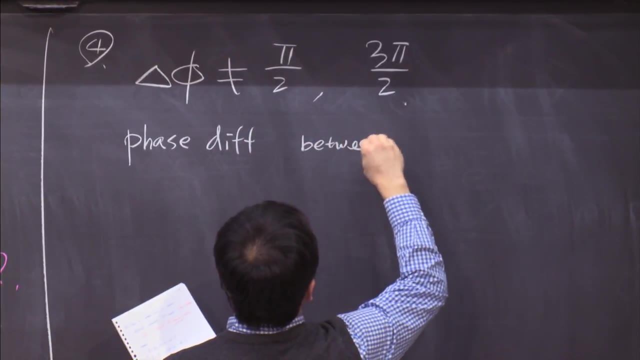 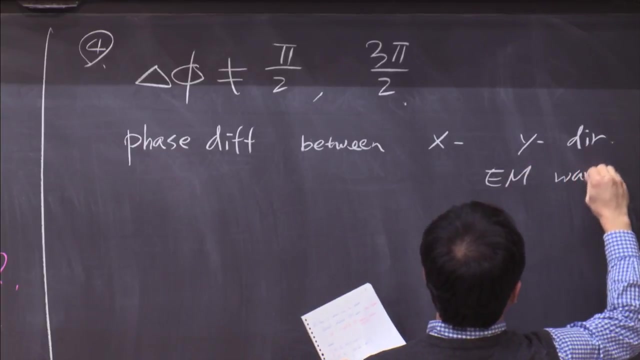 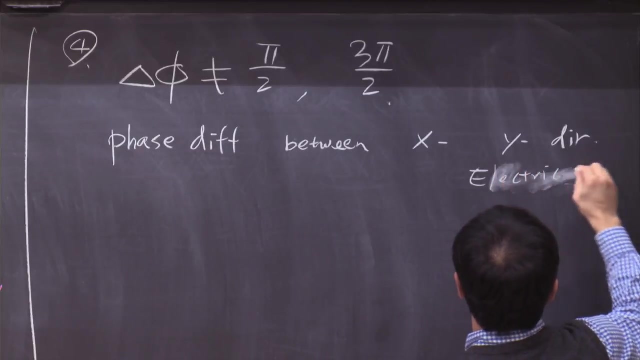 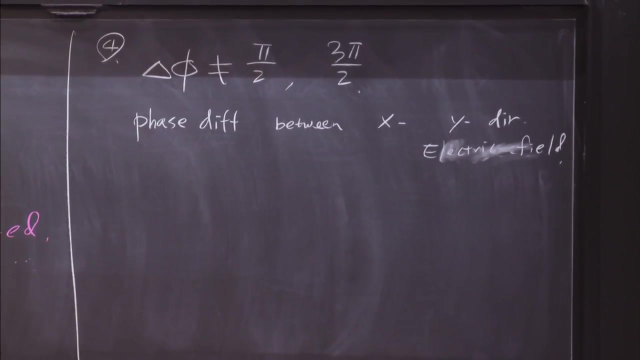 If the delta phi is between the, which is the phase difference between x and the y direction. EM waves: OK. If the electric field OK. If the phase difference is not pi over 2 or not 3 pi over 2,. 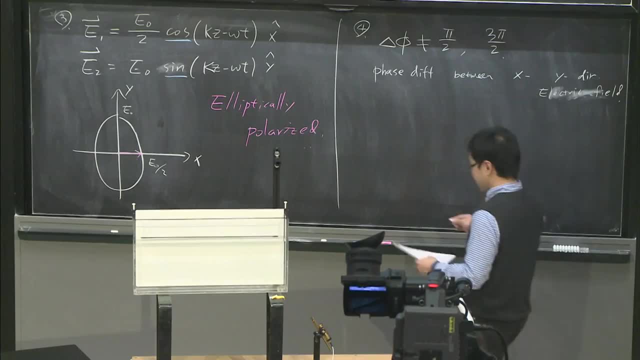 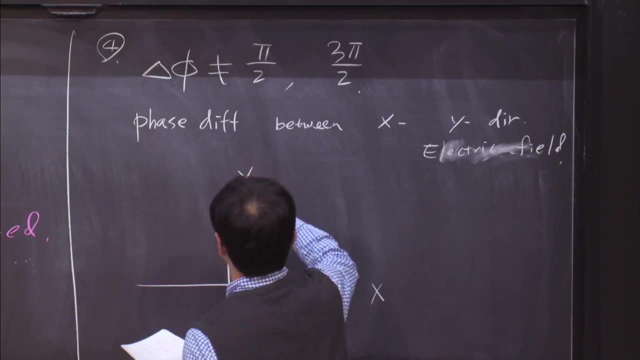 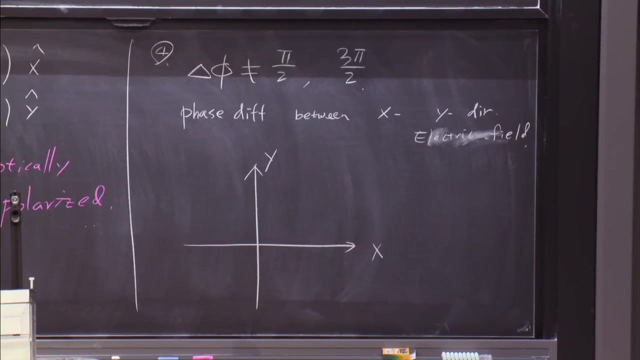 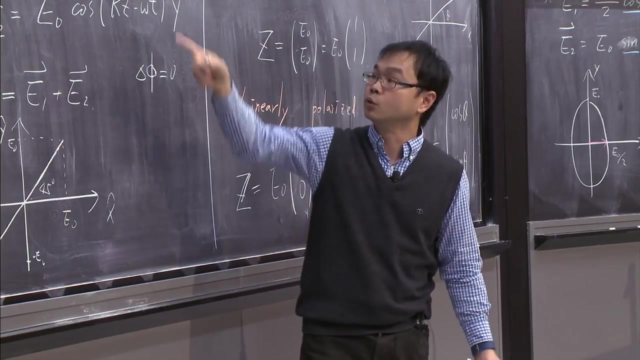 then you can also create an elliptically polarized wave. OK, So that's actually start from the original figure which, when we actually discuss situation number one, OK, I have delta phi, The phase difference equal to 0. Right, When that happen, you have a linearly polarized wave. 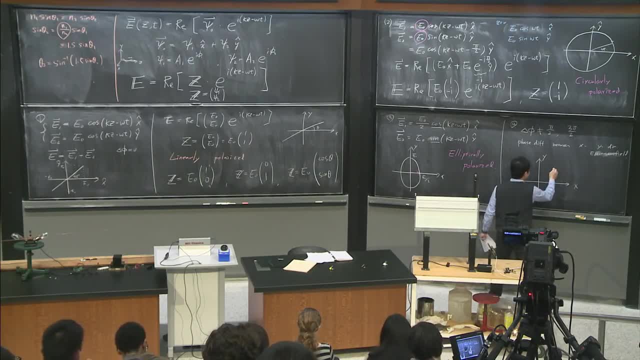 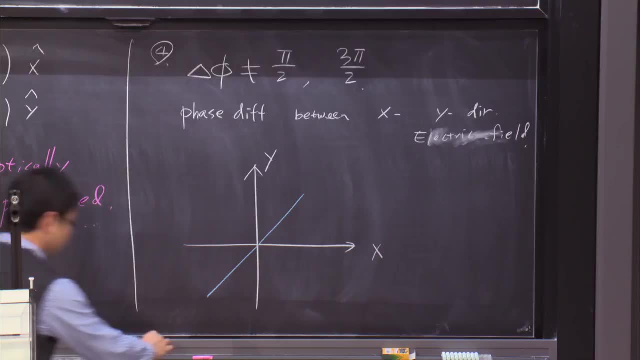 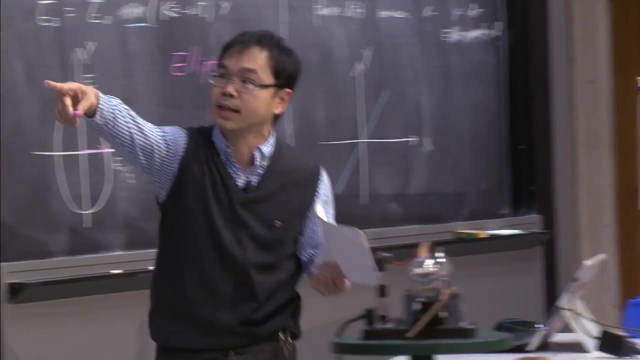 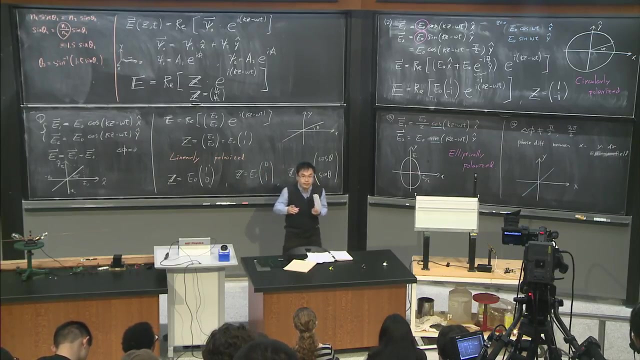 Right. Basically, what you are going to get is a line in this two-dimensional space If I increase. So now I slightly delayed. OK, If I slightly delay the electric field in the y direction. OK, So if I slightly delay electric field in the y direction. 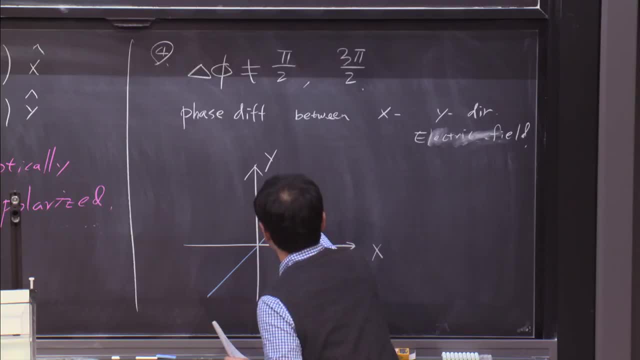 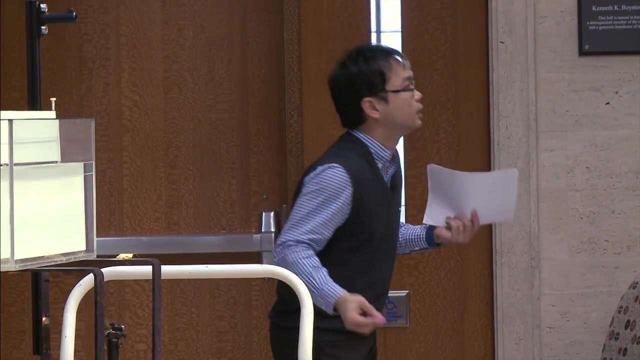 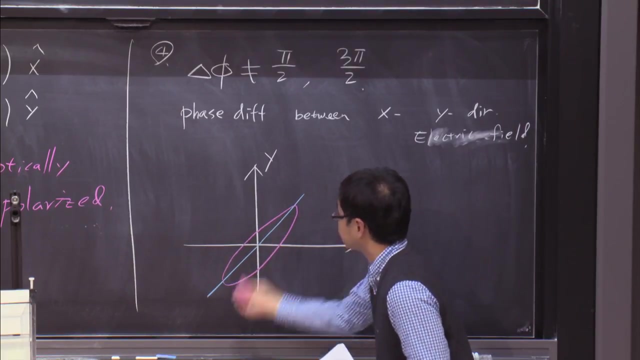 so that delta phi now is greater than 1, what is going to happen is that it's going to look like this: This means that they will not reach maxima really because of the phase difference, And you will see that originally, when there were no phase difference, you 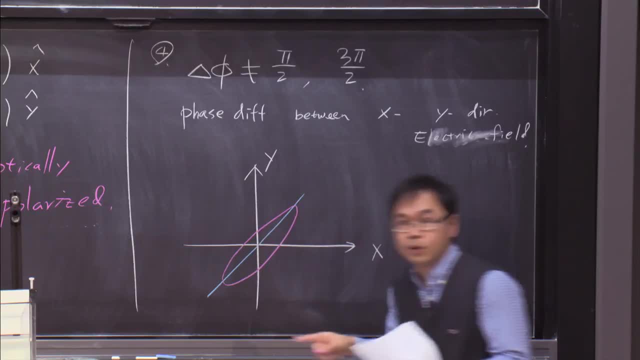 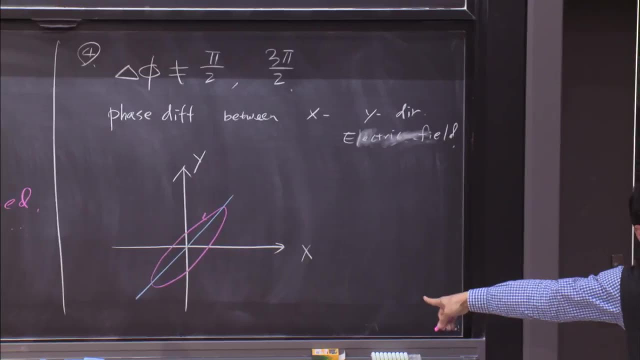 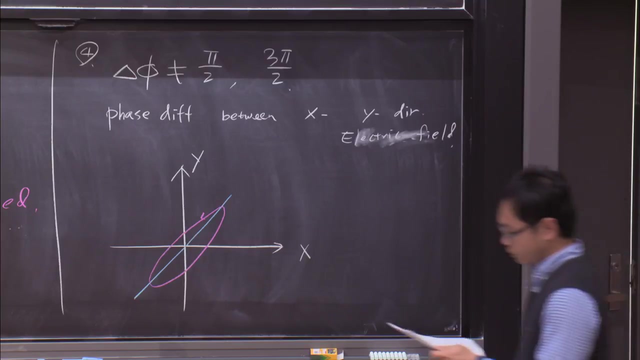 will be oscillating back and forth in this blue line. When you increase the delta phi slightly, then you are going to get also an elliptical shape. OK, But now it's tilted with some degree, which is 45 degree in this case. 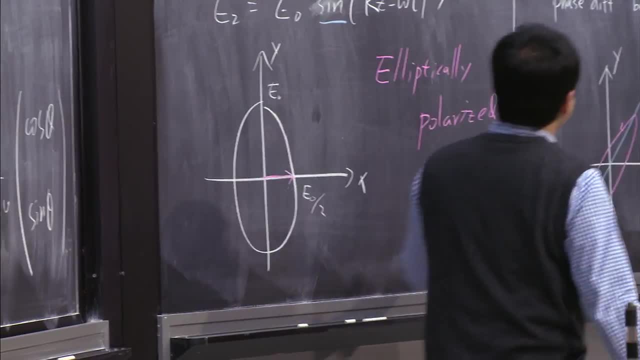 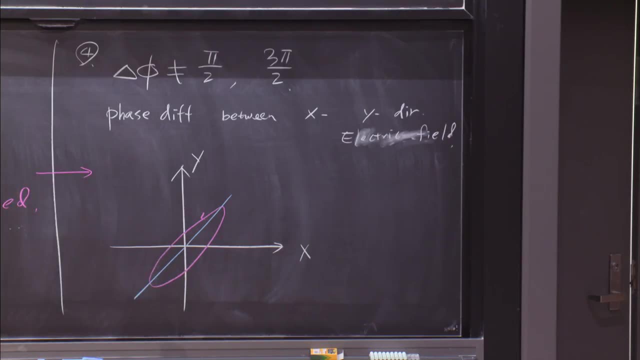 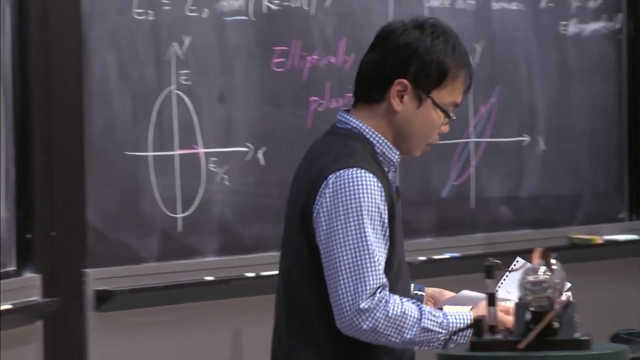 OK, So therefore you can see that now I can also create- This is also- an elliptically polarized wave. I can also create elliptically polarized wave by adding two components, which they have some slight phase difference. OK, So that is actually how actually I can create something. 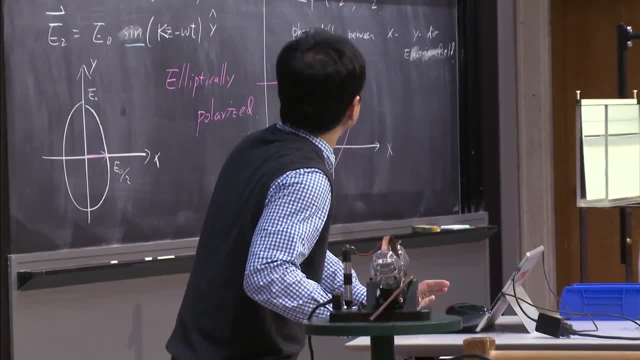 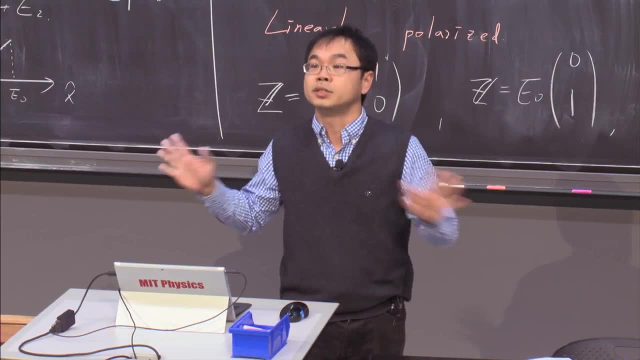 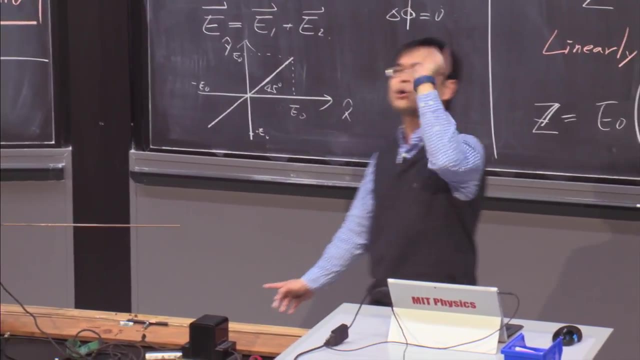 which is called circularly polarized or elliptically polarized. OK, Originally, before you come into this class, it may look really completely bizarre that, oh, OK, I can have electric field going up and down as a function of time. 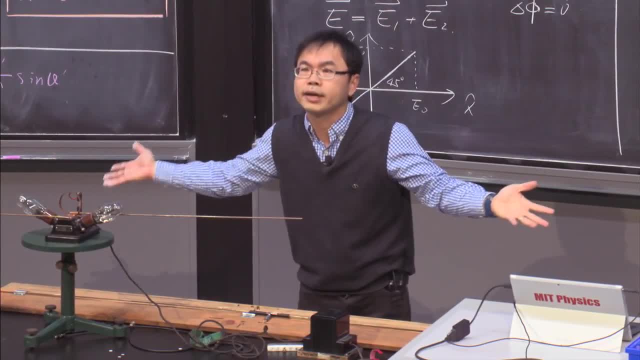 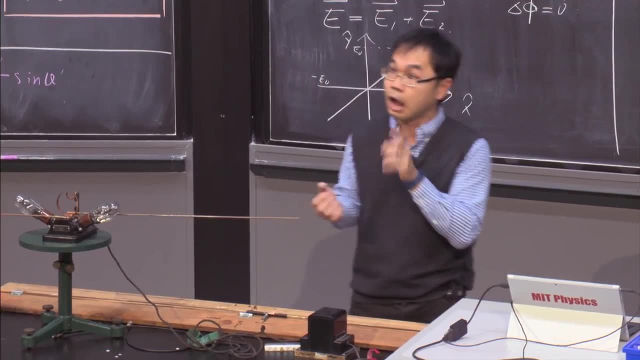 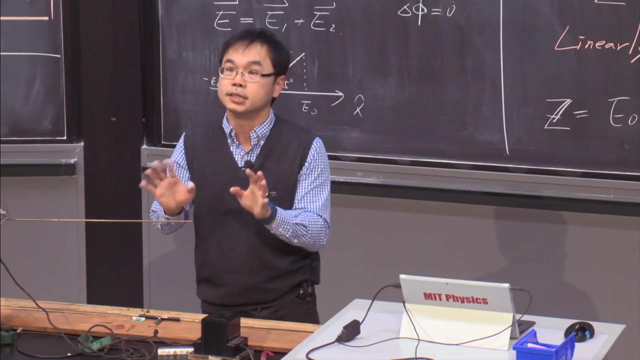 But how could I rotate this thing right? Looks really strange. How can I see this from the Maxwell's equation right? But now you get the idea. Basically, that's because I can now add two components. Both components individually are linearly polarized. 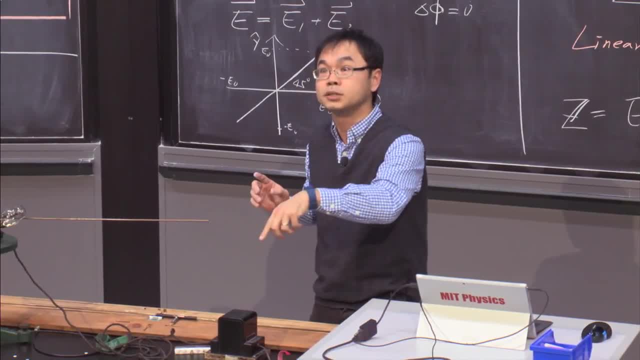 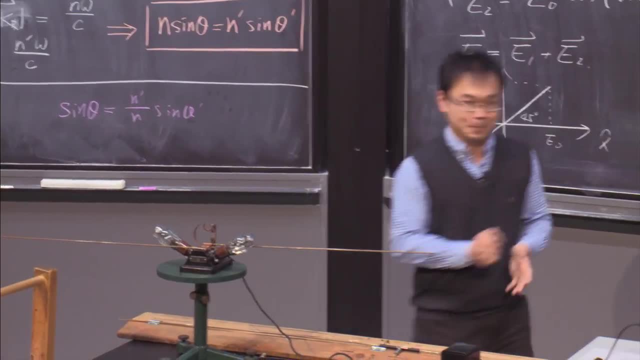 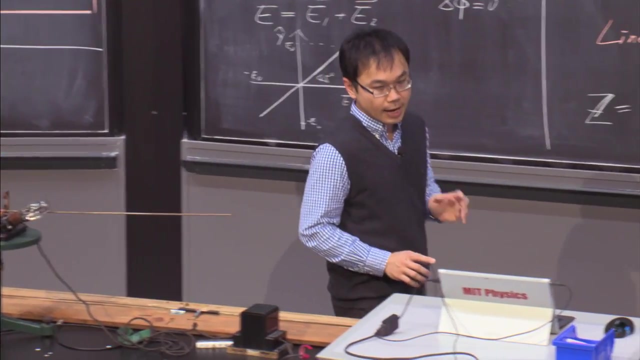 OK, But if I introduce a phase difference, then the superposition of these two components become something which is actually rotating as a function of time. That's pretty interesting, OK, So that's actually visualize all what we have learned so far. The first one is linearly polarized. 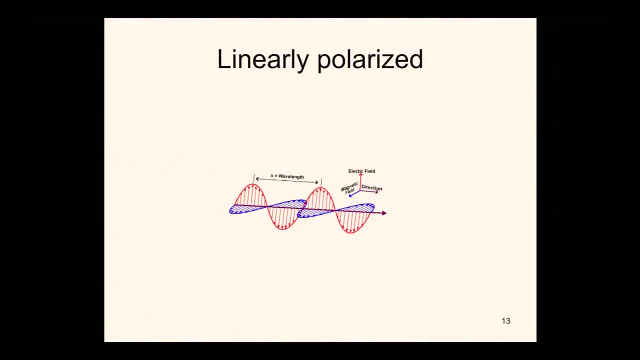 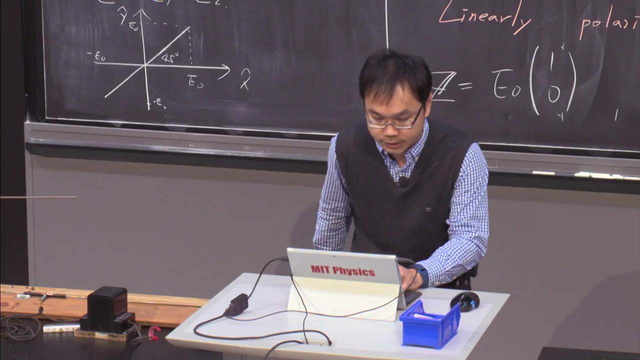 Actually it doesn't surprise you. That's actually the example which we have been using in the previous lectures And this is actually the situation of circularly polarized wave. So that's focused on the figure at z equal to 0.. 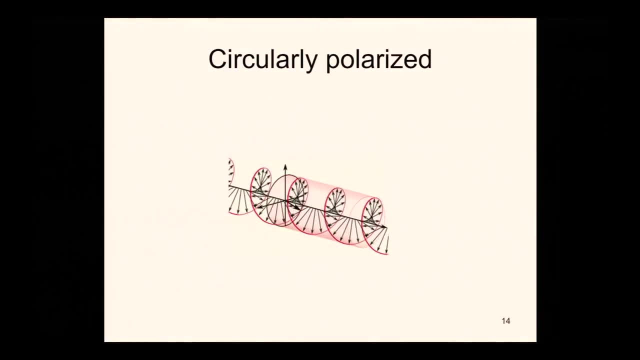 So you can see that in this case the direction of the electric field is actually rotating as a function of time And of course, as we actually discussed, if I can actually add two electric fields with different amplitude or introduce slightly different phase, then you 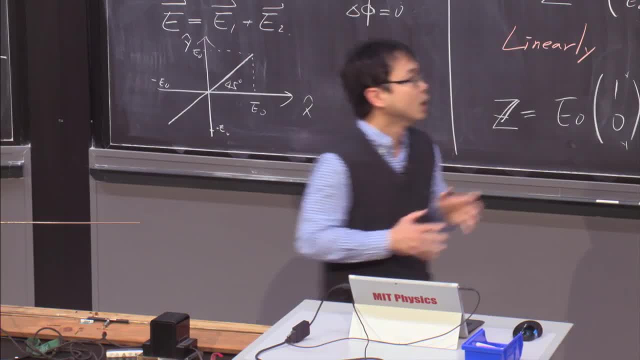 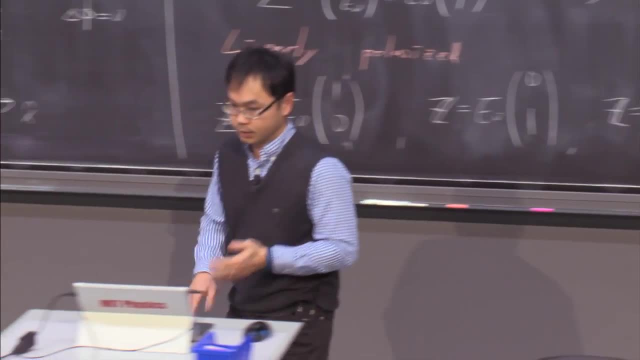 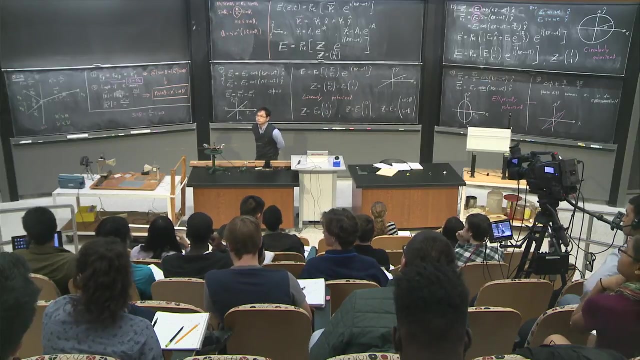 will see that not only the direction is changing, but also the amplitude is changing, And in this case we call it a ethically polarized wave. OK, Any questions? so far, Yes, So the magnitude of the wind is constant with time. now 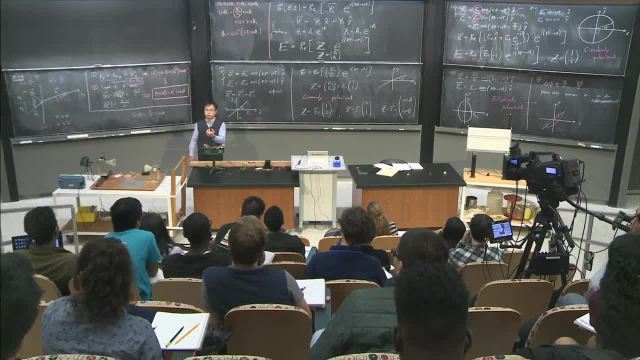 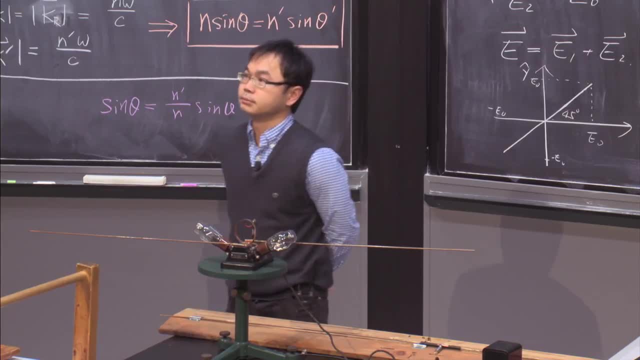 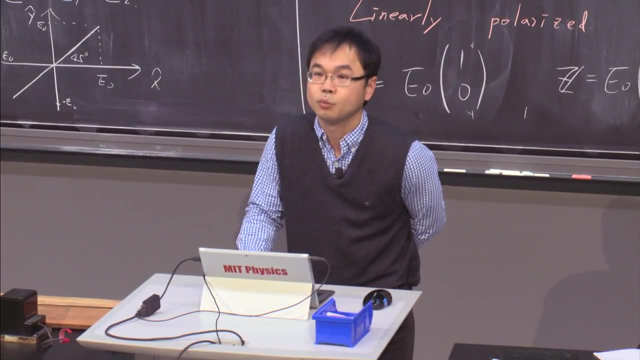 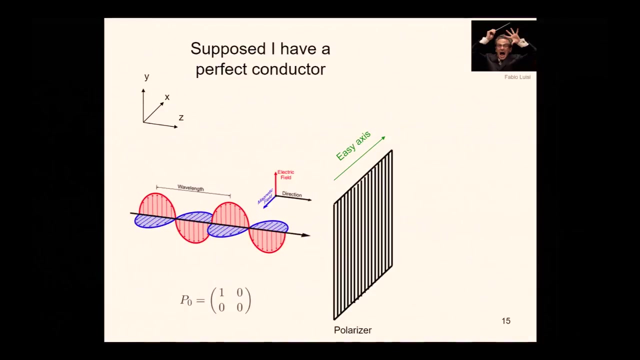 Yes, The magnitude is actually the yeah. So the magnitude, or say the intensity, is proportional to e, squared right. So it's actually a constant. So now let me add more excitement here. So now suppose I have a perfect conductor. 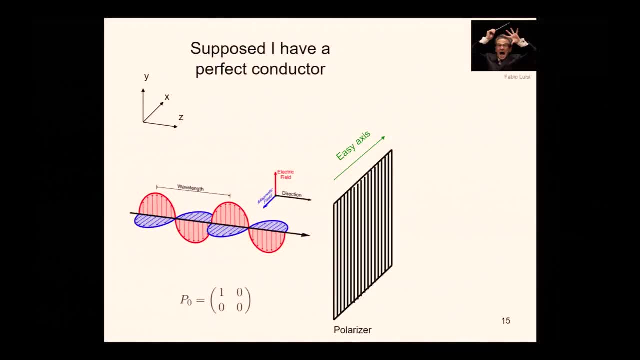 All right. So what I'm going to do is that I'm going to introduce some more excitement by shooting this linearly polarized wave through some material. OK, If I have a perfect conductor. OK, where all those strips? OK, I have only strips. 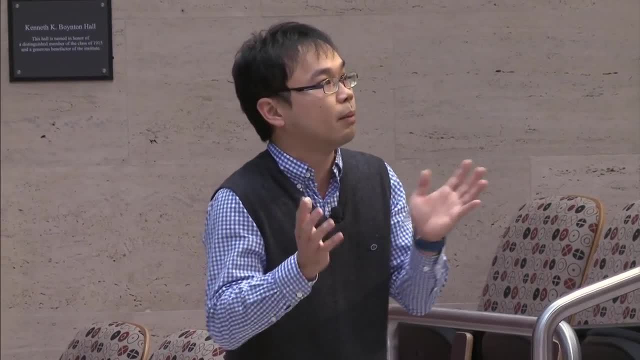 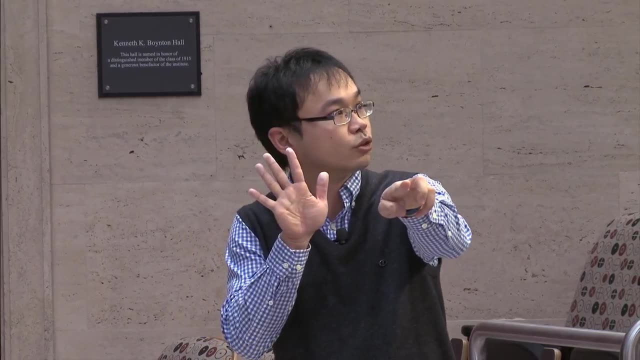 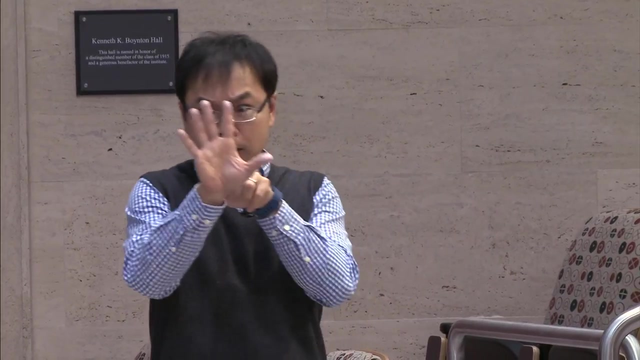 of perfect conductor instead of a plate. OK, We were talking about plate before right, And the lesson we learned is that the plate is going to refract the electromagnetic wave because the electrons on the plate is so busy it's trying to make sure. 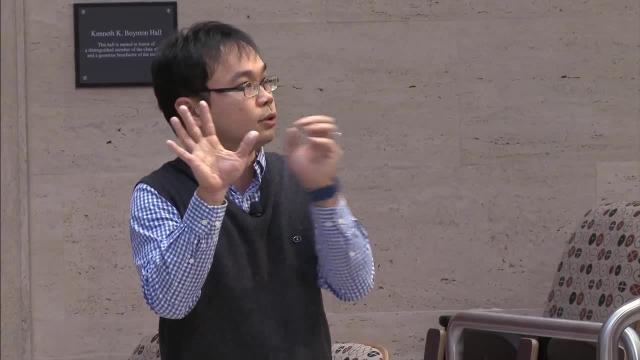 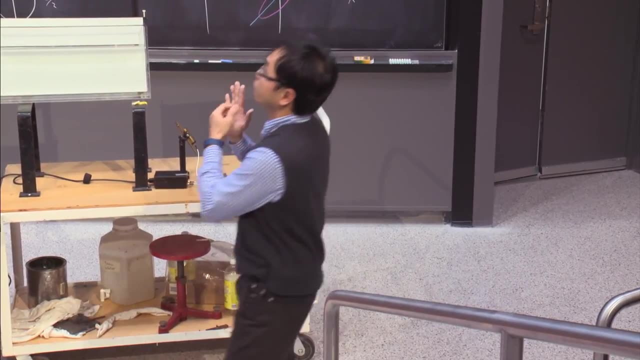 that the electric field in the surface of the plate is equal to zero, right? Because all those electrons are really moving around. so that makes sure the electric field is canceled And therefore it's going to refract the electromagnetic wave, OK. 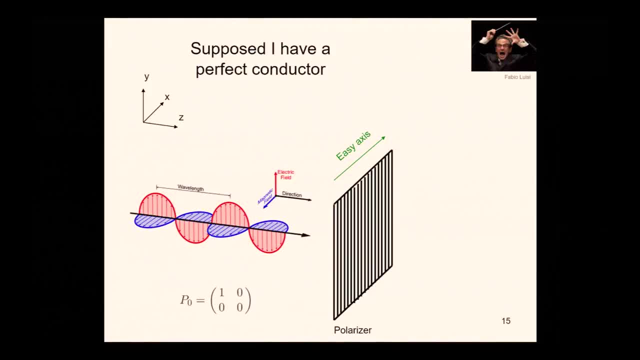 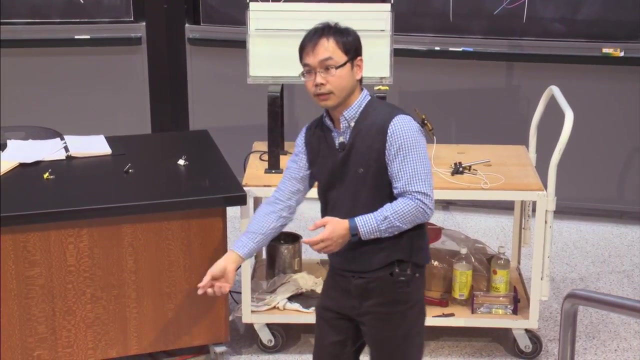 So how about I actually restrict the direction of the movement of the electron, so that it can only move in the oriental direction? OK, What is going to happen is that, in this case, the electric field is actually oscillating up and down. 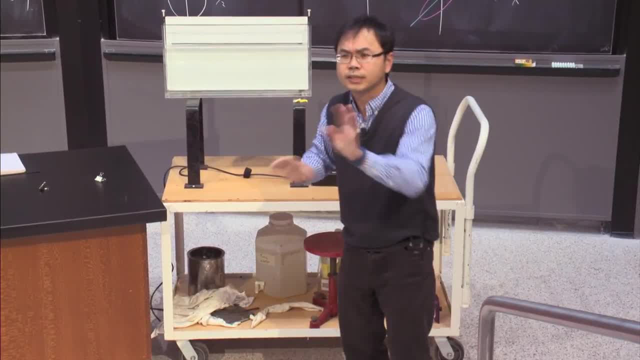 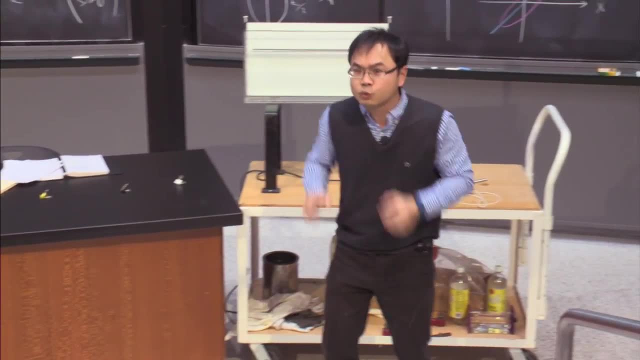 Right, And the electrons see this field And they will say no, no, no, This is not what we work. OK, This is actually now we are going to vote for, And I'm going to arrange ourselves to compensate that. 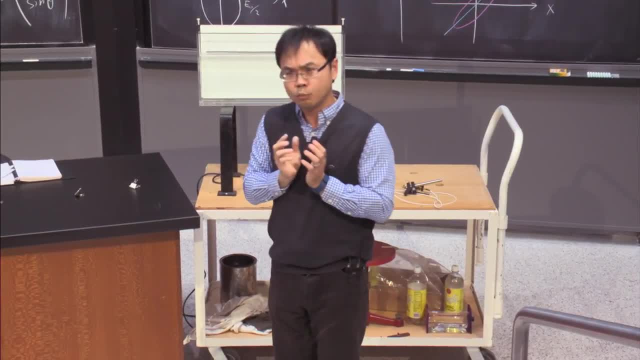 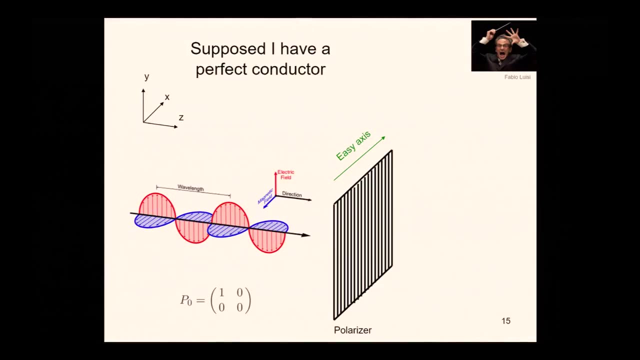 All right. And they were asking: can I move? Oh, yes, I can move in the oriental direction. So they jump up and down. Then they can actually cancel this electric field. OK, Therefore, what is going to happen when we have this perfect conductor? 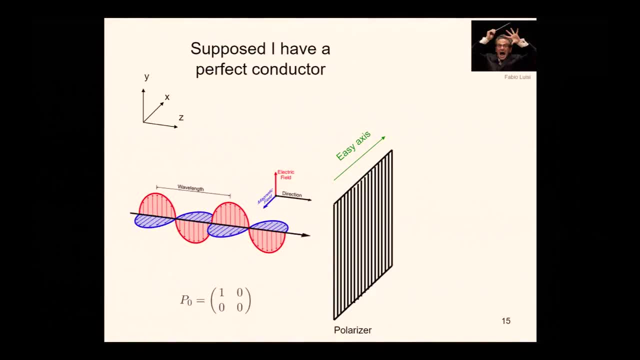 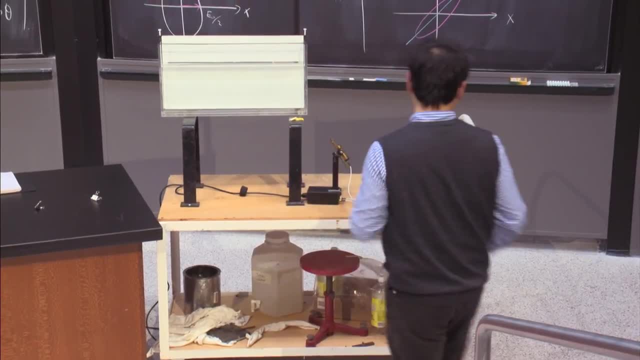 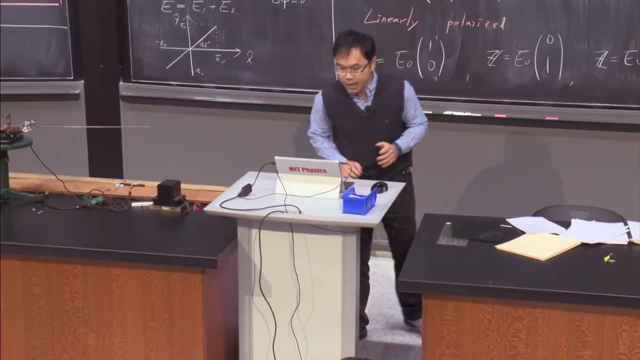 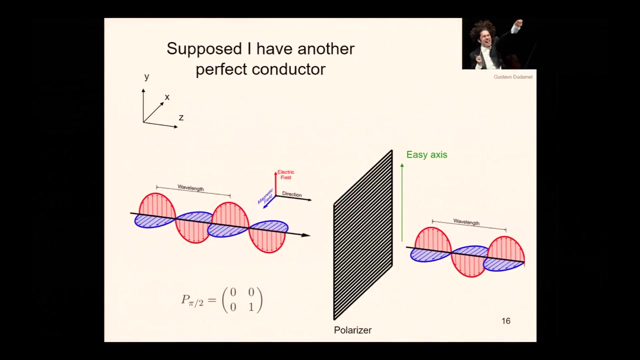 is that the electromagnetic field is going to be bounced back like what we had before when we talk about a metal plate. All right, So that's actually pretty nice. Now suppose I have another perfect conductor. OK, If I have another perfect conductor. 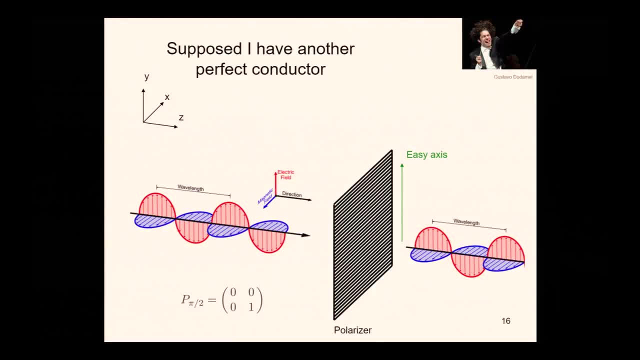 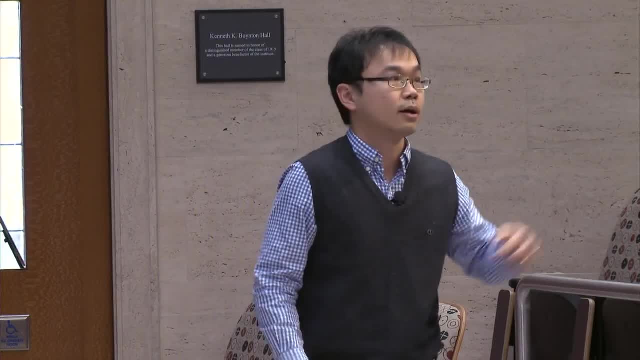 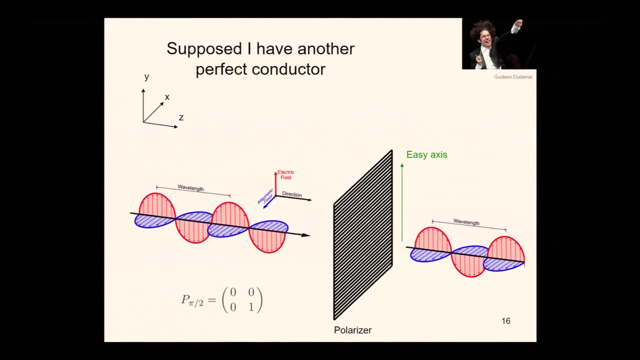 this time the perfect conductor is arranged such that all those charges can only move inside or outside of the board instead of going up and down. Now I have the incident wave, which is actually polarized in the oriental direction. OK, So you can see that this time the electrons 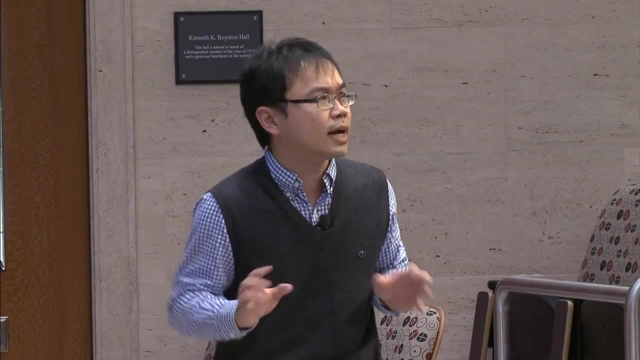 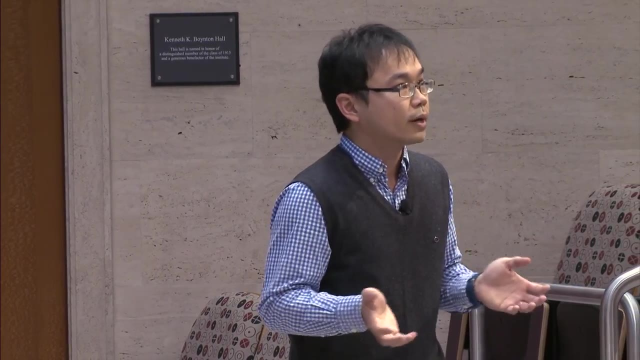 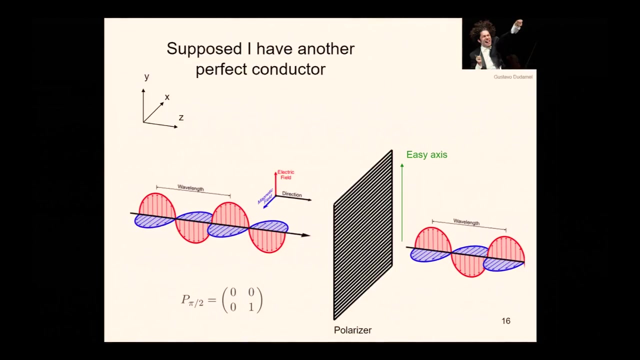 are really nervous about this And, oh no, I have to do something. But they cannot move up and down. Therefore, what is going to happen is that there is an isolation of electric field at this boundary And this polarized wave can pass through this so-called 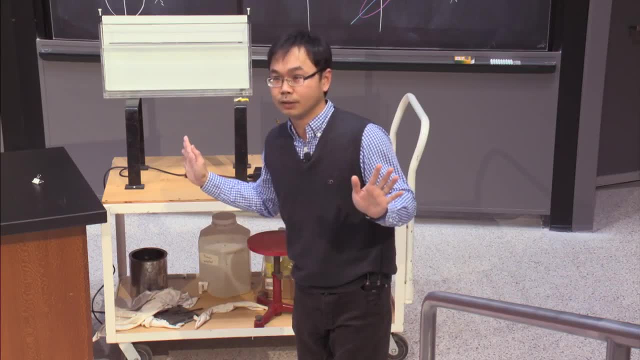 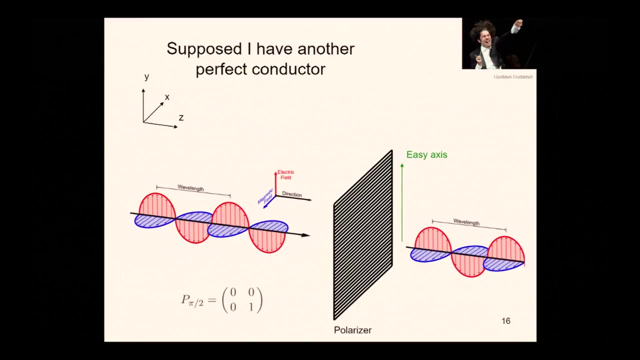 polarizer or perfect conductor, without getting stopped or get refracted. OK, And as you can see that in these two examples I have so-called the easy axis, So you can see that the easy axis, as the name actually tells you, the easy axis is the axis which is easy. 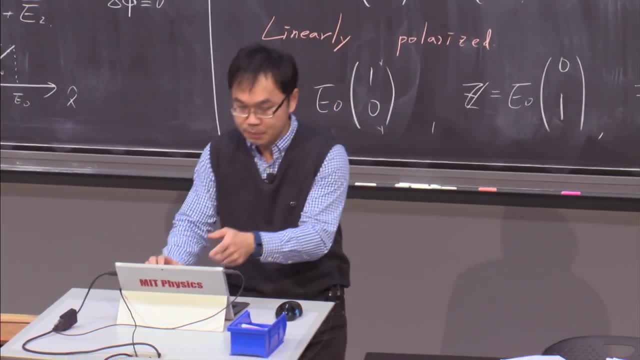 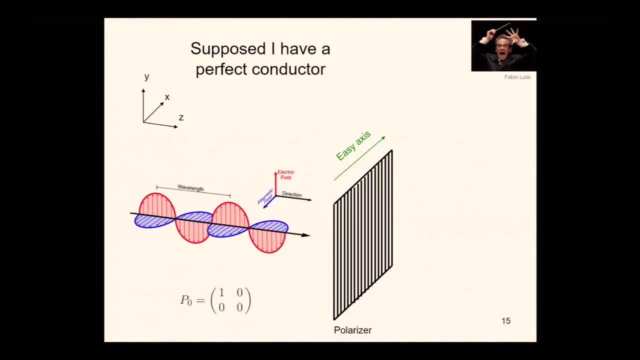 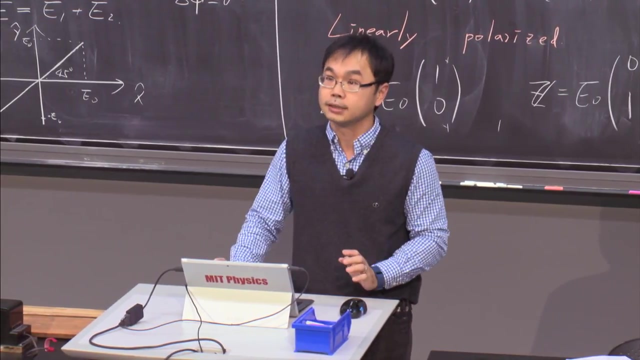 OK, All right. so what does that mean? That means if I have electric field aligned with the easy axis, it will pass through. OK, And the easy axis is perpendicular to the direction that all those streets I have in the perfect conductor. 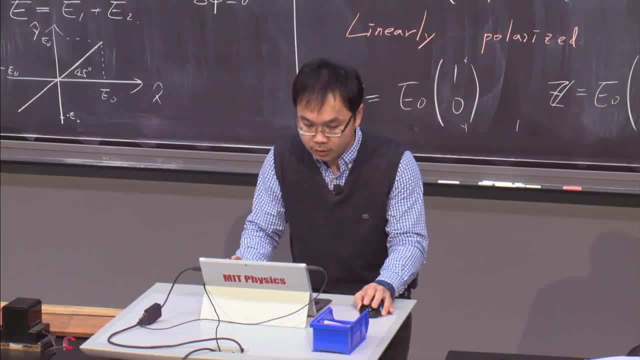 OK, Let's look at the first example. It tells you that, OK, the electric field is not aligned with the easy axis. That means it's not easy, All right, So it's got refracted. Oh, life is hard right. 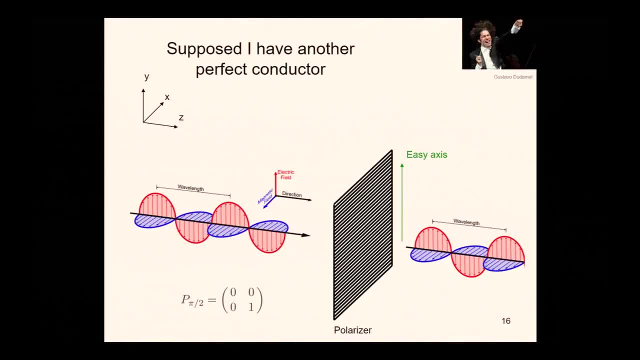 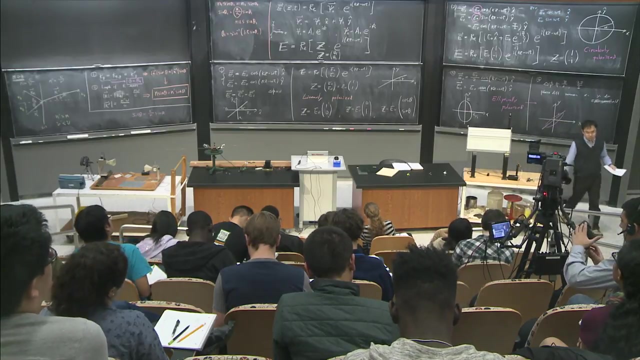 And the second electric field is smarter. It's got aligned with the easy axis And it passes through. OK, That tells you how I remember this so-called easy axis. OK, Any questions? OK, So we have been talking about all those craziness. 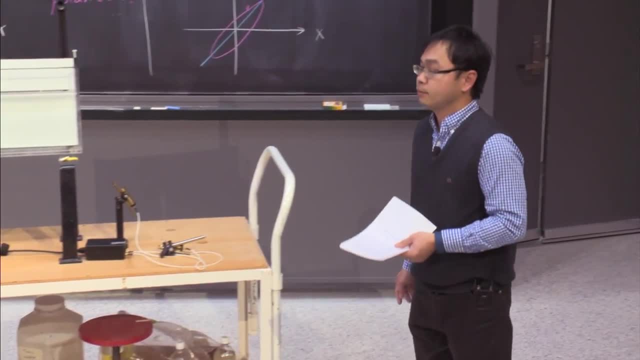 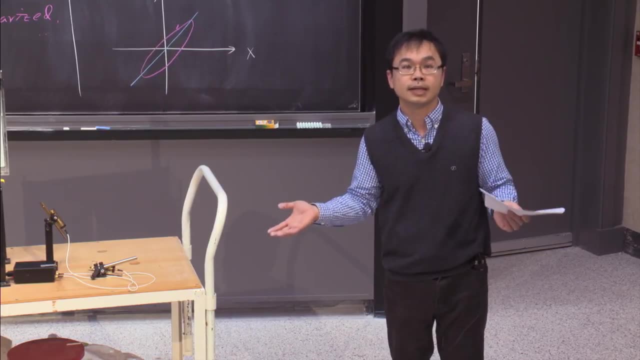 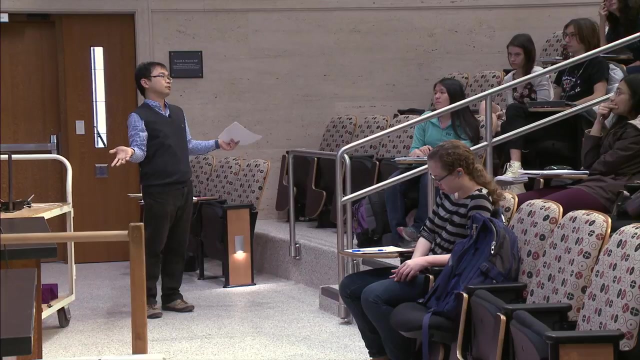 of polarized light, OK, And I hope that you also have learned about unpolarized light, because most of the lights are unpolarized. For example, light emitted from those light bulbs are not polarized Right, Because every emission of a photon 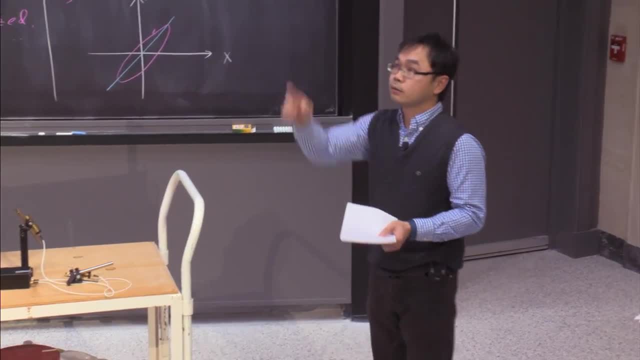 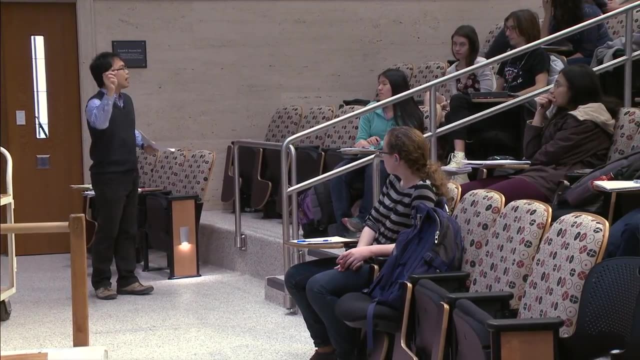 can be aligned in different direction. Right, Therefore, I OK. as I was talking about, there are infinite number of photons hitting my face and bounce back to your eye. Right, All those things are not aligned to the same direction as what we have been discussing before. 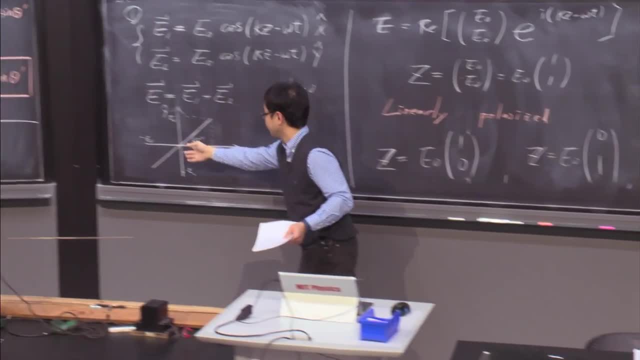 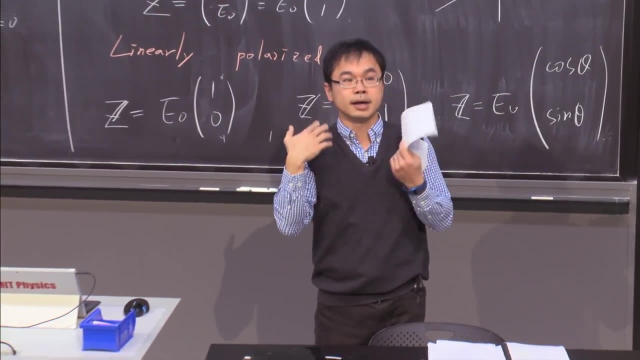 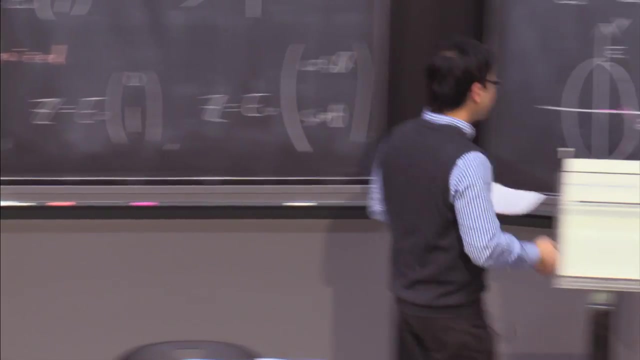 Right. So if I linearly polarized the wave, it's going to be all the electric field is pointing to the same direction And apparently those lights hitting my face is actually not aligned And it's actually pointing to random direction. OK, 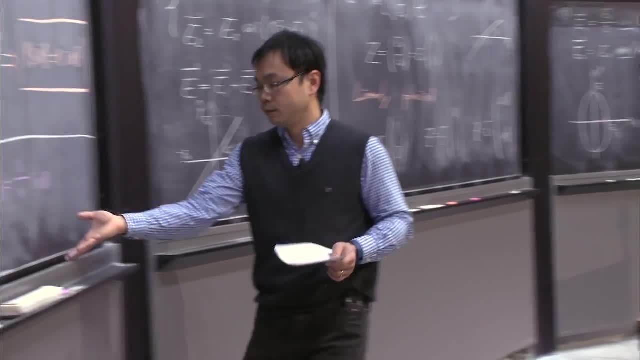 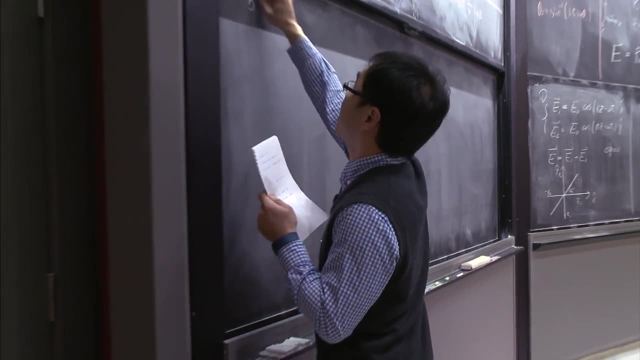 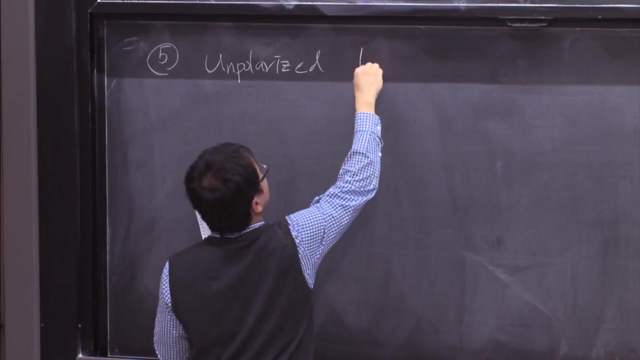 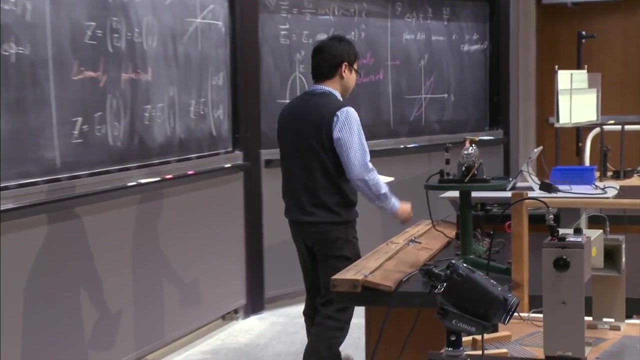 So that brings me to the fifth situation which I would like to talk about. The fifth situation is that I could have unpolarized, Unpolarized light. OK, So what do I mean by unpolarized light? Light means electromagnetic waves, which. 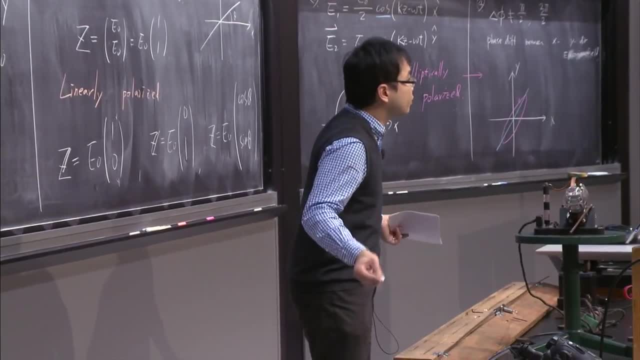 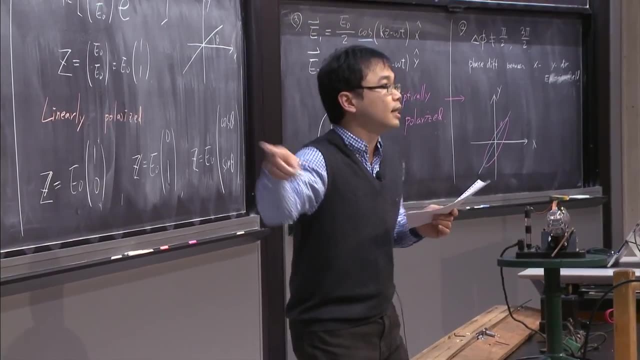 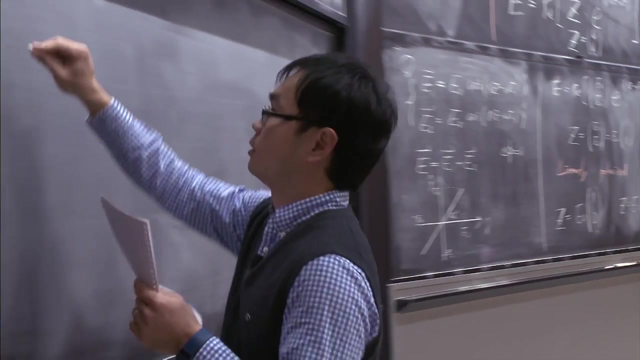 were produced independently by a large number of uncorrelated source. OK, You may ask, OK, wait, wait, wait. Unpolarized means that we have a lot of different light source pointing to different angle. Shouldn't it just look like this? 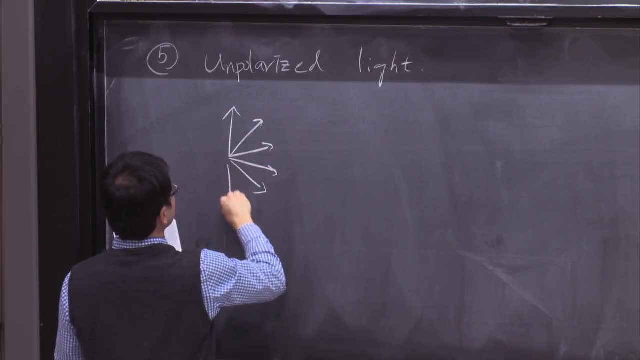 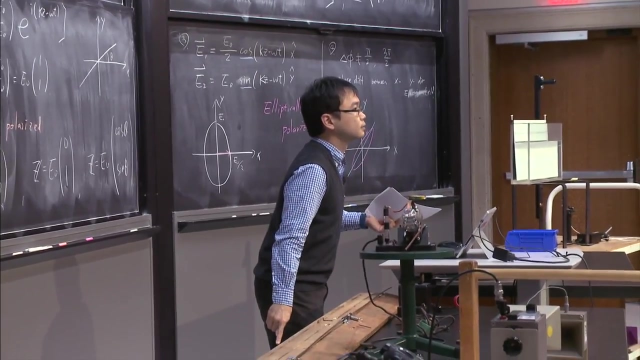 So you have pointing this direction, all the direction, all the possible direction, pointing to all different possible direction, like this Right. Shouldn't that diagram actually tell you something about unpolarized light? Life is hard If everything is aligned, and also 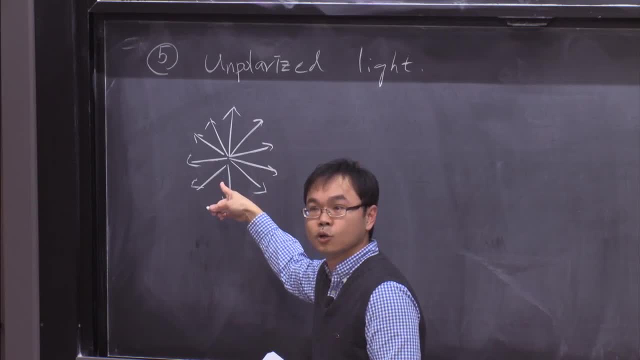 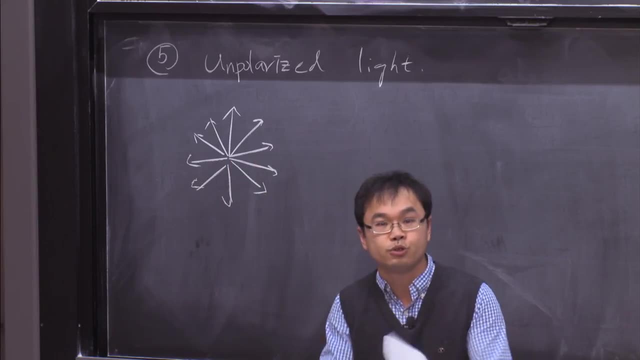 if everything is arriving at the same time, like this, OK, what is going to happen? They cancel, Right, Because all those things are vectors If they reach maxima at the same time, this means that they are emitted always at the same time. 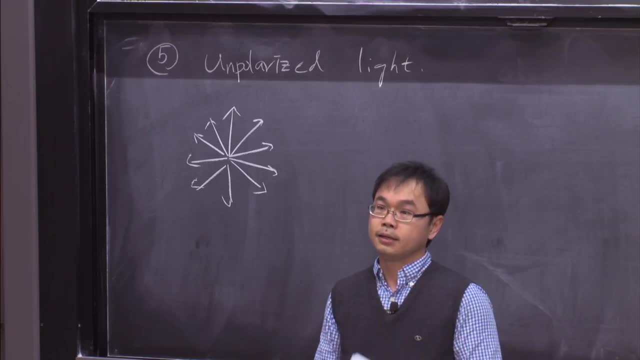 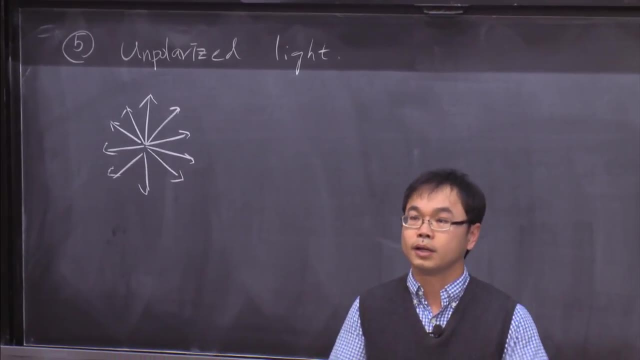 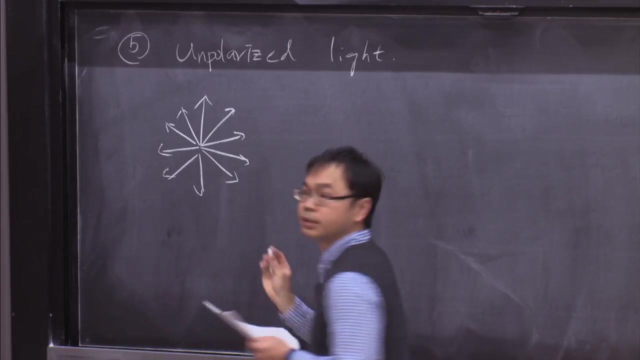 but in random direction and emitted at the same wavelength, then they are going to cancel all each other. So apparently that's actually not what unpolarized light is. What I mean is that they can be pointing to different direction, but the emission time and the wavelength 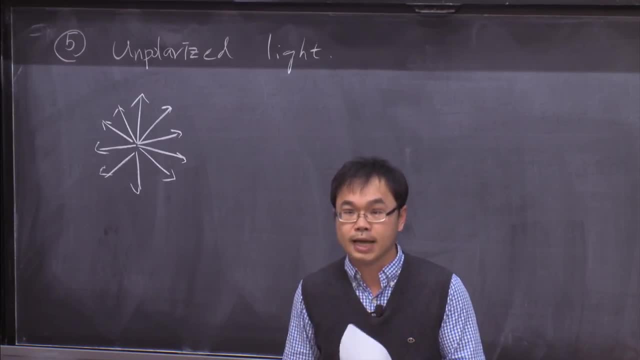 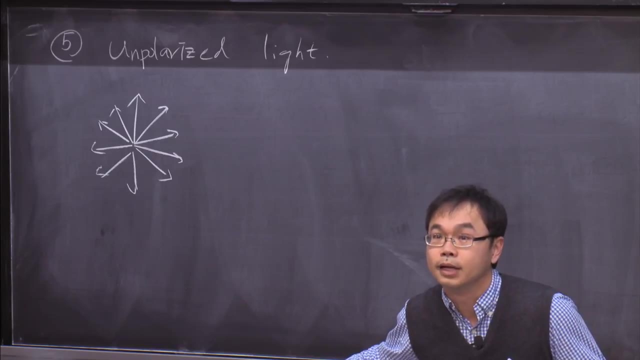 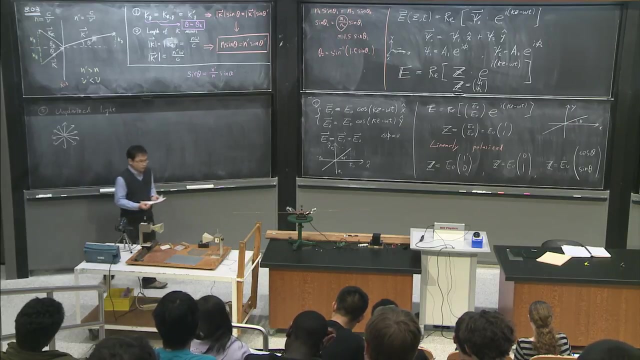 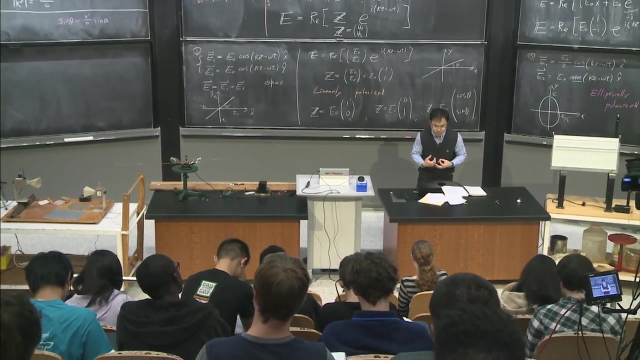 of all those emitted electromagnetic wave can be slightly different. Otherwise they will just cancel each other completely. OK, Any questions about what I just said? OK, So very good. So now what I'm going to do is to show you some examples related to polarizer. 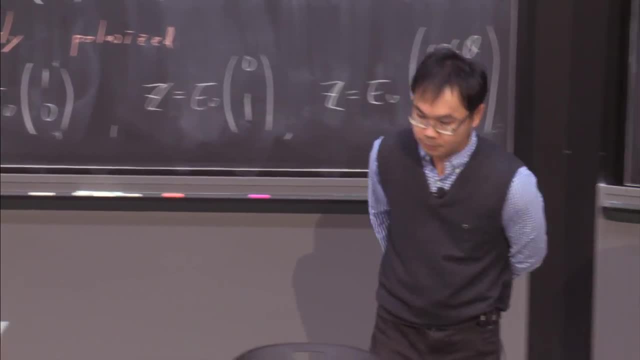 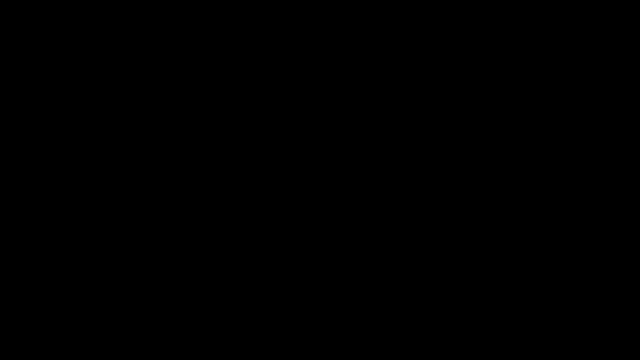 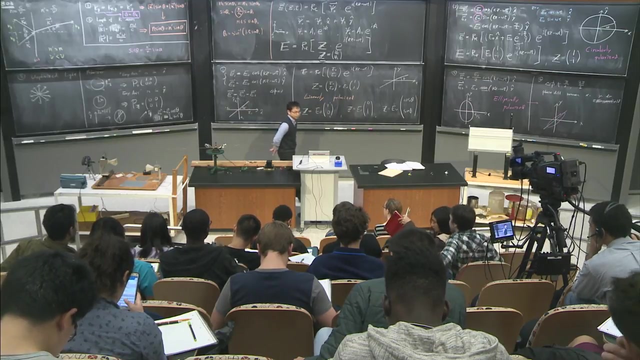 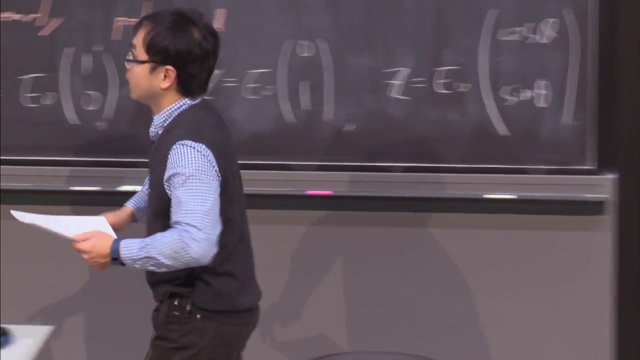 Before that, I will take a five-minute break before we come back to the demonstration. So we will come back at 36.. OK, So welcome back. So we will continue the discussion of the polarized wave and the polarizers. So before that, actually I already 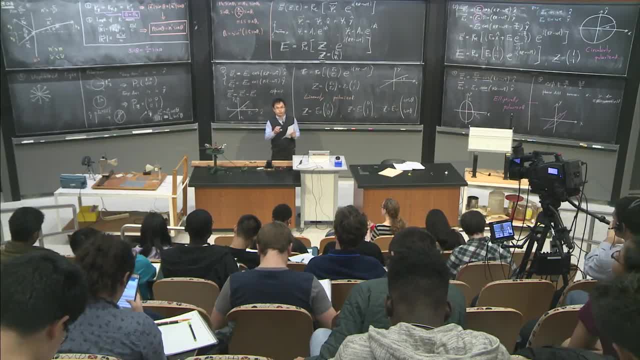 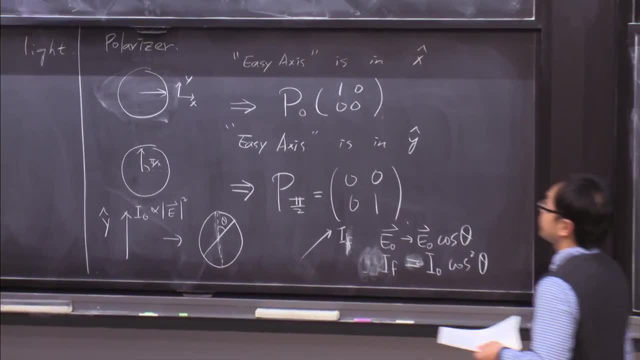 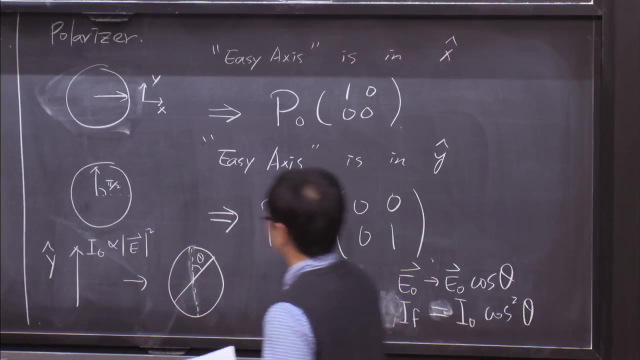 introduced the polarizer by the perfect conductor, arranged in x-direction or y-direction, many of them in strips aligned in x-direction and y-direction, And usually we use a simple diagram like this: a circle and an arrow, to indicate the easy axis. that will actually tell you about the property. 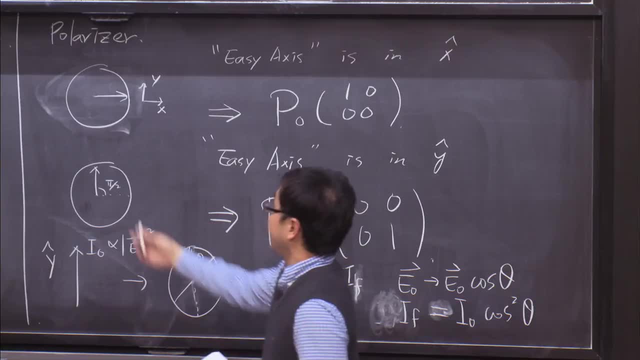 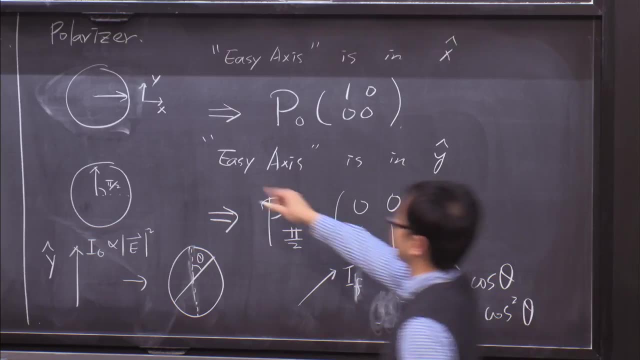 of the polarizer. OK, So in this case, if I have a circle and I have an arrow which is actually pointing toward the x-axis, In this case, my coordinate system is here: Oriental is x, Vertical is y. 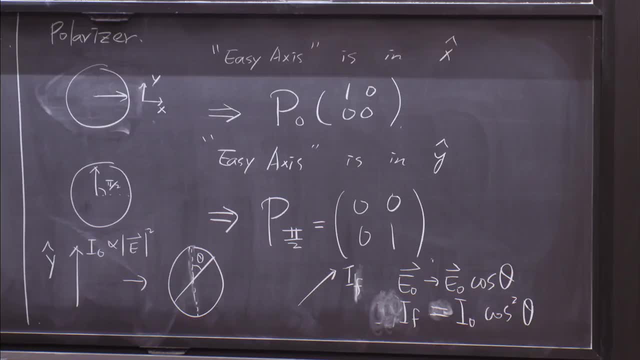 That means my easy axis is actually in the x-direction. OK, And I can actually write down what will be the matrix, the representation of P0, which will actually present the effect of this polarizer. OK, The P0 will be a matrix in this form: 1, 0, 0, 0.. 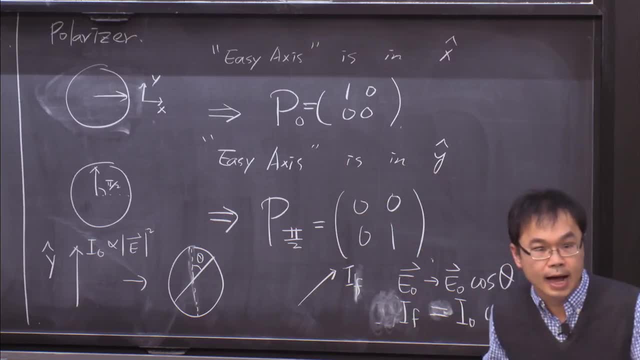 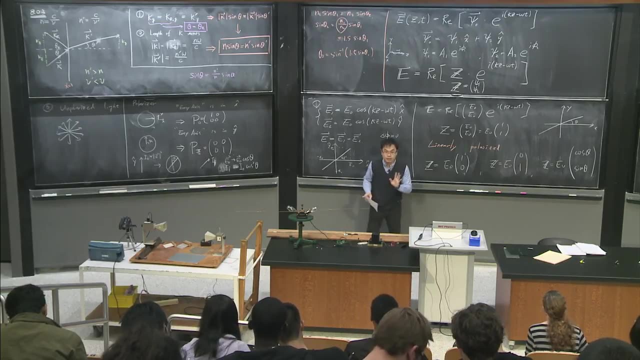 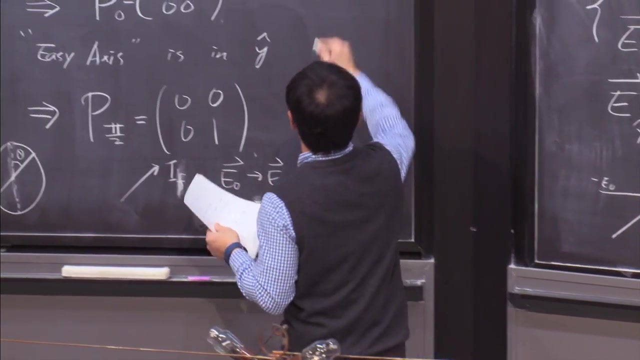 OK, If I have this P0 acting on the z, which is actually, for example, I can have the P0 acting on the z, then, basically what I have been doing, what will happen after the light pass through this polarizer will become z times multiplied by P0. 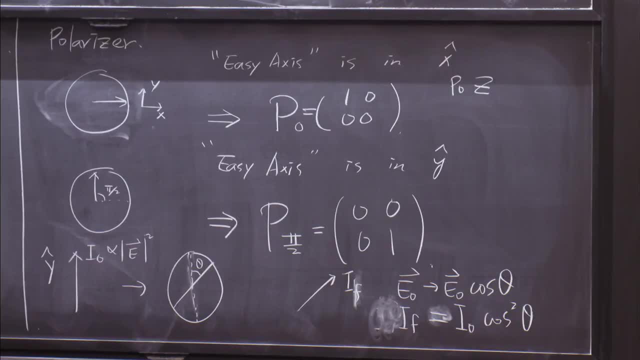 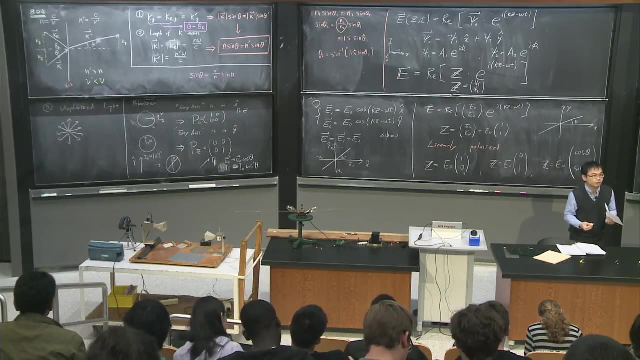 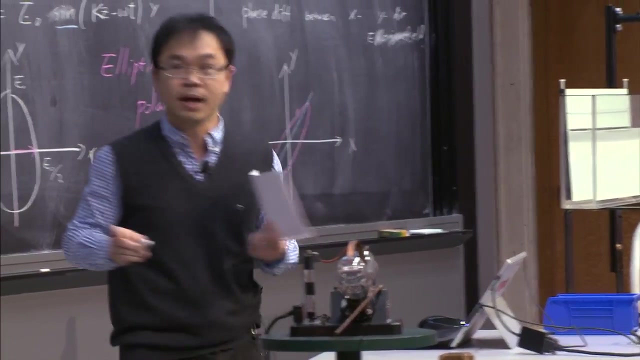 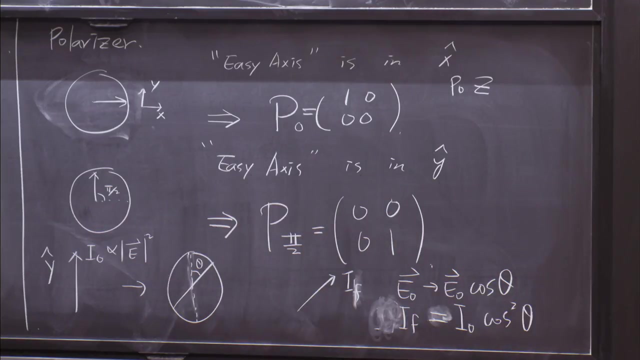 OK. So basically, all this P0 matrix does is to actually extract the projection of the field in the x-axis. OK, But I am just writing it down in the matrix format. And on the other hand, for example, if I have this easy axis which is 90 degrees, 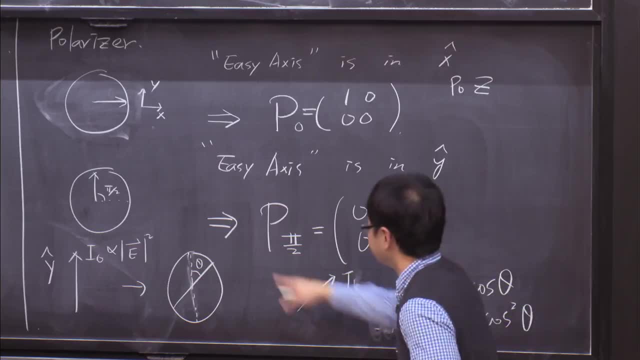 with respect to the x-axis, which is in the y-direction, then I really write this down in the form of P, pi over 2.. This pi over 2 is actually the angle between the easy axis and the x-direction. OK, And in this case you are going to get 0, 0, 0, 1,. 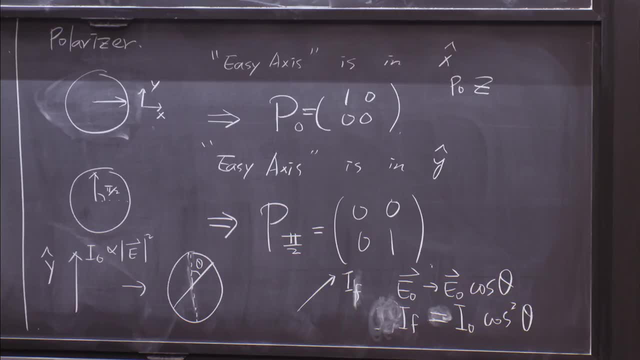 because all this matrix actually does is to extract the component which is actually in the y-direction. OK, And you can of course multiply. when you have an incident electromagnetic wave which you can actually extract, the polarization z matrix, You just multiply P, pi over 2 and the z. 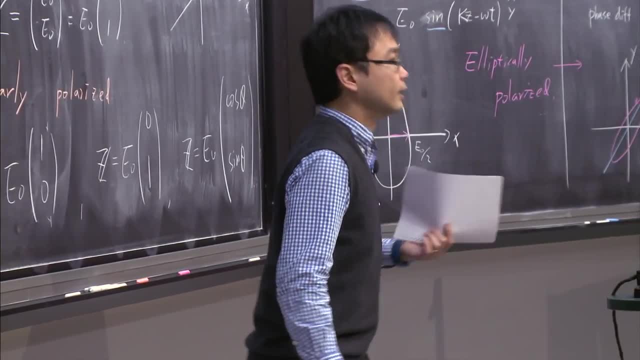 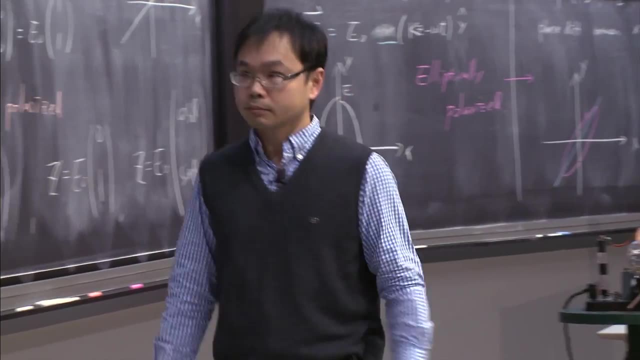 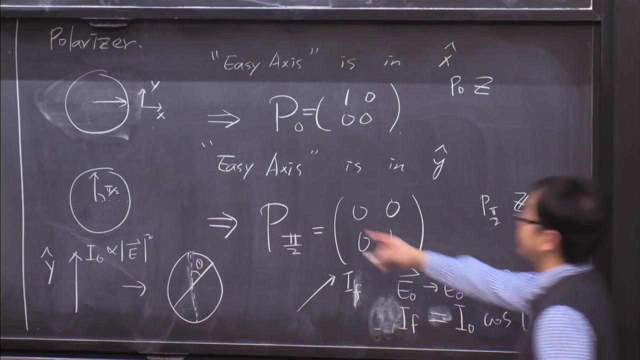 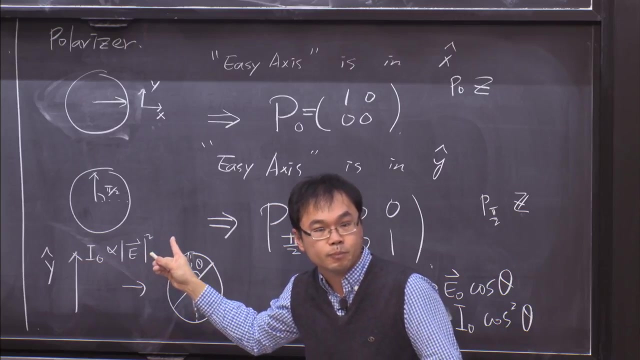 Basically, you can actually get the resulting polarization of the electromagnetic field after passing through this polarizer. OK, What is going to happen is that only the y component will survive. OK, In the case of easy axis aligned in the x-direction, only the x component will survive. 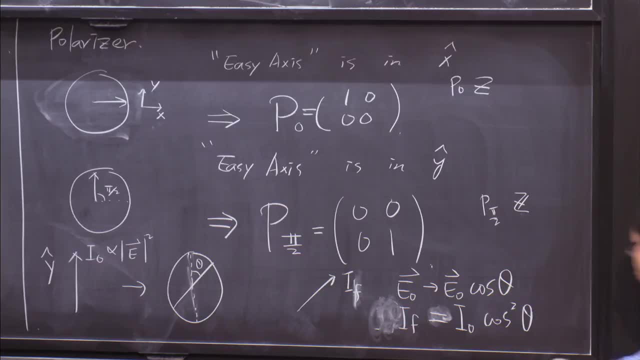 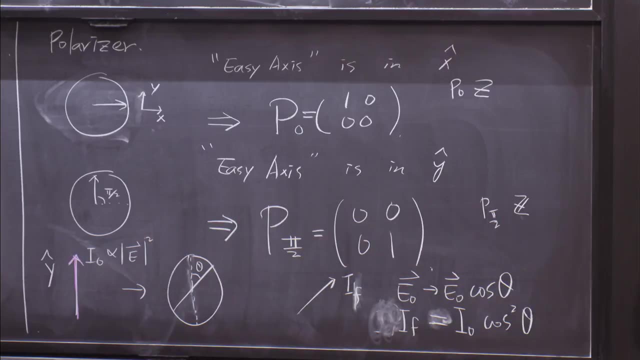 OK, So let me actually go through a short example here. So suppose initially I have the electromagnetic field linearly polarized in the y-direction, OK, And I have that electromagnetic field passing through a polarizer which is actually zeta degree away from the y-axis. 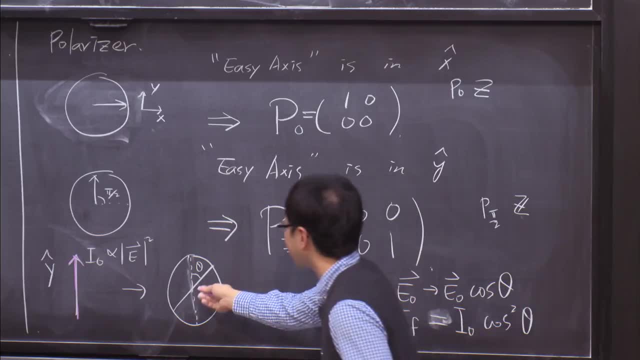 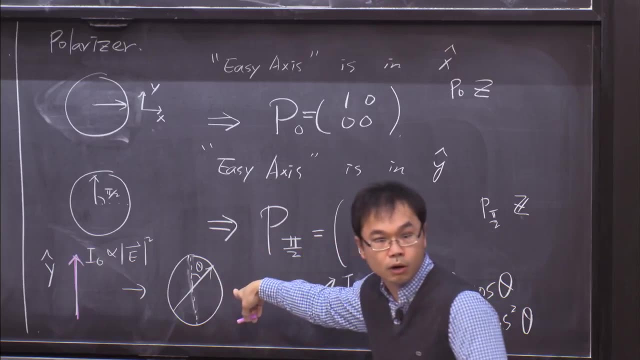 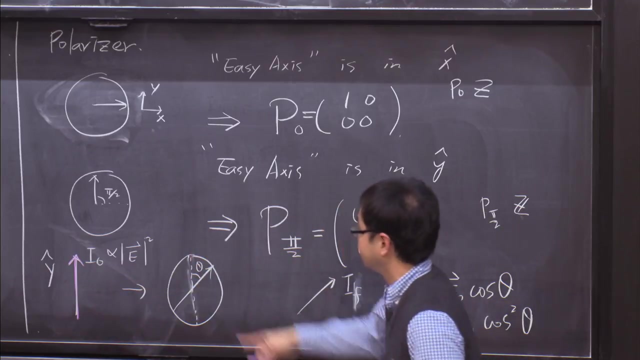 OK, So what is going to happen is that all the component which is actually parallel to the axis survive. So all the component of this, all the projected component in the axis perpendicular to the easy axis, didn't make it, Because the electrons are going to be oscillating up and down. 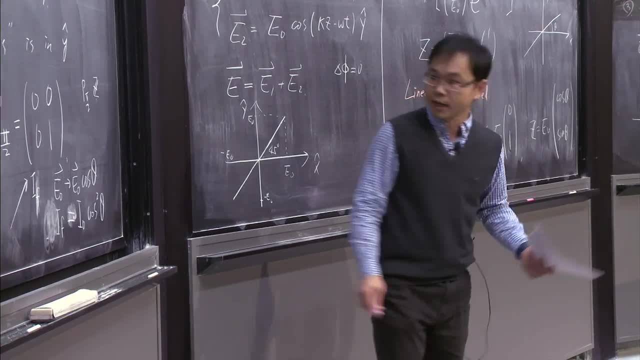 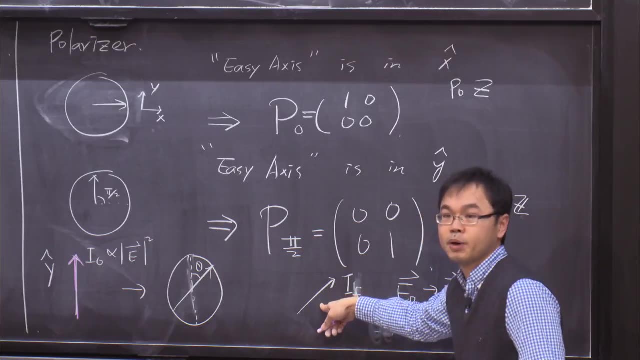 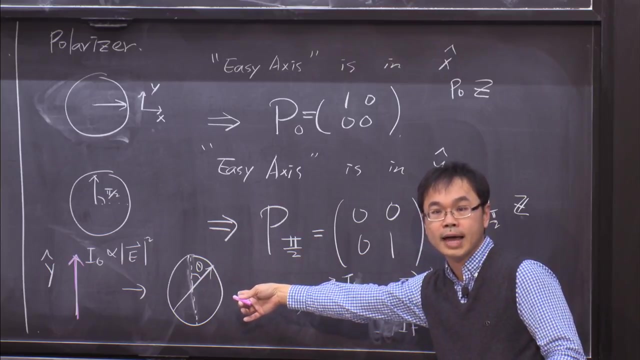 like crazy to compensate and then refract that component. OK, So what is going to happen is that, after passing through the easy axis, the direction of the polarization will be altered such that it's actually in line with the polarizer, the easy axis of the polarizer. 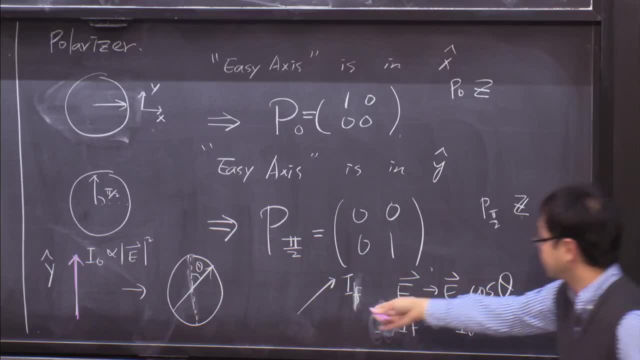 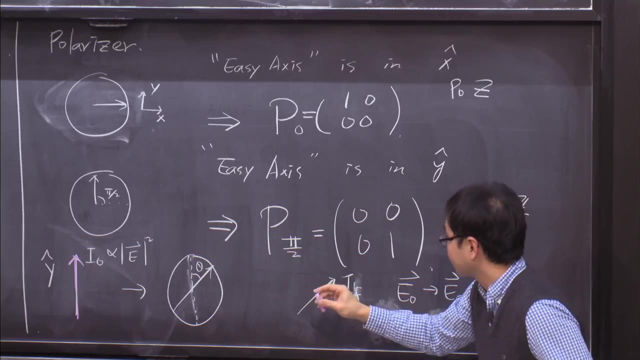 OK, So you can see that after passing through this polarizer, the direction of the polarization, this is actually still linearly polarized. OK, The direction actually changed by zeta degree And also the amplitude also changed, Because only the component parallel. 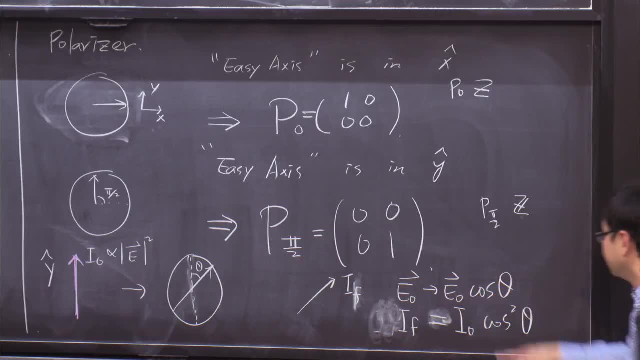 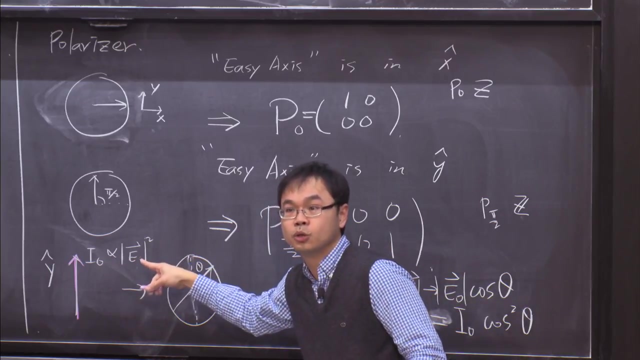 to the axis survived. Therefore, the magnitude of the e vector become e0 cosine of cosine zeta And therefore the amplitude of the light got reduced. It become i0 cosine zeta squared, Because the intensity of the light is actually proportional to e squared. 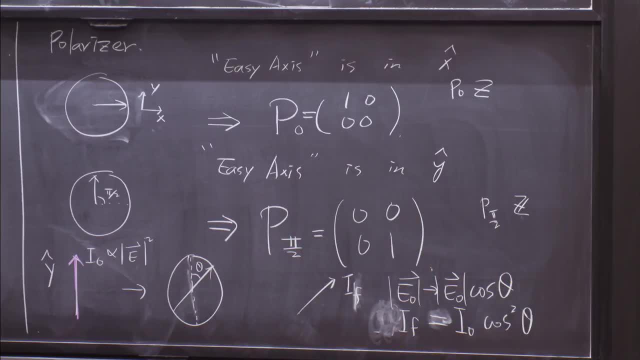 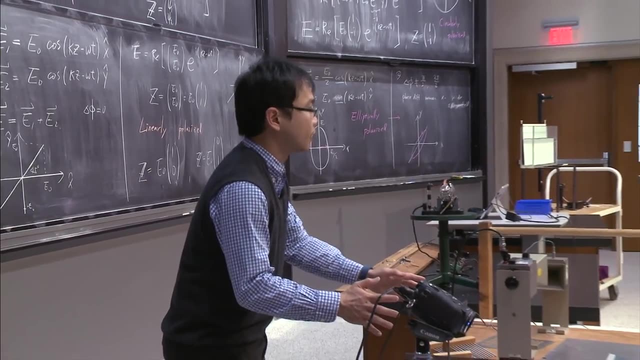 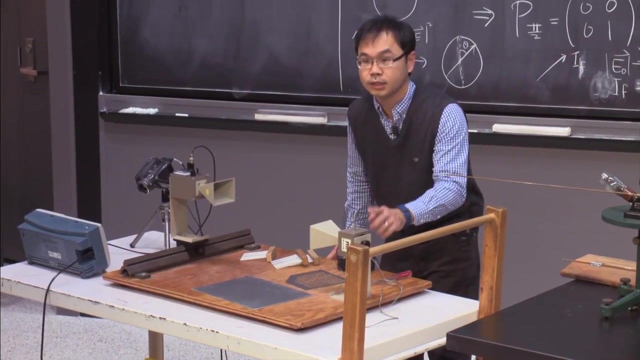 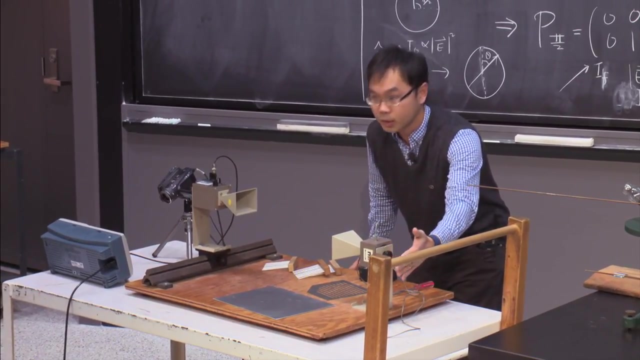 OK, So after all this, So this is time to take a look at some demonstration here. OK, So here I have a setup which actually I have emission of linearly polarized microwave from the left-hand side, which is the source. 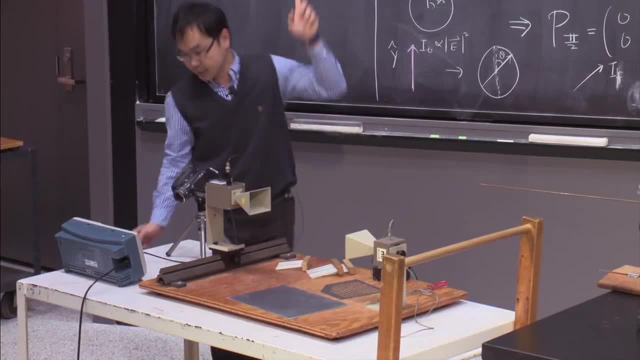 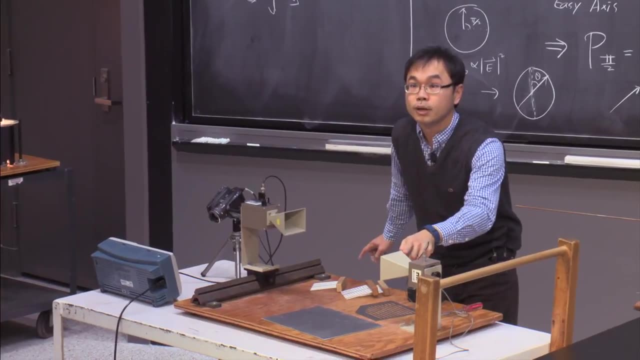 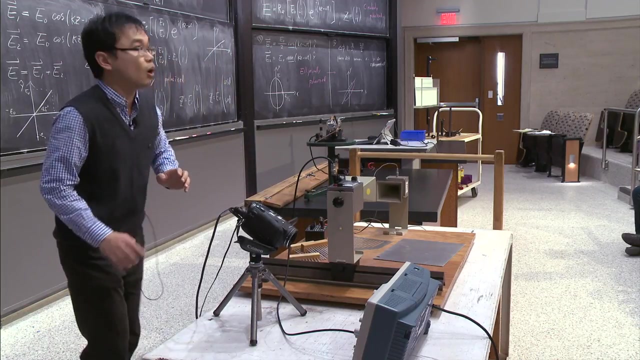 And I have a receiver which is actually connected to the scope. You can see the result. You can see that, indeed, there are energy passing from this source, And it got accepted and then recorded by the scope. OK, Now I have all those. 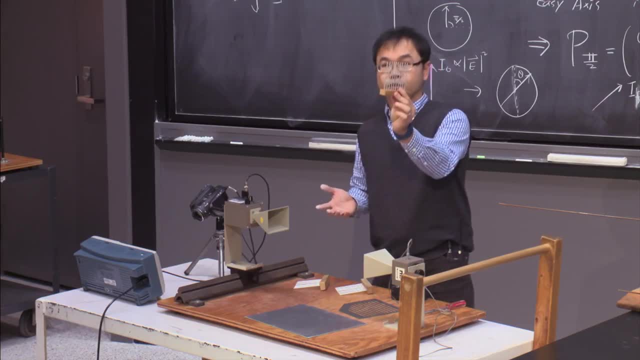 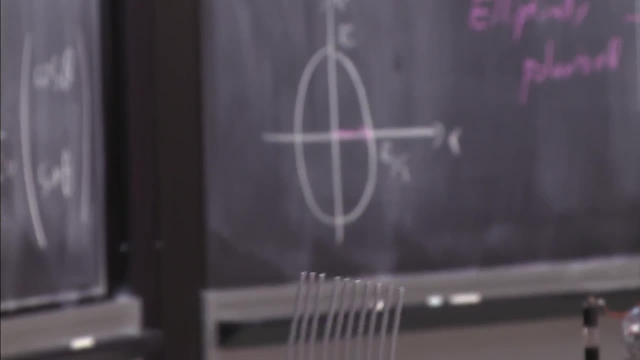 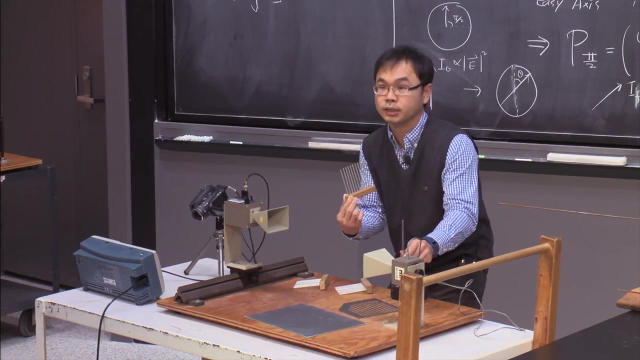 OK, All are not so perfect, But those are metals OK, which actually have many, many streaks or maybe a little rot here, And if my polarization, Or initial linearly polarized wave, is actually pointing in the vertical direction. 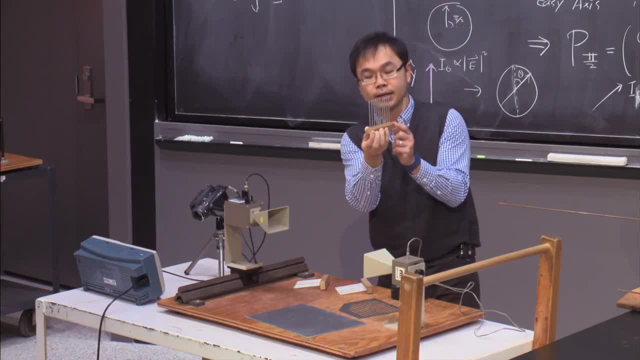 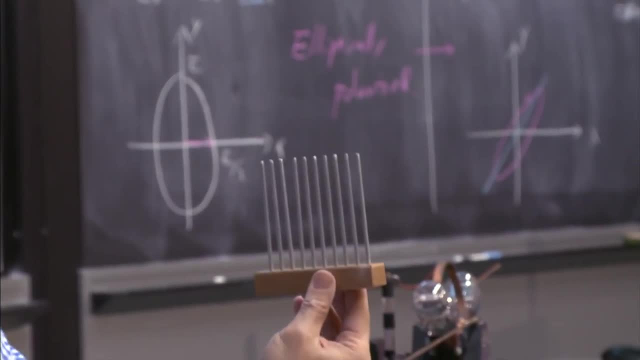 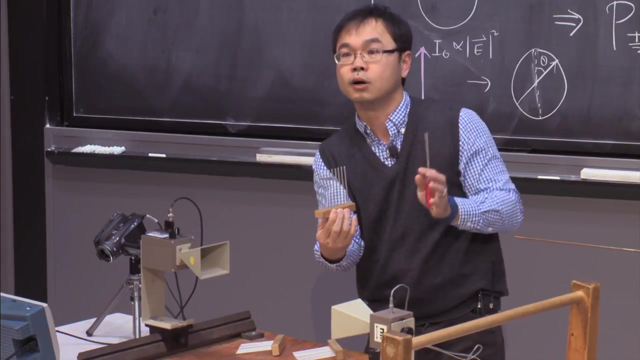 So if I have my polarizer arranged in this direction, can you predict what will happen to the redial on the scope? Will I see signal or not? How many of you actually think we will see signal? OK, If I arrange that the electromagnetic wave 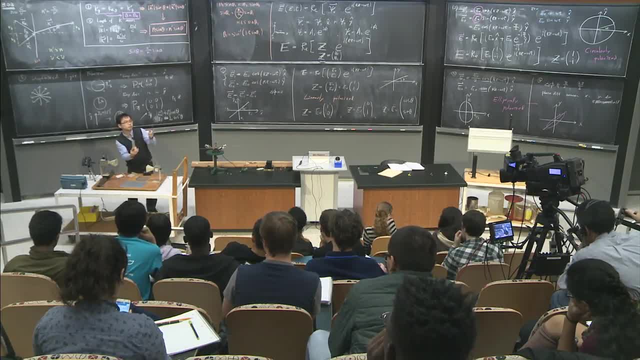 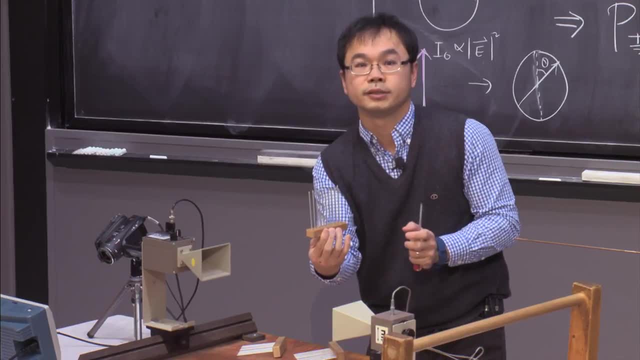 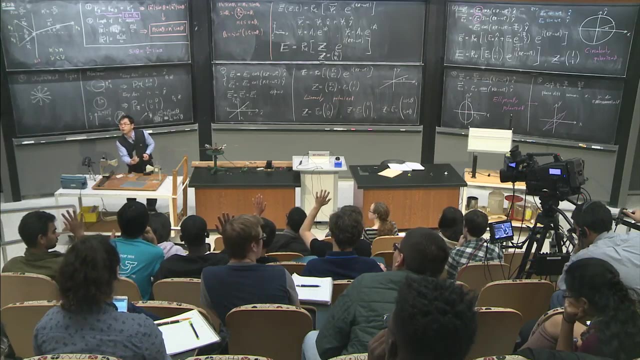 is actually polarized in the up and down direction. OK, One, two, three, OK, And these four people think so. How many of you think nothing will change? Oh sorry, Nothing will be observed by the scope. OK. 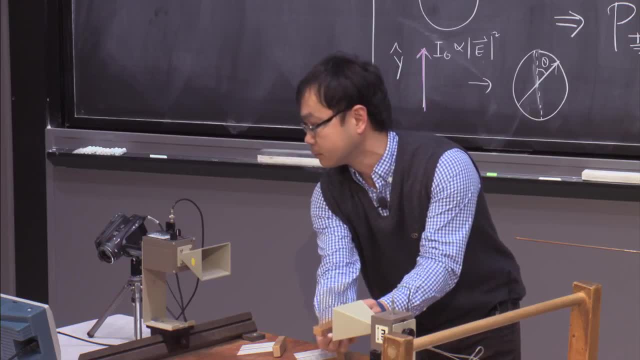 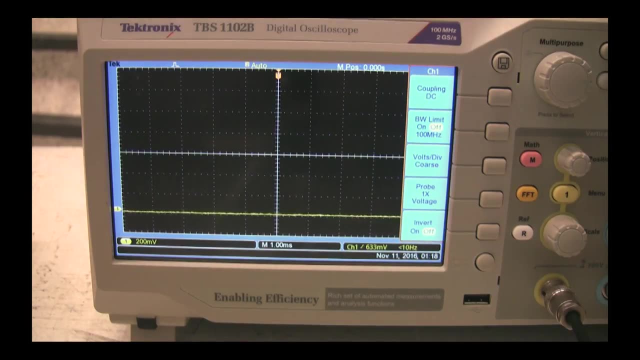 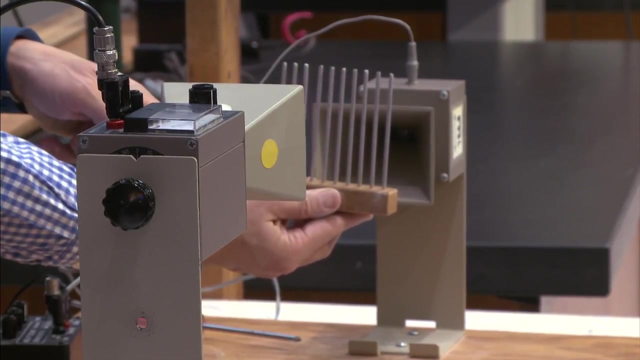 Most of you actually think so. So let's actually really do this experiment. Look at what is happening. Can you see it? Do I see a signal? No, All the signals are canceled Right. Why? Because all the hard work of all those electrons in the metal. 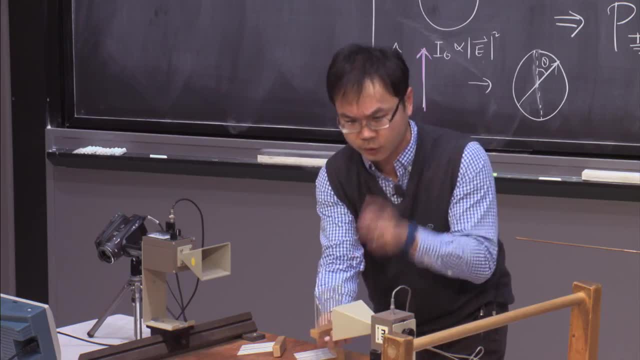 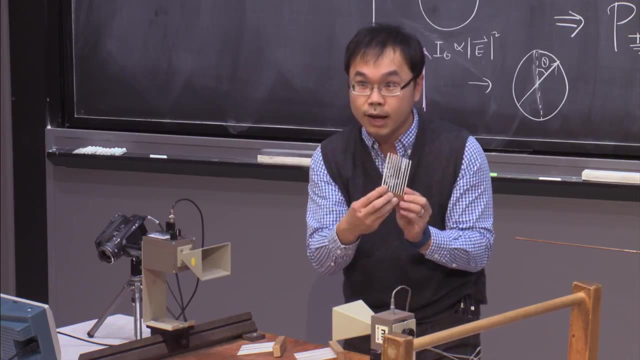 they're like crazy. Oh my god, This is a disaster. I'm going to isolate up and down. Cancel, cancel, cancel. Then it got canceled. OK, On the other hand, I can save all those electrons Right. 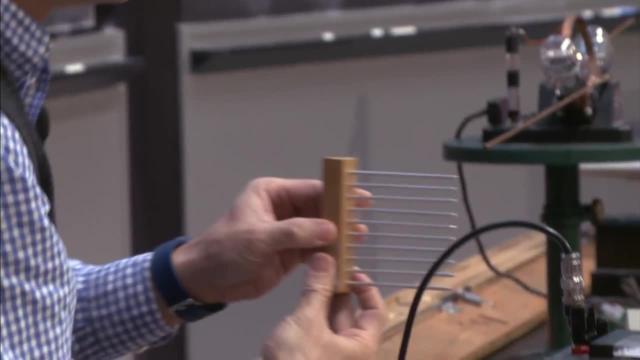 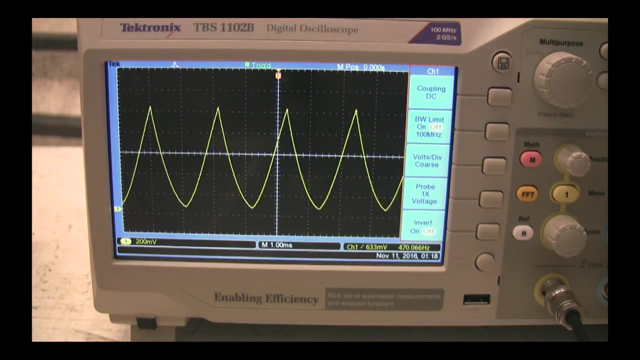 So now I'm going to rotate this thing by 90 degrees and see what is going to happen. Can you see it? Can you see it? Can you see it? Nothing happened right, Because those electrons, oh my god, Crisis coming. 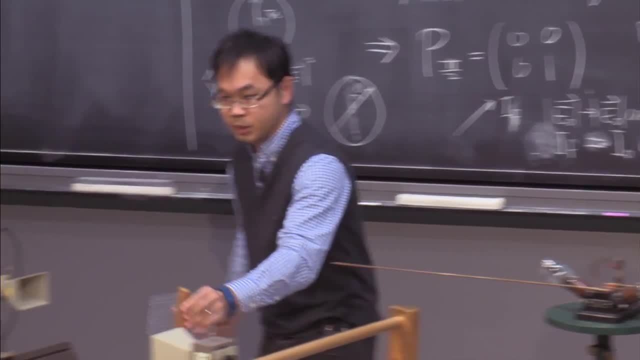 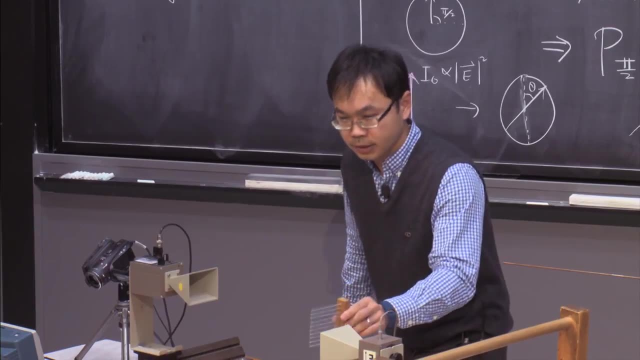 But there's nothing I can do because I cannot move up and down. Therefore there will be no refraction. OK, So they have just to accept that the fact that, OK, this electromagnetic field went through. OK, All right. 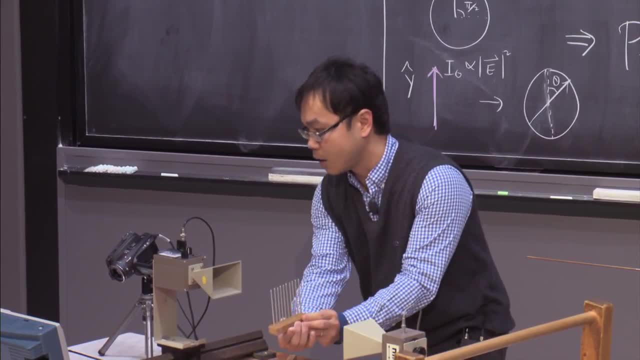 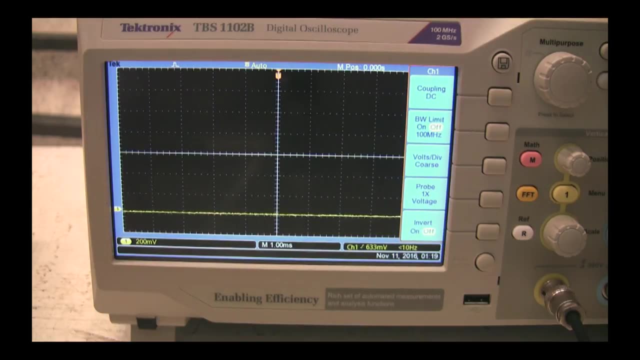 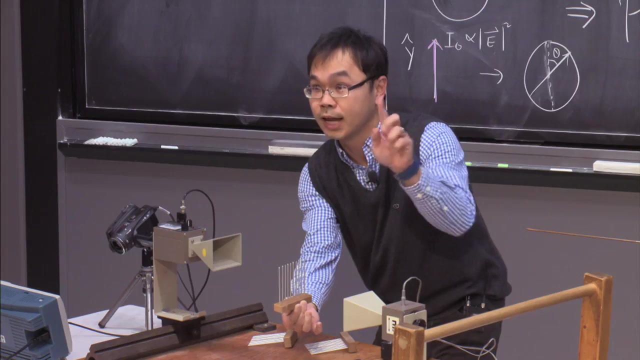 And let's actually do something really interesting. OK, So now I have, I can actually. OK, I can actually make electromagnetic field completely destroyed, right? Because originally the electromagnetic field is linearly polarized up and down in this direction. 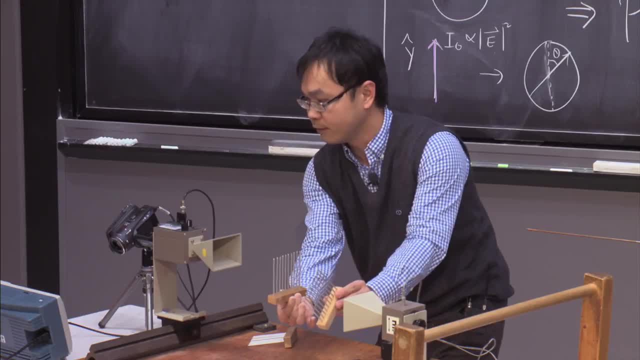 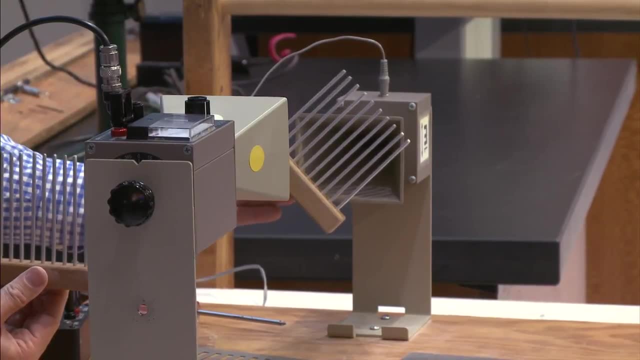 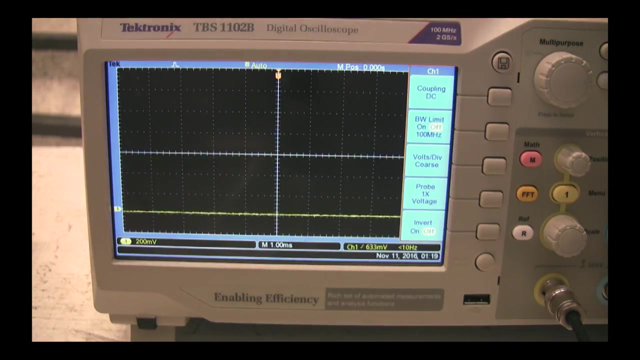 OK, If I have another plate which is actually 45 degree, OK, So if I have a plate which is 45 degree and I put in another one here, OK, it doesn't really work very well. OK, the signal probably is too small. 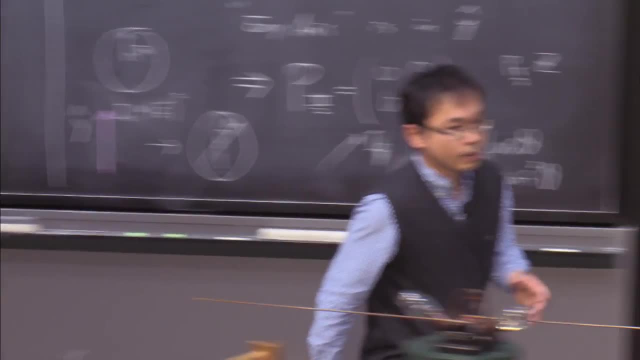 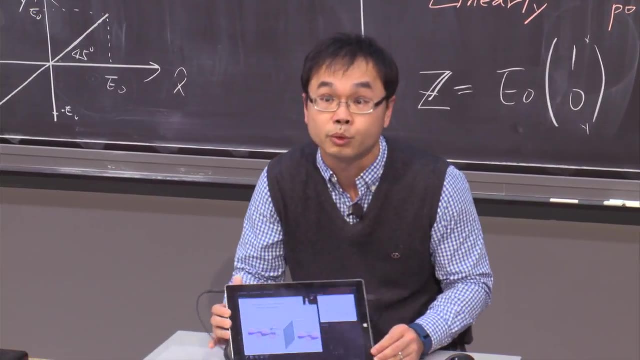 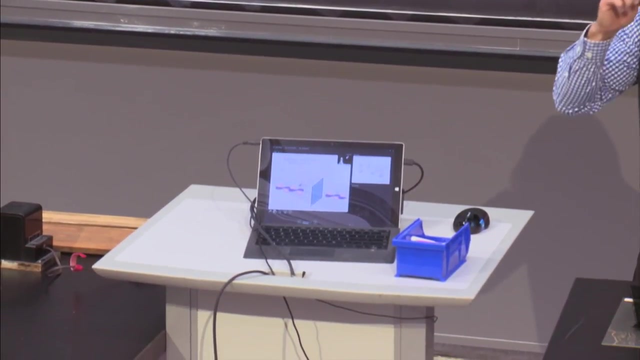 And OK, how about we do this demo in a different way? So right now, here I have my computer here. Can you see my computer? You can see the screen right? OK, The screen is actually made of LED. Those LED screens actually emit polarized light. 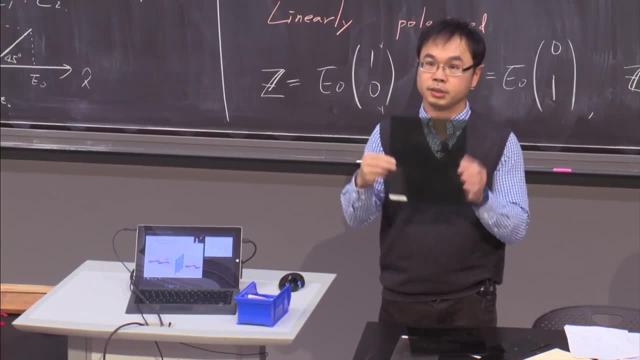 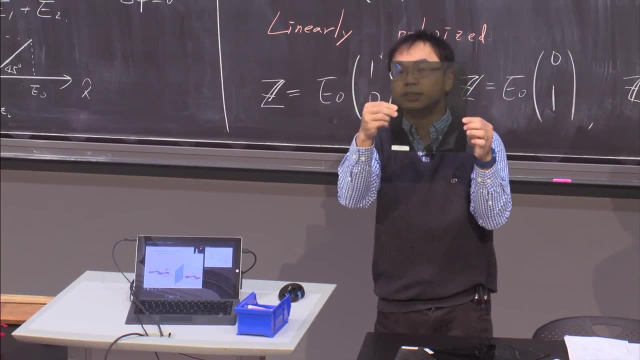 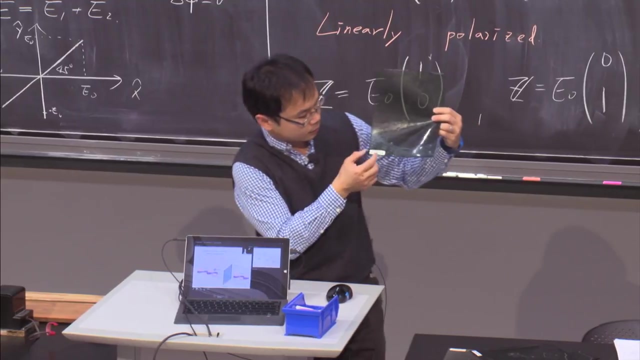 And those are the polarizer, which is actually the equivalent version of those metals, but they're actually arranged in a really fine grain, So you cannot really see all those strips And they look pretty transparent, But the idea is pretty similar. And the polarizer? 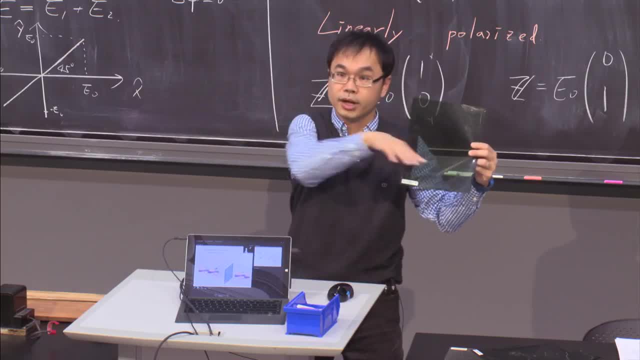 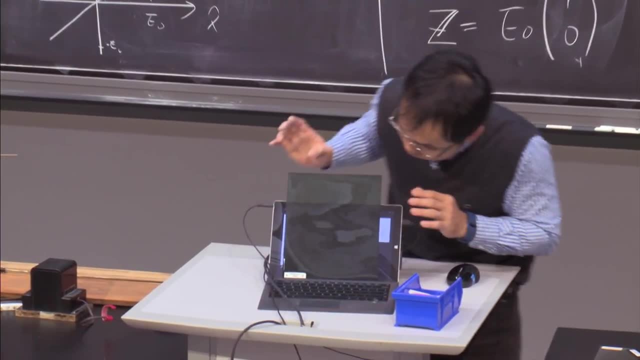 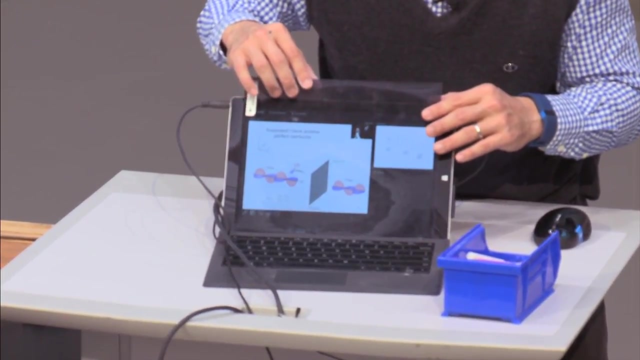 The polarizing axis is actually in the oriental direction. The easy axis is in the oriental direction. So let me put this here. Can you still see the screen? You cannot right. But if I rotate this by 90 degree you can see it right. 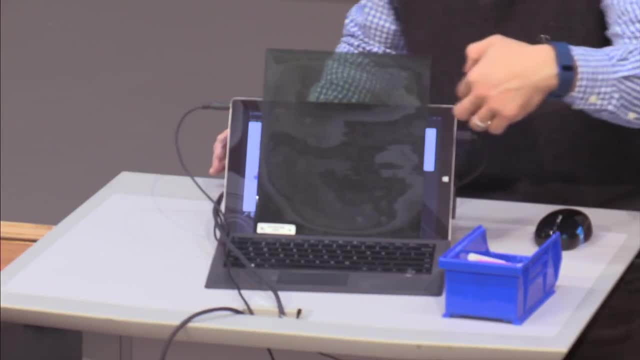 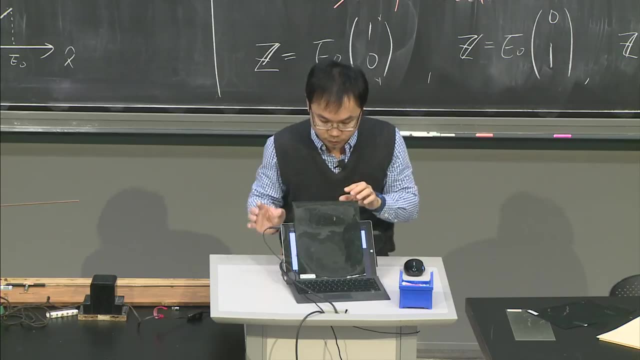 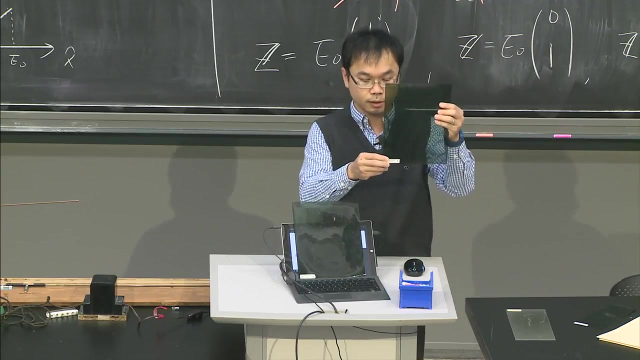 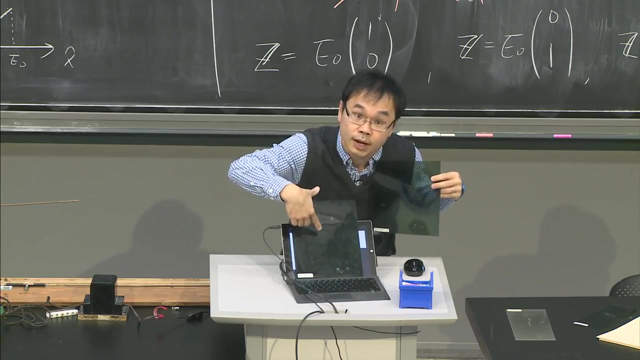 That is because all those light emitted from this screen is actually linearly polarized up and down direction. OK, So now if I have another identical polarizer which I insert between these two? so now you cannot see anything right, Because all the light is actually moving up. 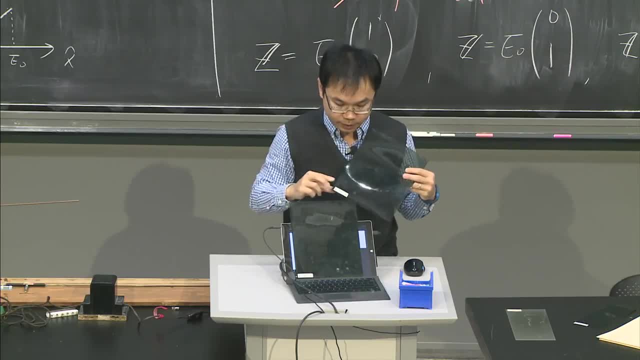 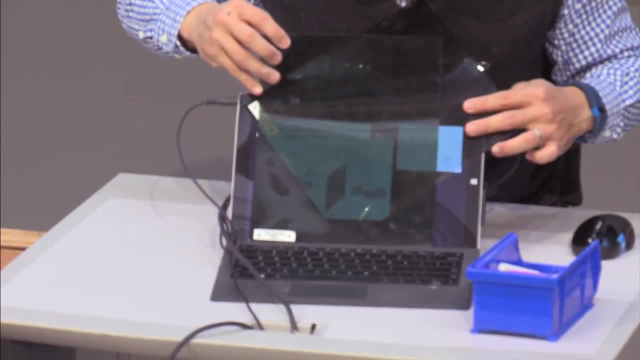 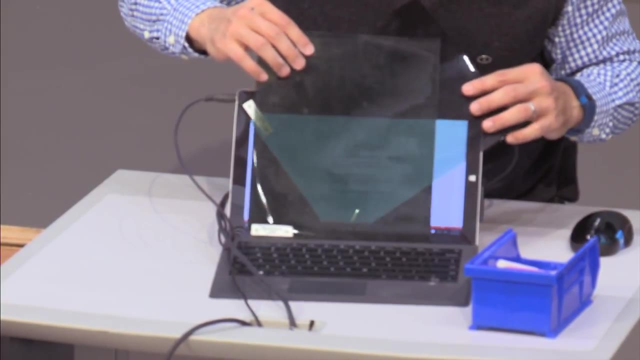 OK, pointing up and down. All the electric field is pointing up and down. And now, if I insert another one, which is 45 degree, you can see it. You can see it Why? That is because, if I insert this additional polarizer, 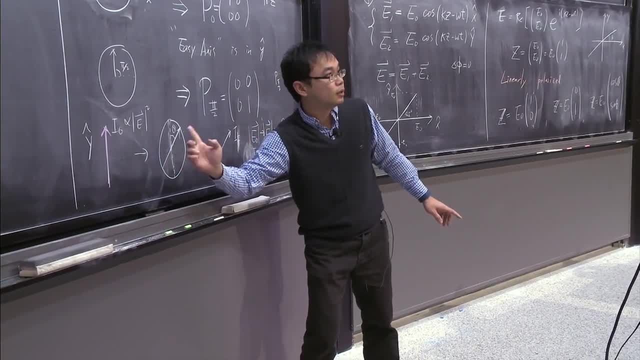 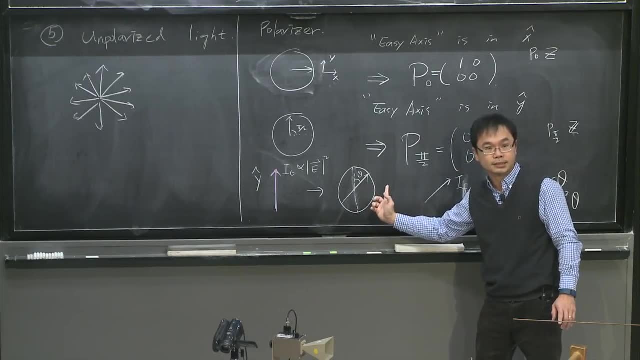 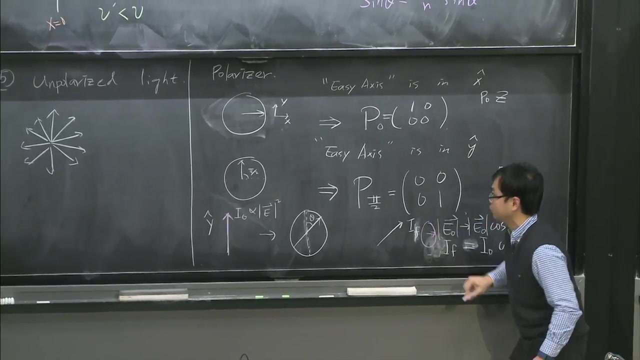 like what I was discussing. it's going to take the projection to the direction of the easy axis And if I have another one which is actually pointing up, this is pointing toward the x direction. then again, since this vector is tilted already, 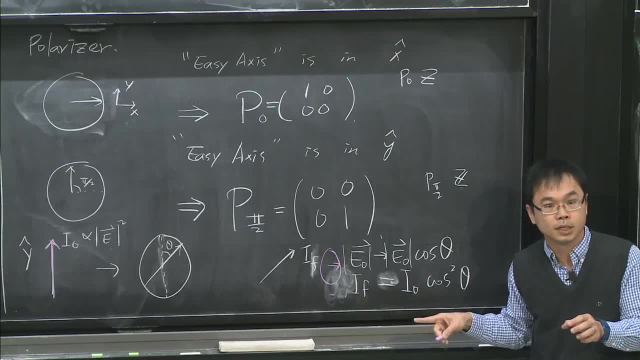 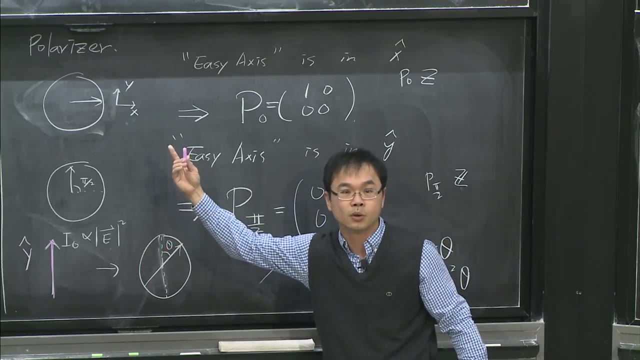 by some theta degree, then you can actually see some residual component which can pass through the second polarizer. OK. On the other hand, if I remove this polarizer in between, then what is going to happen is that all the component is actually pointing to the y direction. 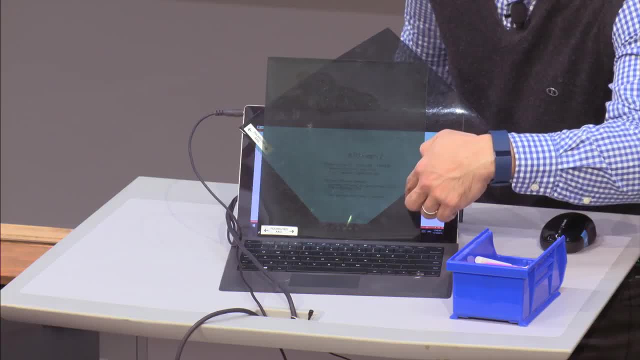 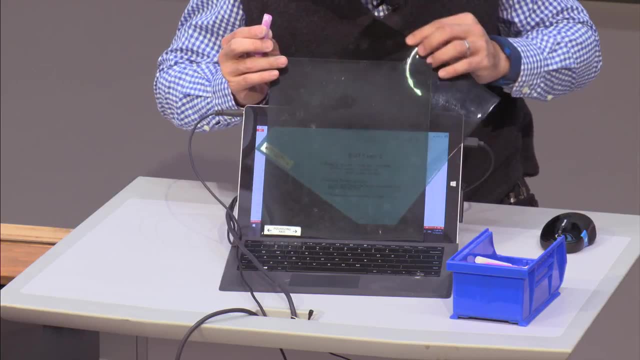 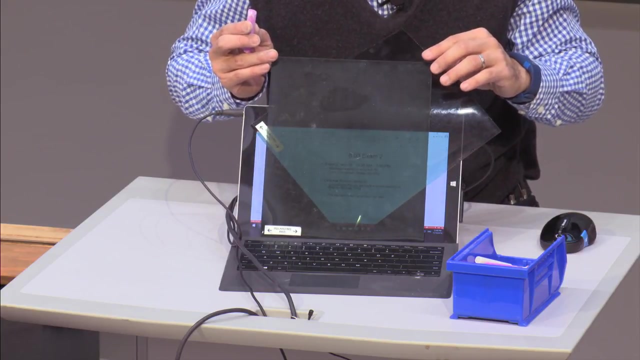 So you cannot see any component which pass through this polarizer. So that's actually pretty interesting And I can actually rotate this and you can see that the magnitude is changing right. Only when I have 45 degree I see a maximum intensity. 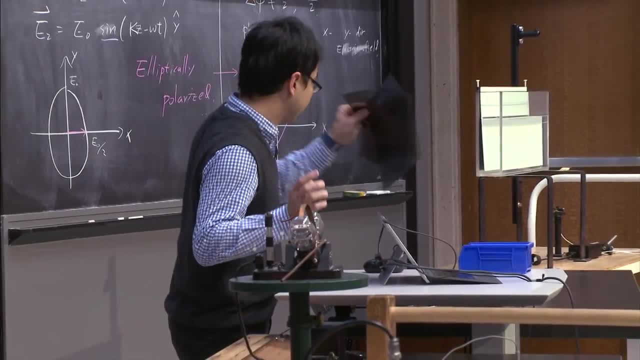 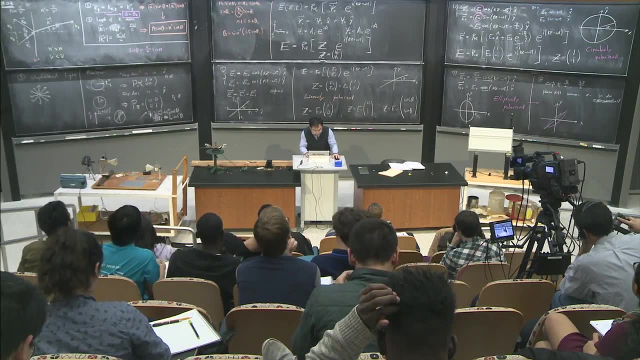 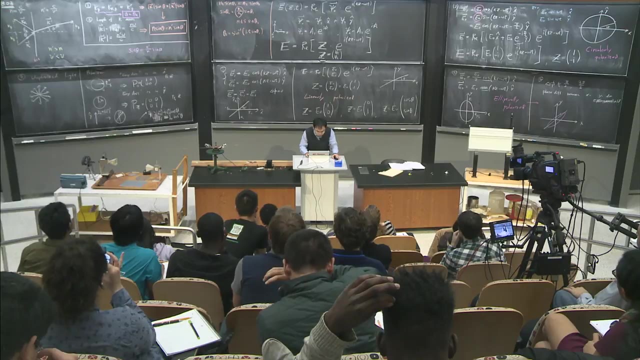 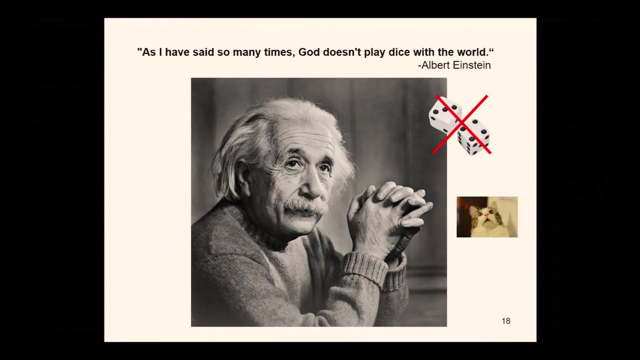 Any questions? OK, Very good. So now what I'm going to do is to discuss with you an interesting question which was posted by Einstein. Einstein said that, as I said, God doesn't play dice with the world Right, So that's actually what he actually believed. 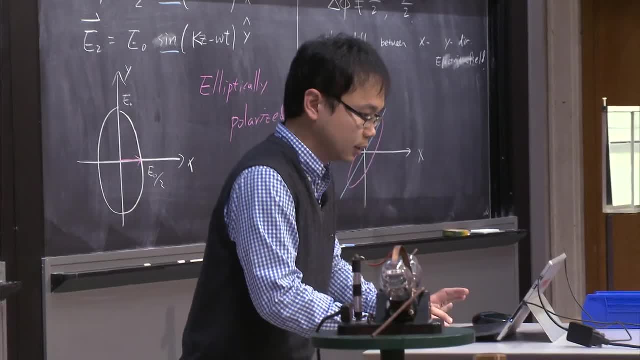 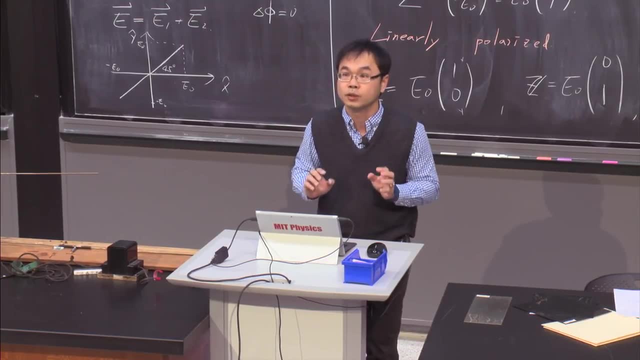 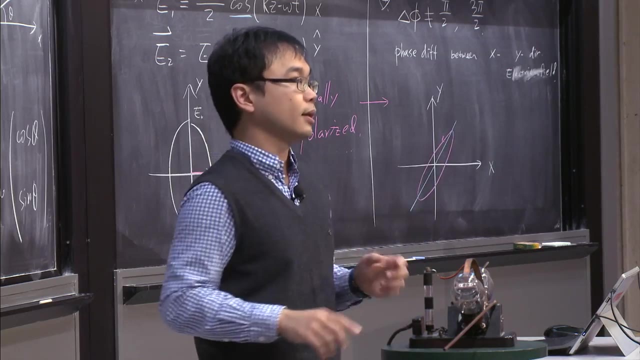 OK, So we can actually do an interesting experiment, which I have: single photon source- OK, So what do I mean by single photon source? I can emit one photon at a time, just one, then the second one and the third one. 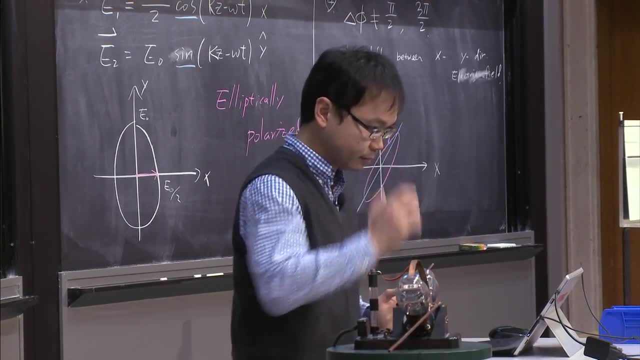 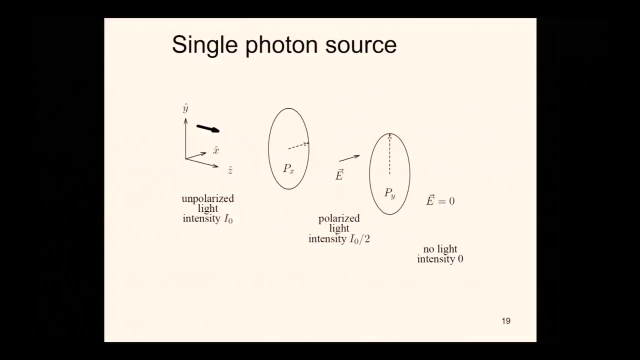 and have them pass through some imaginary polarizer. OK, So let's suppose I have unpolarized light at T i 0.. OK, So, basically, after it passes through this polarizer with any axis pointing to the x direction, in this case. 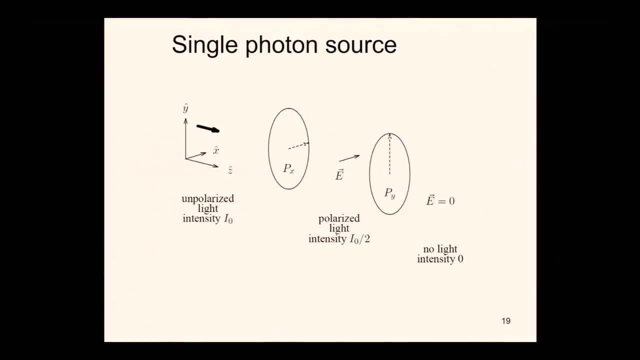 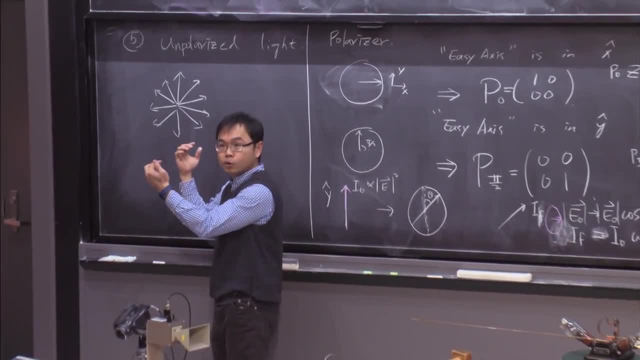 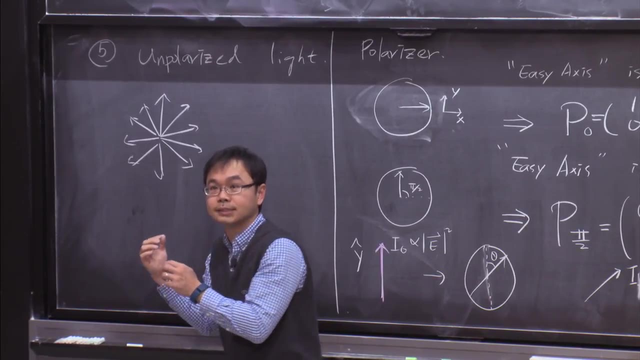 the x direction is pointing to this direction. OK, What you are going to get is that you are going to filter- OK- according from all those unpolarized directions. OK, you are going to filter only the light which is actually parallel to the easy axis, right? 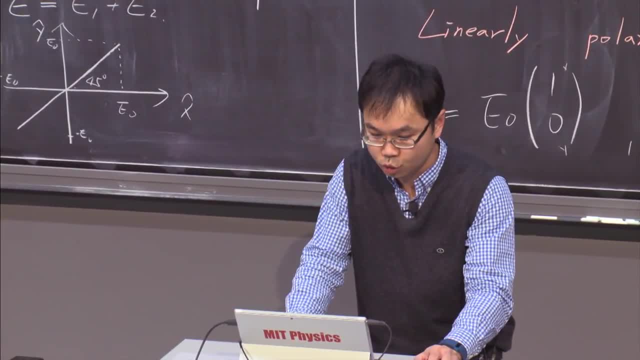 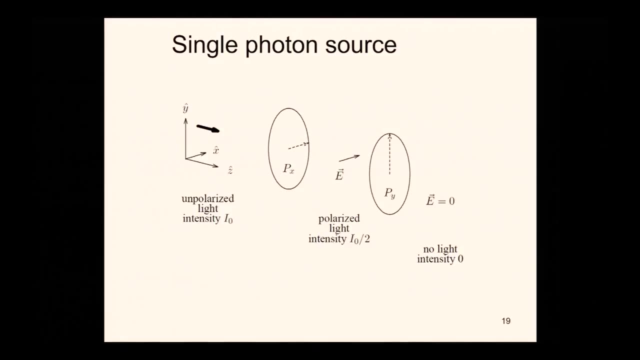 So therefore, after the unpolarized light source pass through this polarizer, you are going to have all the electric field pointing to the x direction. OK, Not everybody can accept. And then, of course, if I have a second one, which is actually: 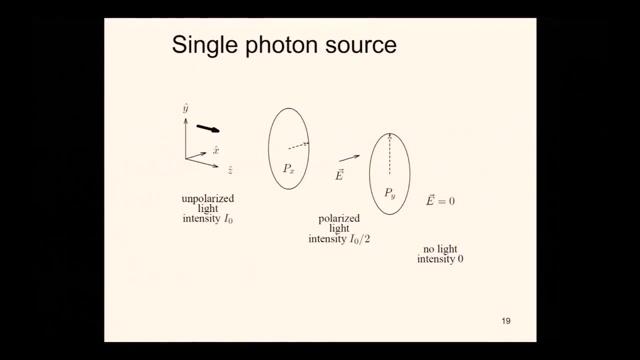 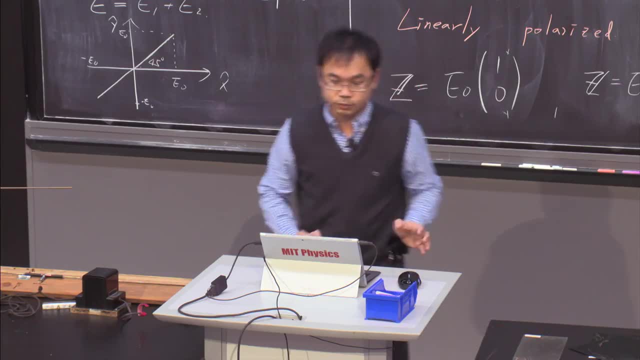 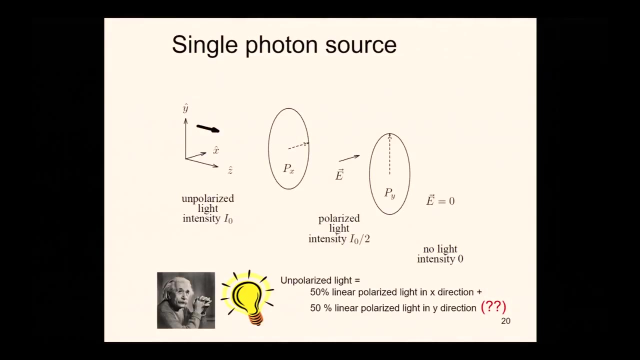 in the y direction. since there will be no component pointing to a y direction, you get zero electric field. OK, So that's very nice. So Einstein was really happy. So that means unpolarized light, maybe it's just 50%. 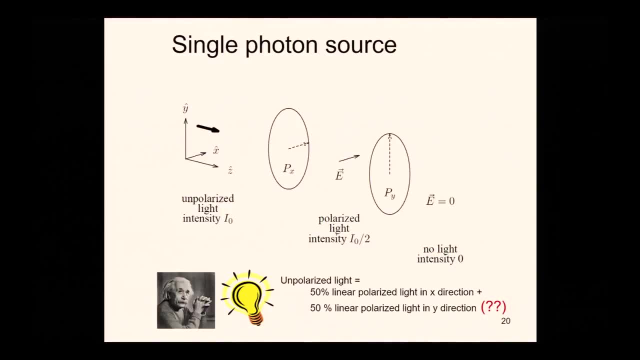 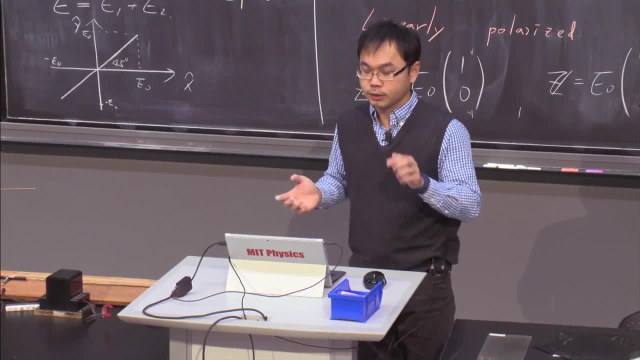 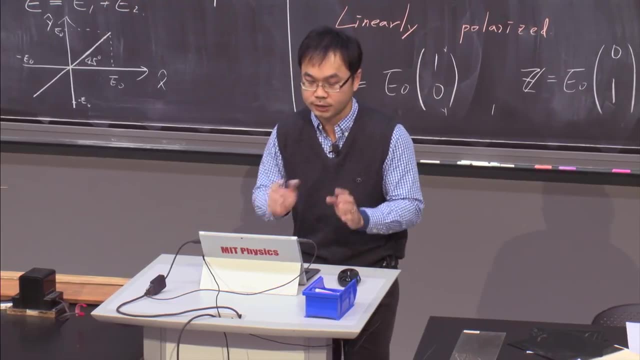 of the polarizer light in the x direction and the 50% of the polarizer light in the y direction. right, Because each time I emit one photon and the first half of that energy got stopped by the x direction. got stopped by the x direction. 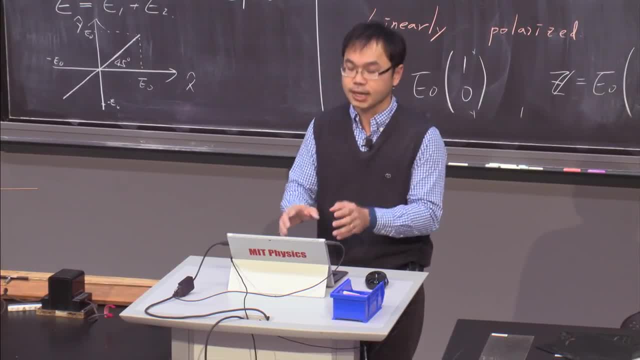 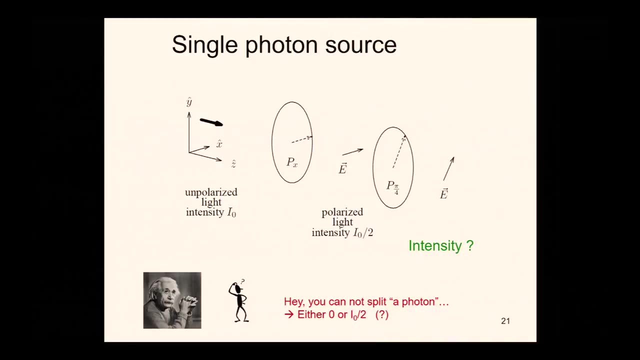 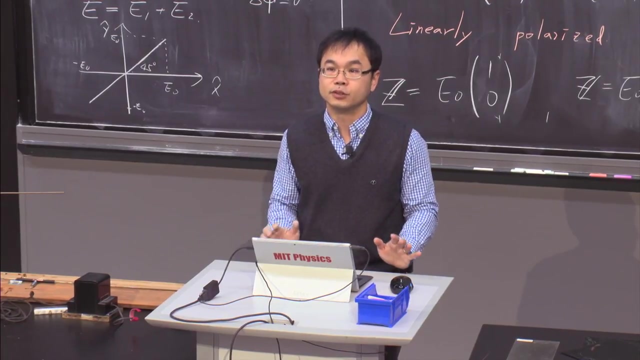 easy axis polarizer, And then the second half got stopped by the second polarizer, right. So that probably makes sense, right? But how about, as we actually did in the demonstration, how about we rotate the second polarizer by 45 degrees? 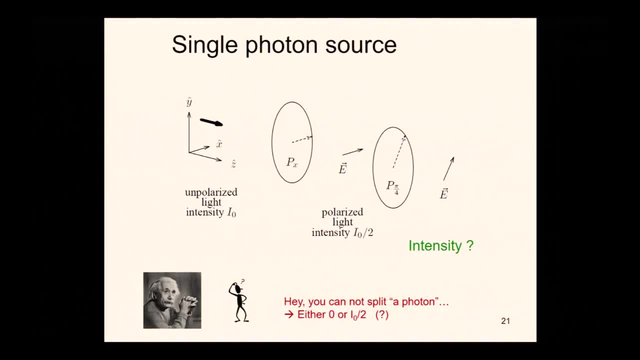 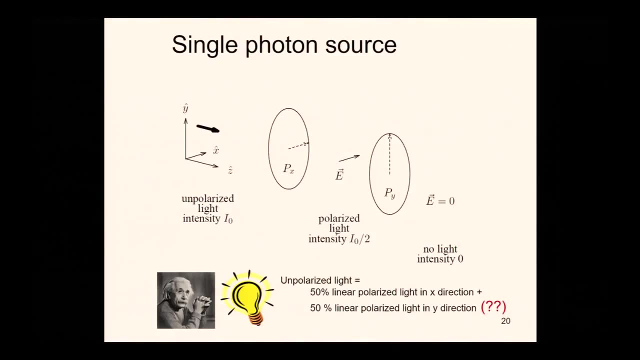 What would be the intensity? right, But now, hey, you cannot split a single photon, right? Because a photon is a photon. Because, if I describe my unpolarized light as 50% linearly polarizing, x linearly polarizing. 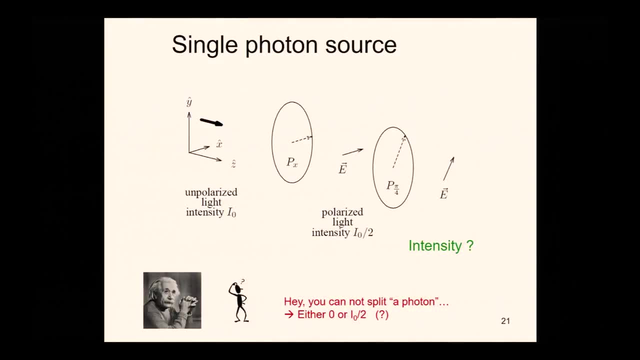 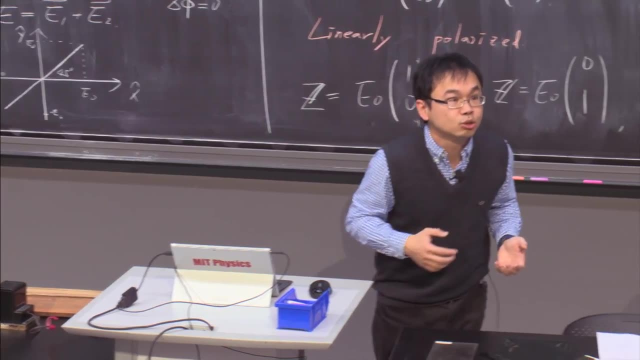 the other half is linearly polarizing y, then I am in trouble because I don't know how to actually calculate what is actually this intensity. So basically, maybe all of them actually pass through or all of them doesn't pass through, right? 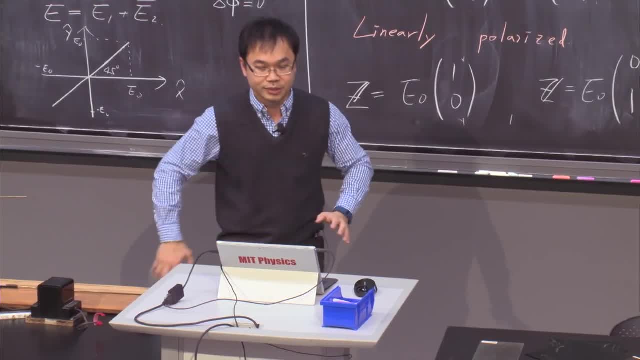 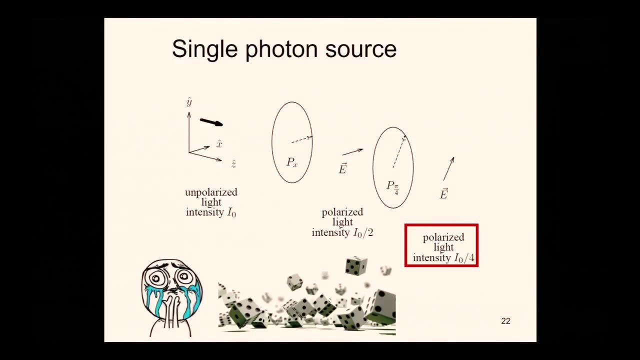 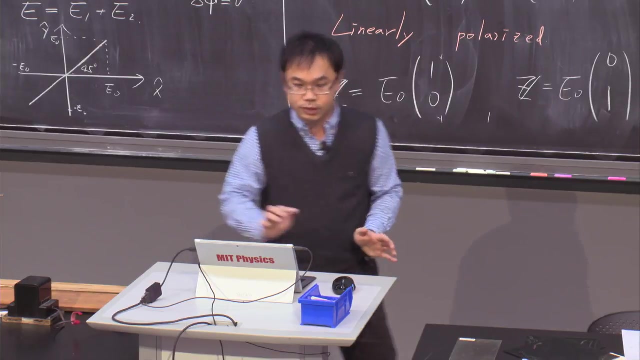 Then actually we can do this experiment And this is the result. What you are going to get is that the intensity is going to be i0 over 4.. That is actually not 0 or i over 2, right, So that means really the natural prey dies. 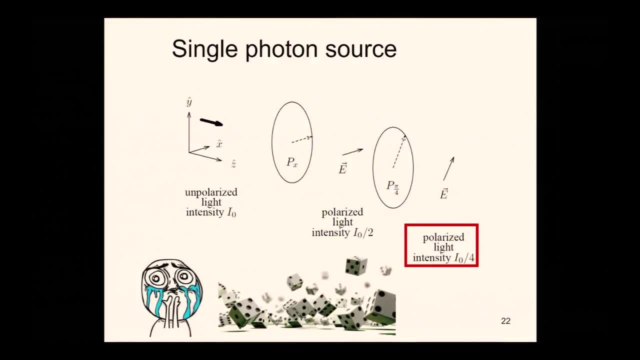 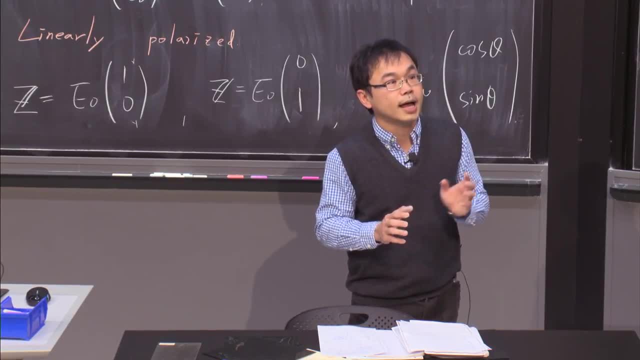 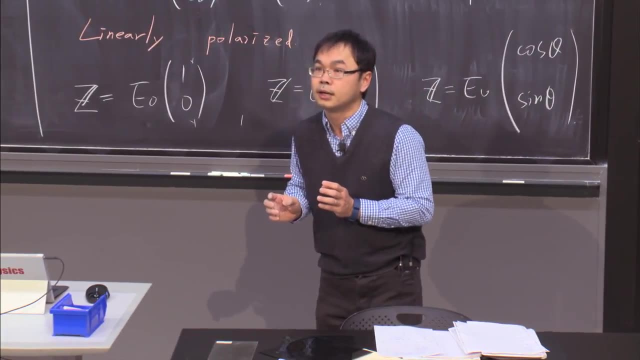 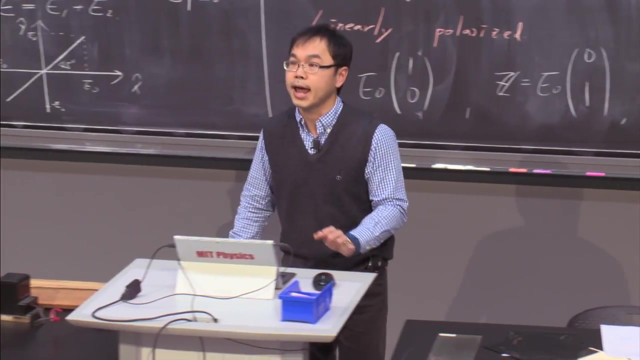 because a single photon actually passes through something which can be described by wave. So that actually gives us some connection, possible connection to quantum mechanics, Because that means a single photon are not like a single object which is actually passing through all those polarizers. 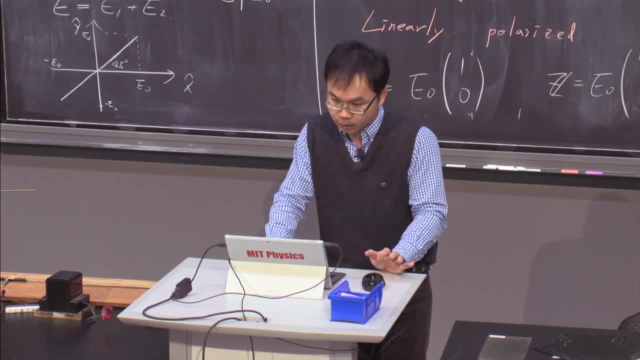 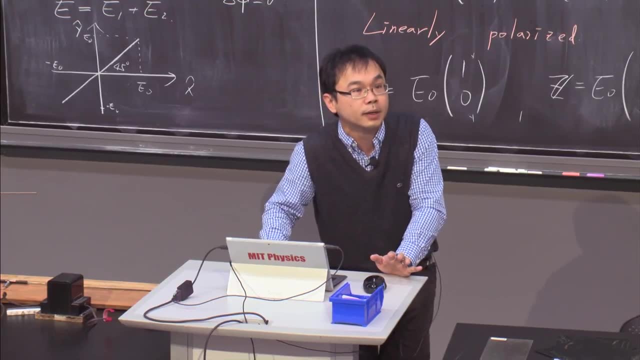 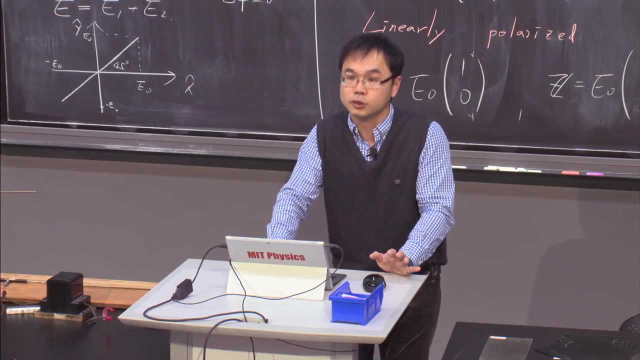 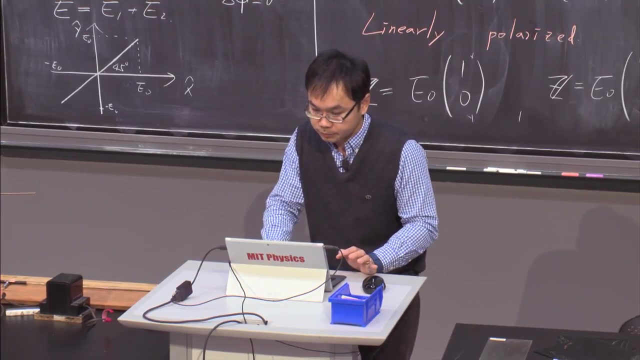 But they actually act also like waves. OK, So that is one thing which we will follow up with later lectures, which, when we talk about interference et cetera, we are going to also discuss related issues about the connection to quantum mechanics. 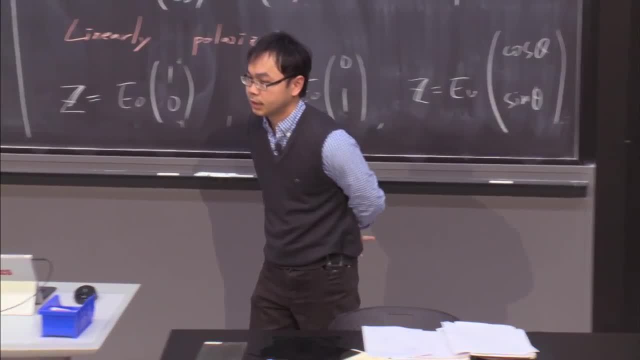 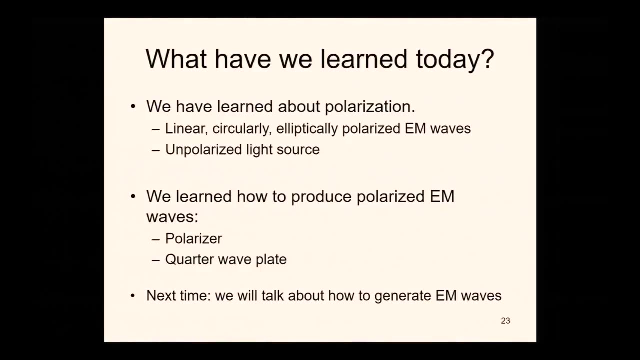 OK, So today we actually have learned about polarization- linearly polarized, circularly polarized and elliptically polarized electromagnetic wave and also unpolarized light source, And we have learned about how to produce polarized electromagnetic wave with polarizer right. 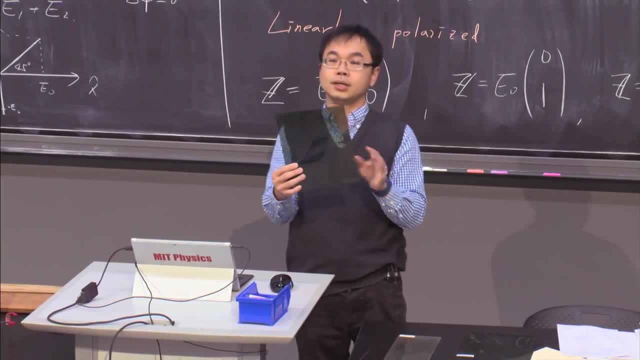 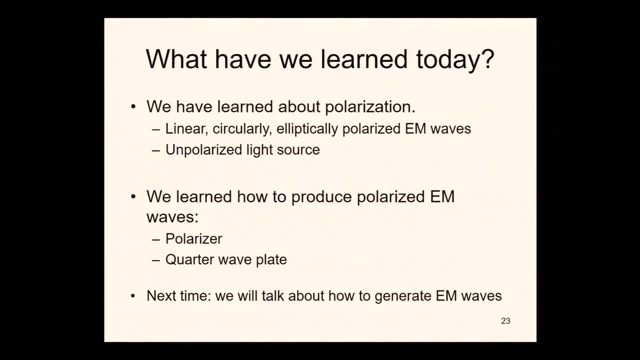 Basically have the unpolarized light source pass through polarizer, You will have a polarized light. We didn't cover a quarter wave plate yet. We are going to cover that next time. And also next time we will talk about how we actually 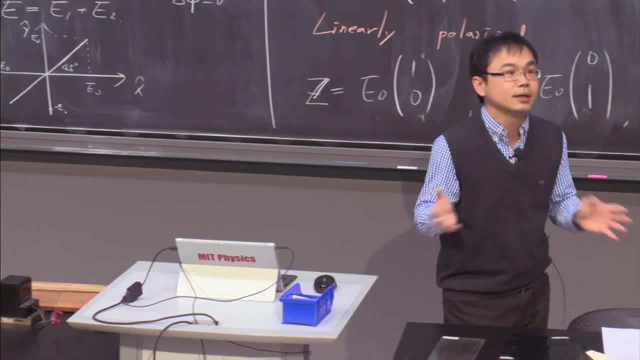 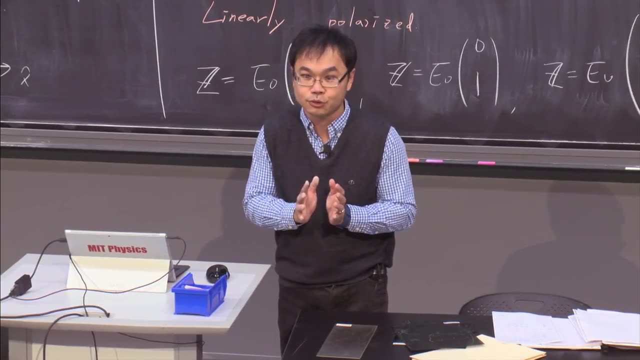 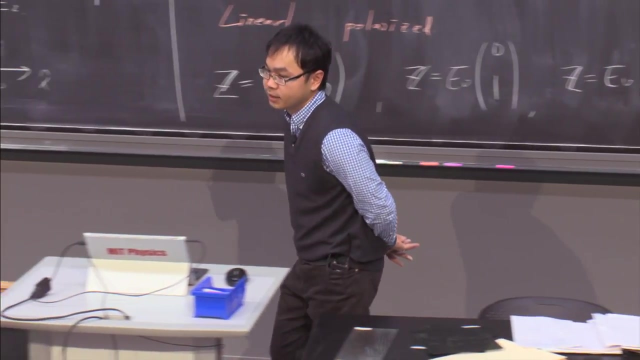 can generate electromagnetic field. the electromagnetic field, We have been talking about electromagnetic field for a long time, But how are they actually generated is an issue which we haven't actually touched, And that is actually going to happen after the midterm next week. Thank you very much.